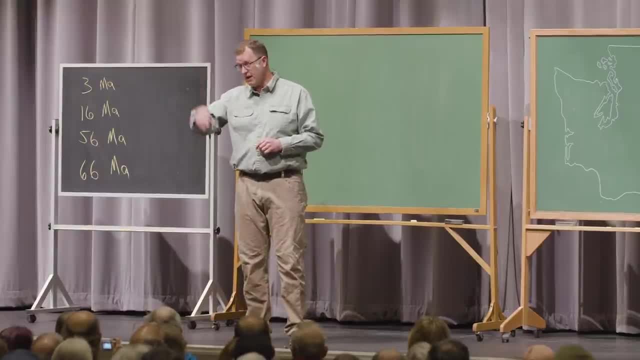 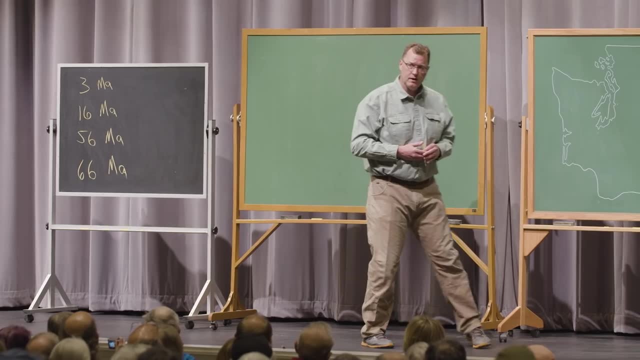 and we could find plant fossils, probably before it got dark tonight. They're all over the place in the bedrock north of town. You got to know where to go. You got to find the right logging road, the right Forest Service road. You got to find some sandstone and shale. 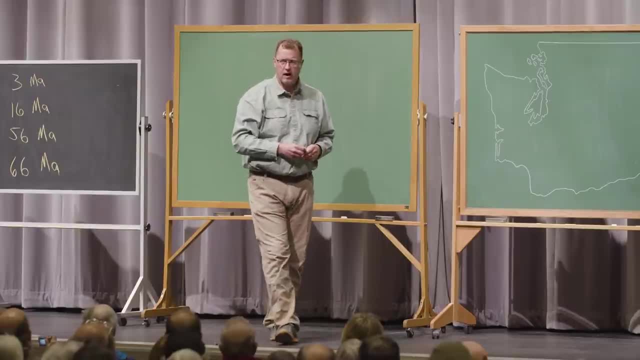 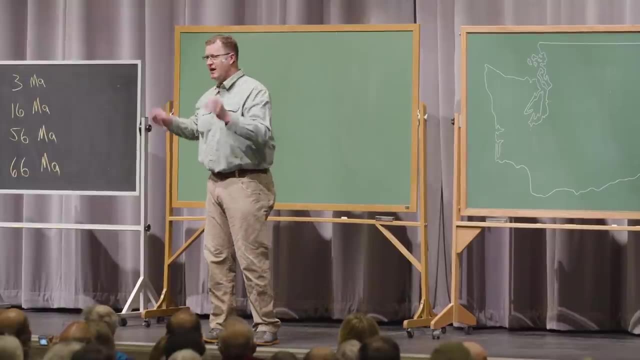 And once we get to the right outcrop, we'd throw the truck into park, We'd get the five gallon buckets out of the back of the vehicle, We'd get the rock hammers and the sledges and the chisels and the screwdrivers and the paintbrushes. 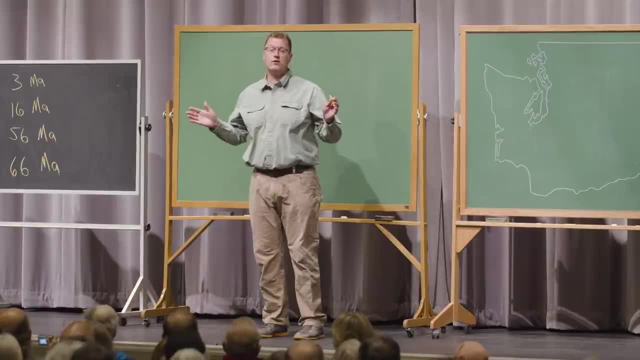 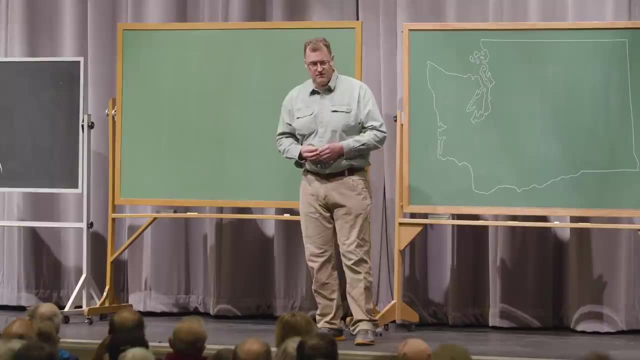 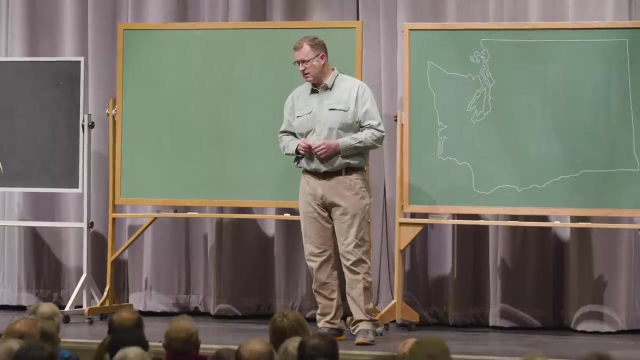 And the you know everything And we'd collect. we'd have a grand old time And we would find hundreds and hundreds of fossilized leaves north of town, Leaves from palm trees, palm leaves the size of dinner plates. There's an unlimited supply of these things. 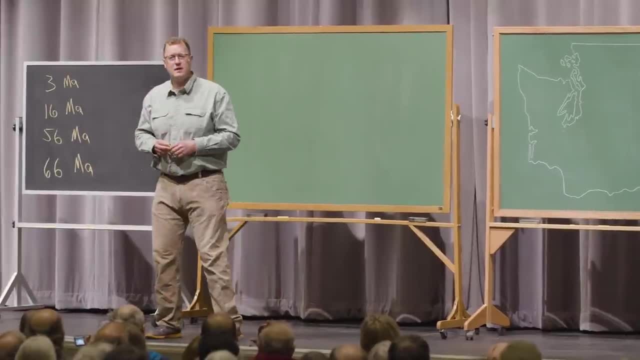 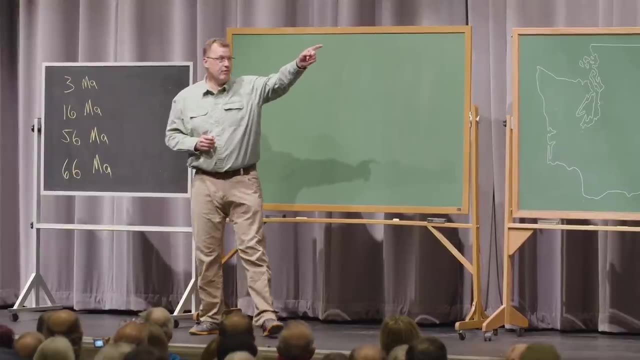 45 minutes north of town. Let's say we had a great time and we did that tonight. And then we come back tomorrow night and we say let's do that again. And then we come back tomorrow night again And we jump in our vehicles and we go the other way. Within 30 minutes we could be in the 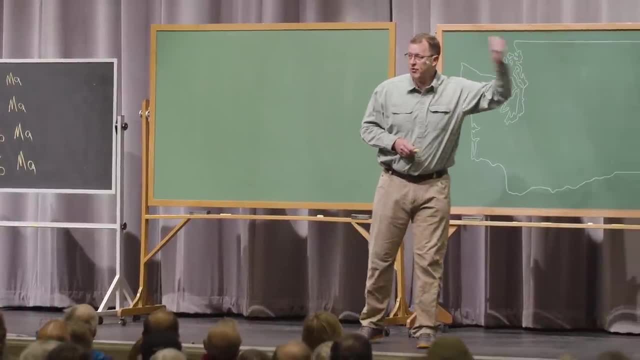 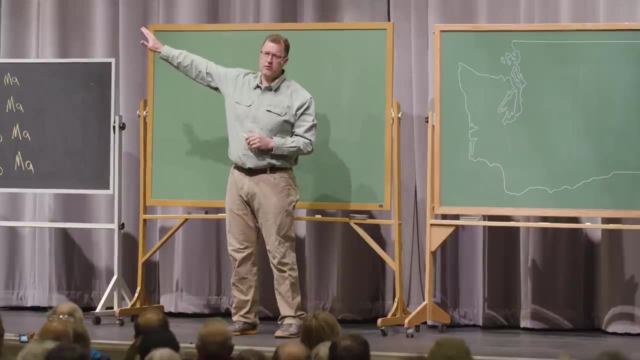 Yakima Canyon, or up Badger Pocket, or 30 miles to the east of here, and go to the town of Vantage, And this time we'd be in the desert. We wouldn't be up in the forest, We'd be out in the desert. 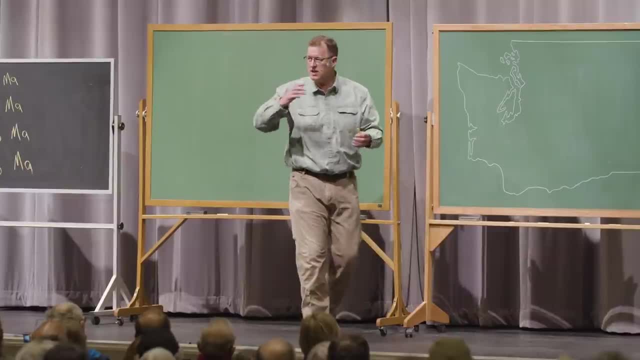 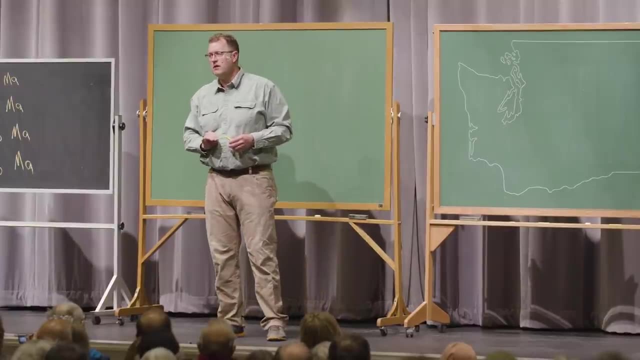 Probably the wind would be howling right. It's green this time of year- There'd be some sagebrush and some cheatgrass, And if we knew which layer to work with- and it's basalt lava rock this time south of town- we would find impressive tree trunks in the basalt lava. 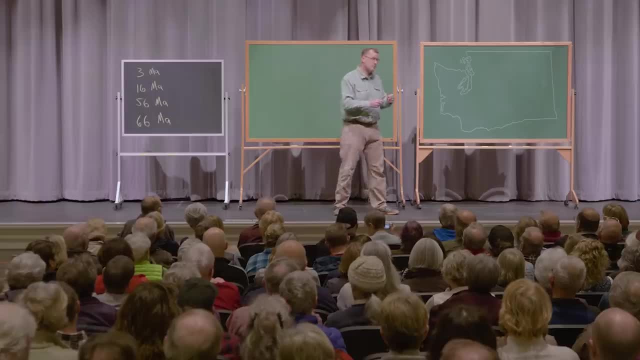 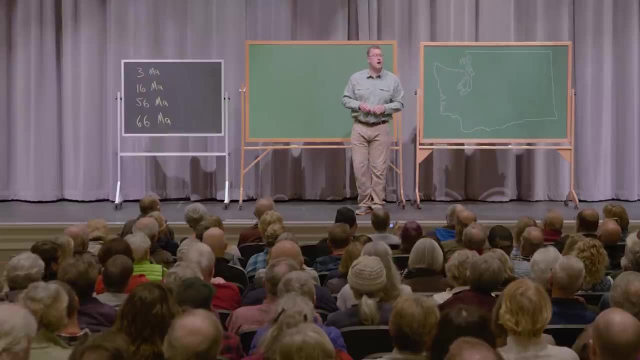 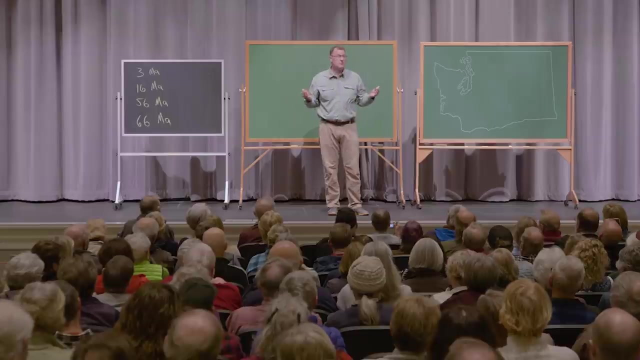 from long ago And the most famous of those fossilized tree trunks that petrified wood are ginkgo trees. So my first question tonight are: are those palm trees north of town and those ginkgo trees south of town from the same forest? Is that the same time that we're talking about? 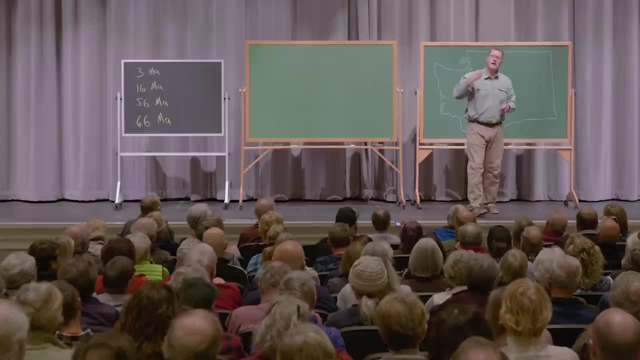 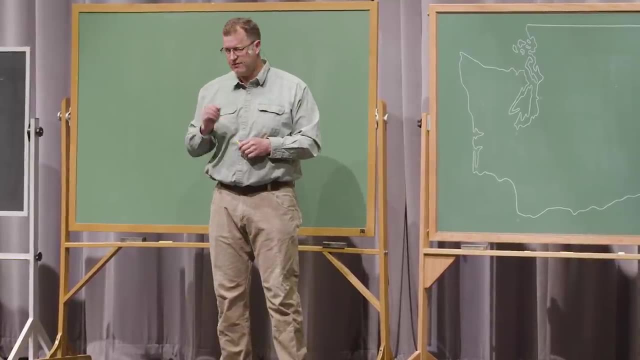 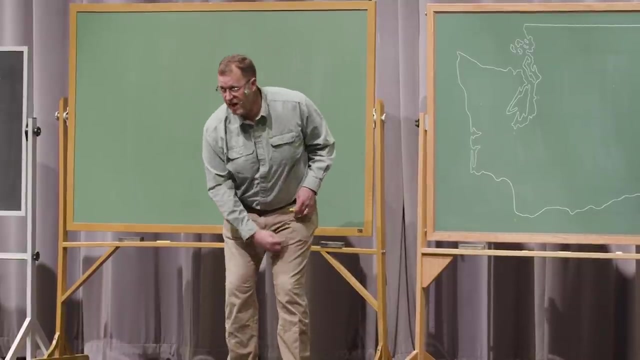 Put that one on hold for just a second. So one of the lectures we did last year in this series, I shared the excitement that we all had because somebody from the Burke Museum in Seattle found the first dinosaur bone ever found in Washington. They found it in San Juan Islands- a fragment of a left thigh bone of a T-Rex First. 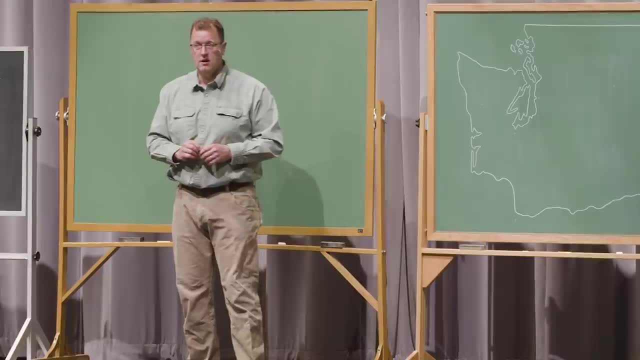 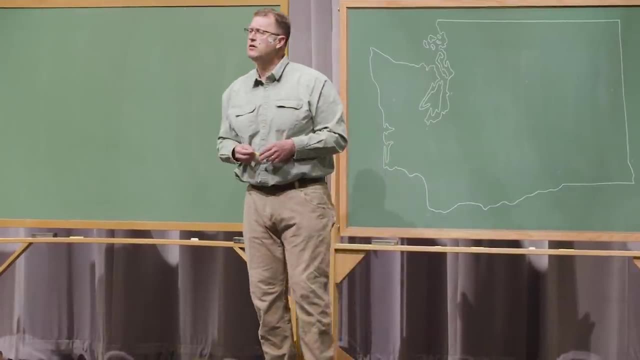 dinosaur bone ever found in Washington. We recorded that lecture, We put it on YouTube and I started getting a bunch of comments last spring And the comments- some of the comments- were like hey, I think you blew it on that dinosaur thing because I live in New York. 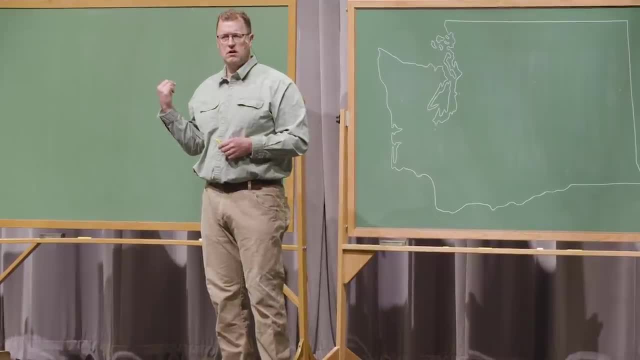 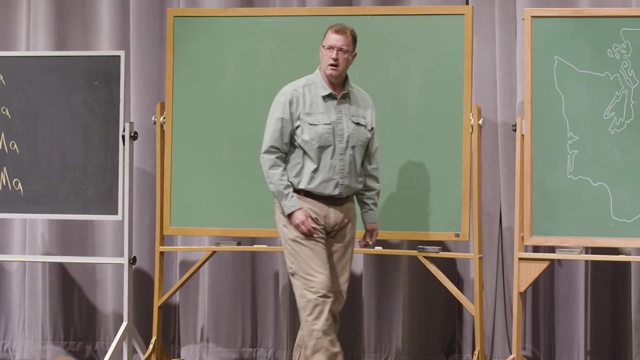 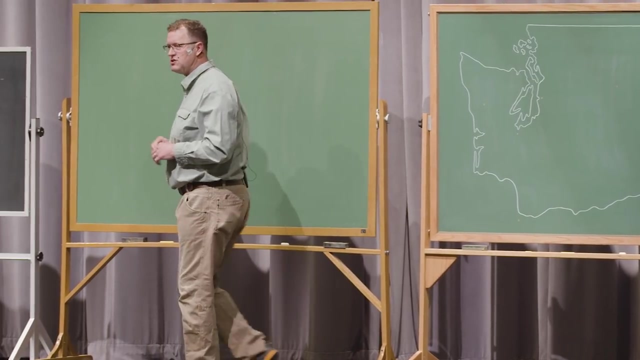 And they dug up a dinosaur like 25 years ago Or I live in Granger. We got statues of dinosaurs all over the place. There's dinosaurs. We got them right here And Moxie and Selah and Tri-Cities in Seattle. They kept talking about all these dinosaurs being pulled out of the ground. So I 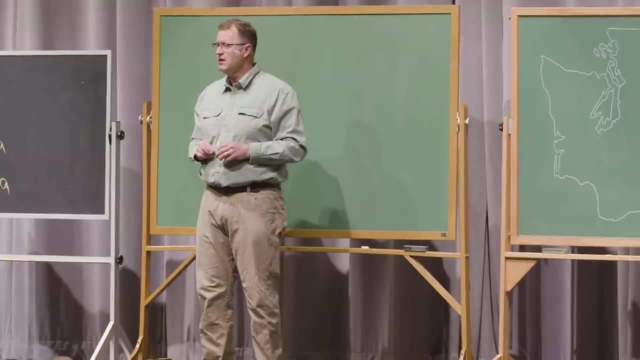 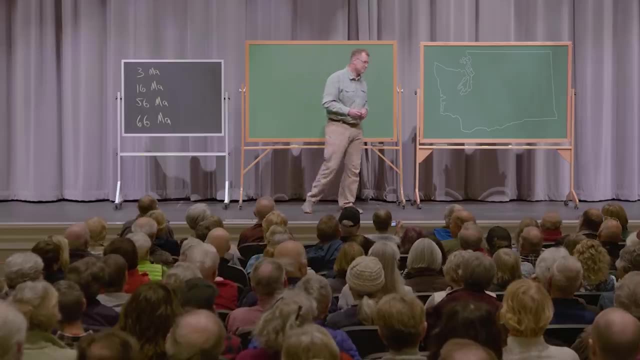 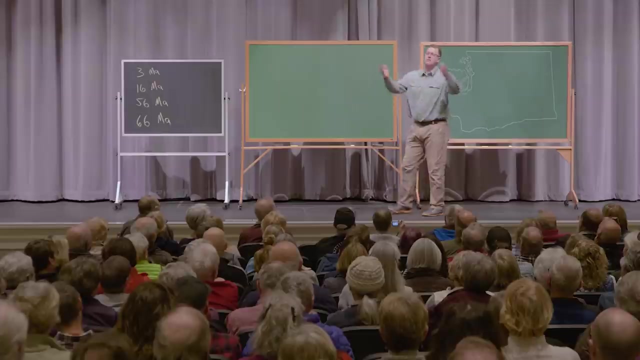 replied to each comment and I said: no, those were mammoths. And they come right back and go. I agree, Those dinosaurs were really mammoth, They were really big. So there's confusion. There's confusion, I think, among many people. If they give it much thought, most of these fossils 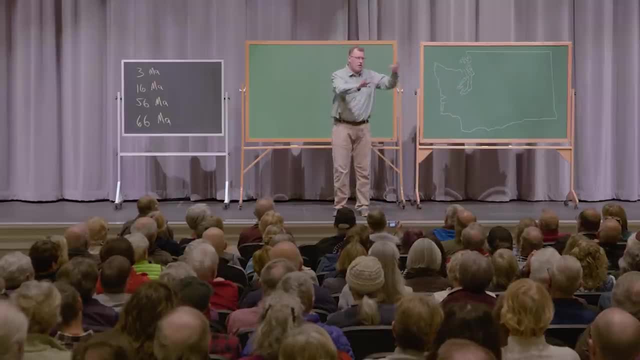 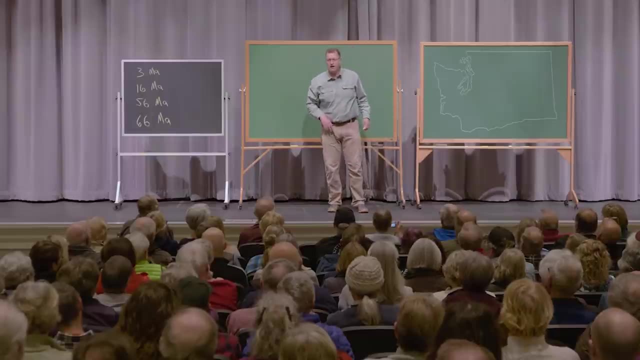 plants and animals are just from prehistoric times And they're all kind of back there together: The palm trees and the ginkgo trees, and the dinosaurs and the woolly mammoths. it's all just back there. Hell, we'll throw in some cavemen for fun, right? It's all just. 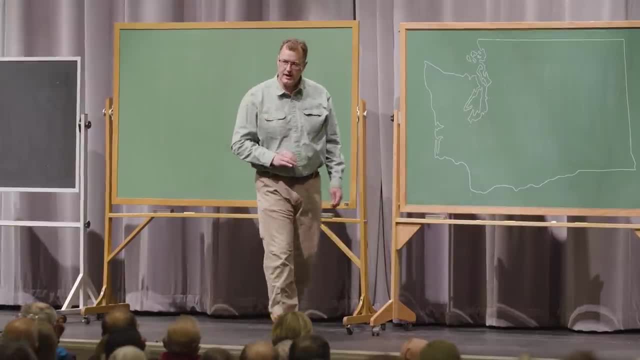 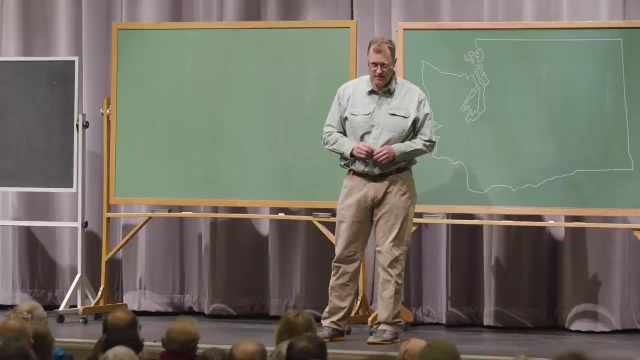 it's just back there. So one of the main things I want to do tonight is make sure that when we talk about specific plant fossils, we know where we are in our geologic history. Each of those plant fossils or animal fossils are talking about a specific environment from the 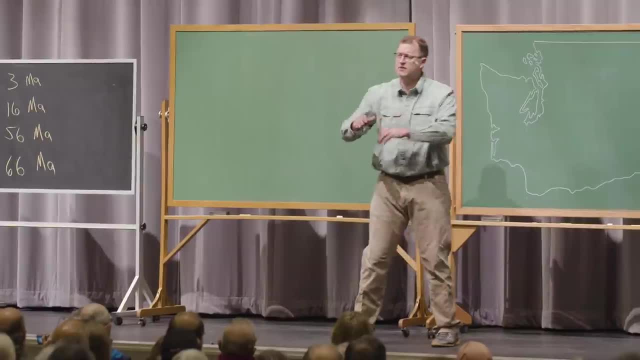 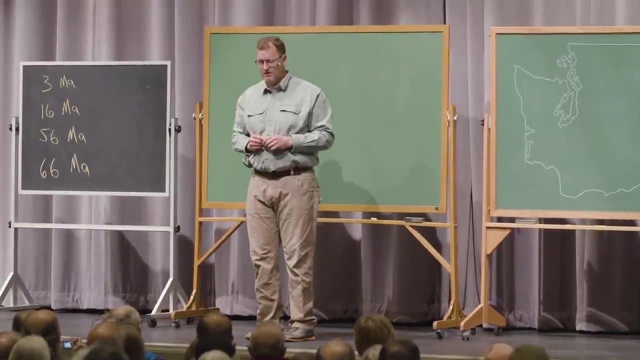 past And plant fossils are famous for being very sensitive to conditions, to climate conditions, And if we change our fossils through time, we change our climate through time. So the plant fossils are important to study, not just because they're cool, not just because we can throw them in the 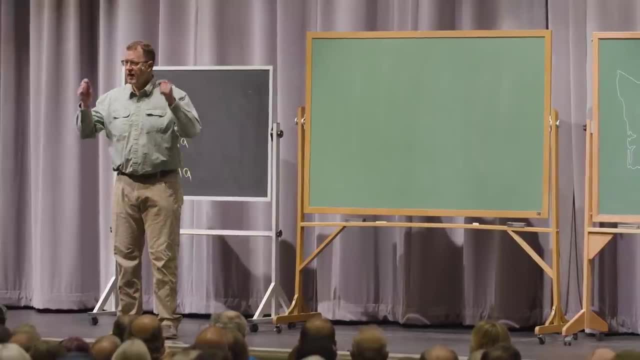 back of our truck and bring them in and put them in the front yard, but they are important for scientific study as well. So we're talking about a specific plant fossil in the history, Each of those. So I've got a quick little timeline up here. 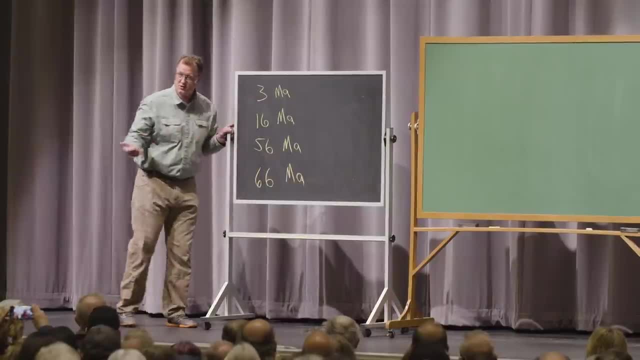 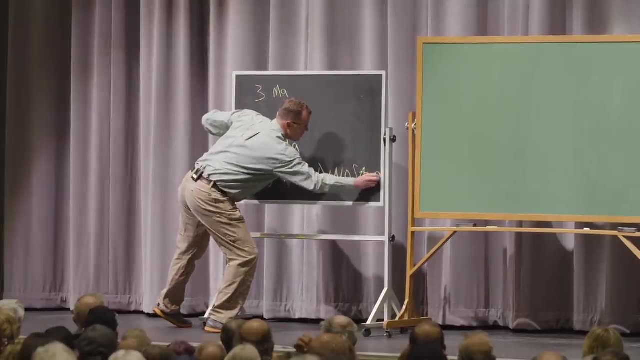 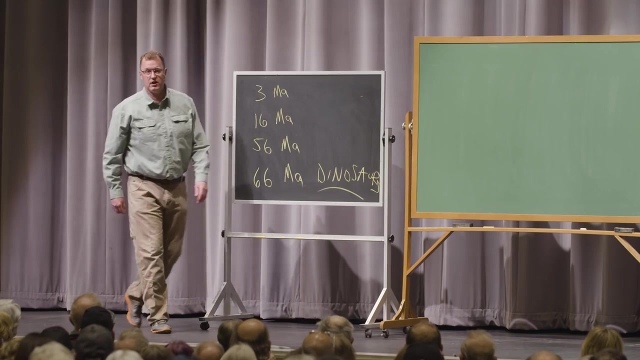 I'm going to do this very quickly. These are in millions of years. This is a science lecture. 66 million years ago, most of us know that the dinosaurs of the world, the dinosaurs of the world, became extinct. There are no dinosaur bones worldwide in rocks that are younger than 66 million years ago. Not one dinosaur bone is younger than 66. So this is the famous extinction of the dinosaurs, And below that we've got lots of dinosaurs around the world. That dinosaur bone on Sushia Island in the San Juans came out of some siltstone 80 million years old. 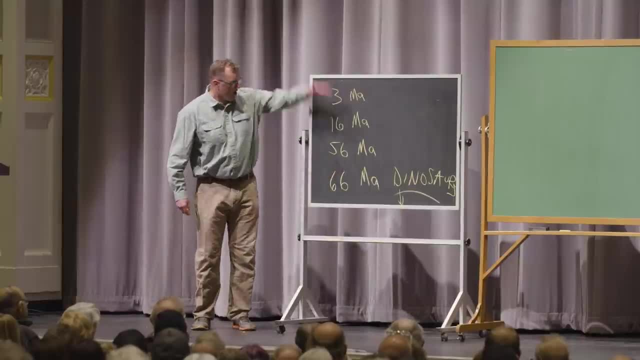 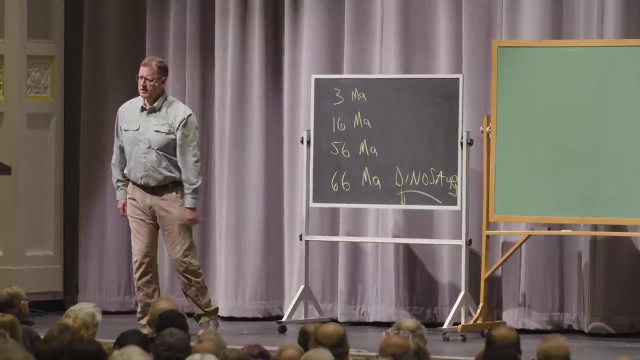 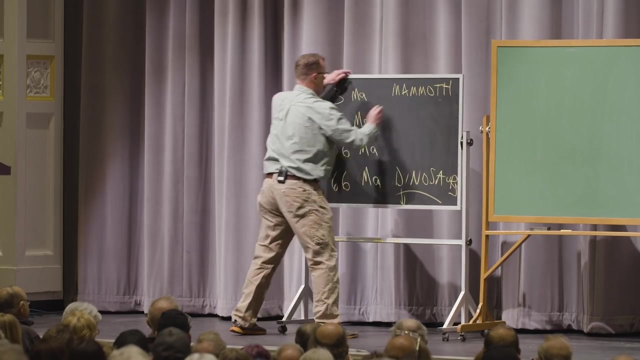 Our plant fossils tonight here in the Pacific Northwest are all younger than the dinosaur time. Great Now the mammoths. dinosaurs, mammoths. is there really a difference? Of course there is. The mammoths are an ice age creature. the woolly mammoths. And I can just pick the number three For simplicity. but during the ice age, the last 2.6 million years, we had these woolly mammoths dominating much of the world, including central Washington here. So I don't care really personally about the anatomical differences between dinosaurs and mammoths. 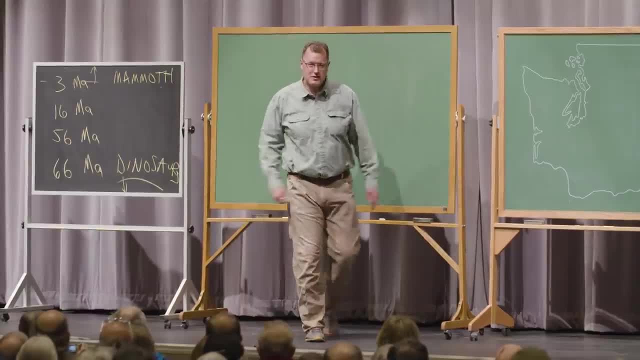 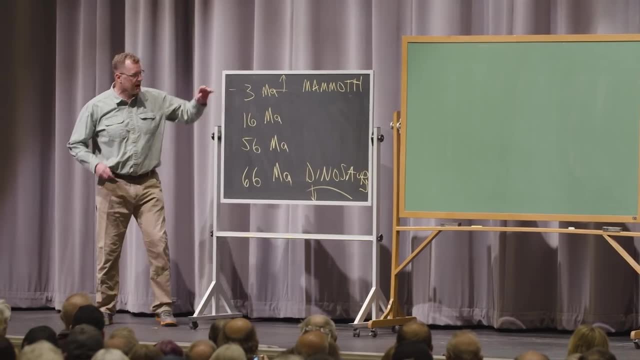 I'm interested in the fact that they represent a difference of more than 60 million years worth of time. That's where I'm coming from, But this is not a lecture on plant fossils, excuse me. this is not a lecture on animal fossils. 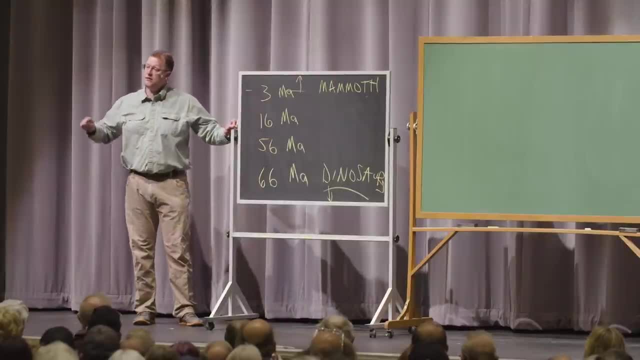 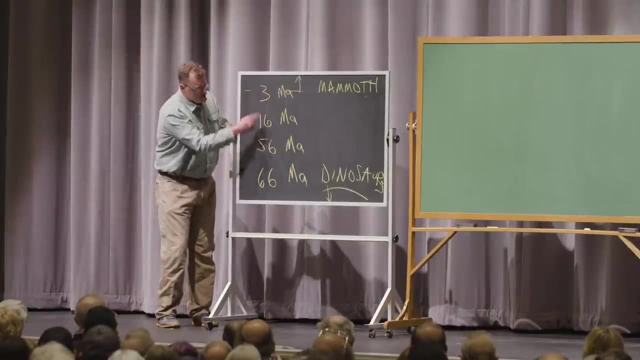 It's a lecture on plants And there are lots of different plant fossils. I've got tons of visuals for you tonight, tons of video clips and beautiful pictures, And we're between these two times older- excuse me, younger than the dinosaurs, older than the mammoths. 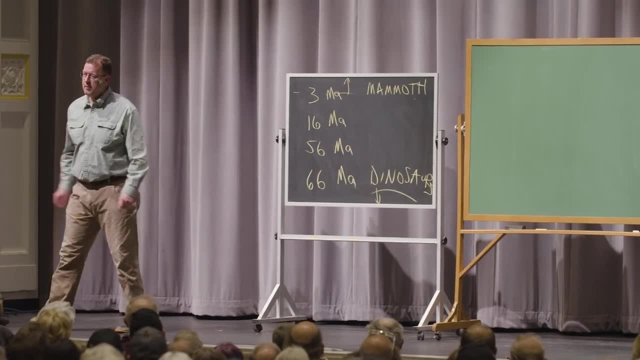 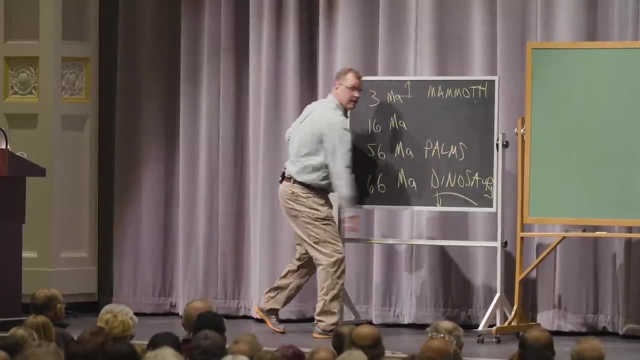 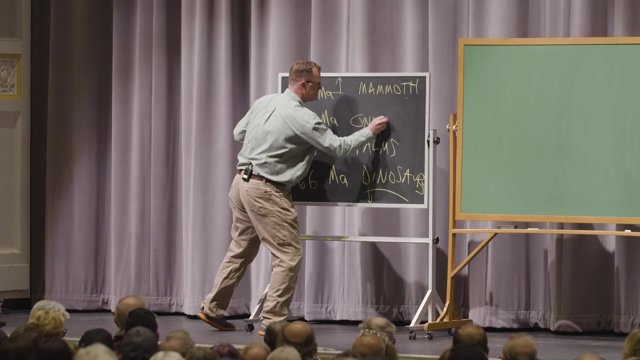 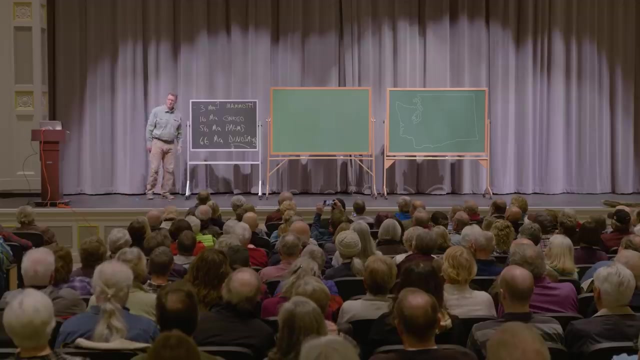 But I want to zero in on two key dates: A bunch of plant fossils from 56 million years ago and those are our palms up at Blewett Pass And the Ginkgo trees out by Vantage Yakima Canyon, Badger Pocket. those are roughly 16 million years ago. 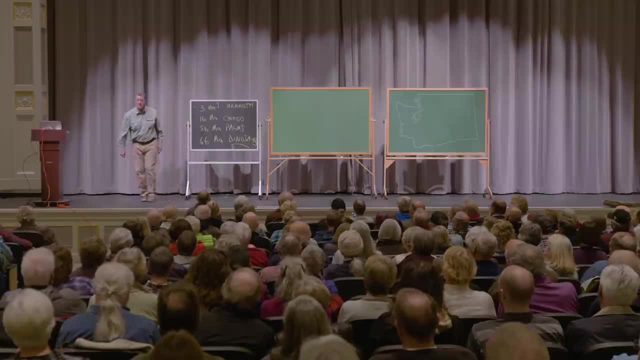 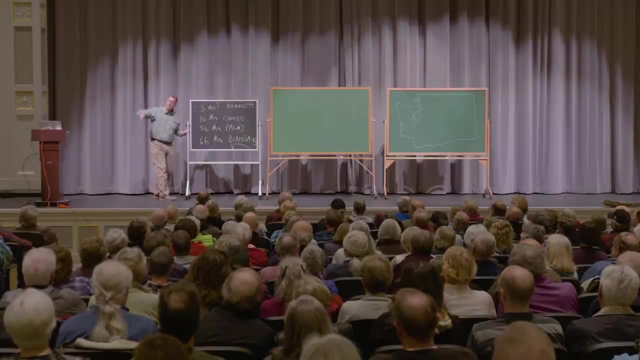 So they're not the same forest, they're separated by 40 million years. So we're going to do some things with these two timeframes primarily, and then we'll dabble in a few other spots. It's down in Oregon, Northern Idaho et cetera, between these two things. Okay, Let's keep it moving, Because I want to make sure we get to all the timeframes. Okay, Let's keep it moving, Because I want to make sure we get to all the timeframes. Okay, Let's keep it moving, Because I want to make sure we get to all the timeframes. 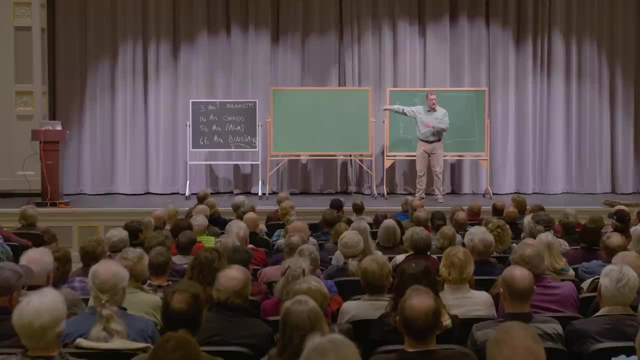 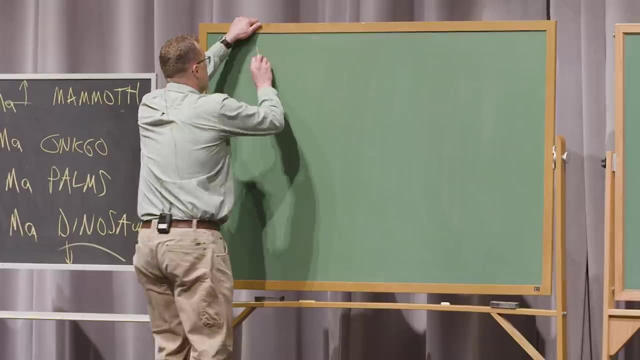 Because I want to make sure we get to all these wonderful visuals. So I'm going to leave that on the blackboard. I'm not going to change it. That's our little reminder of our times that we're talking about. So why palm trees? 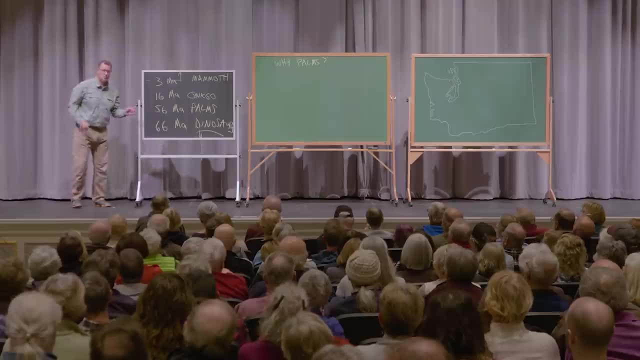 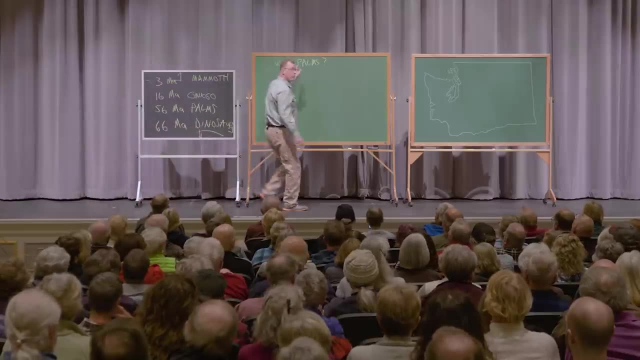 Why palm trees 56 million years ago? And, to be fair, the Swak Formation has a range of ages, but a bunch of the palm fawns are coming from 56 million years ago. Well, we know that palm fronds and palm trees like hot and humid conditions. 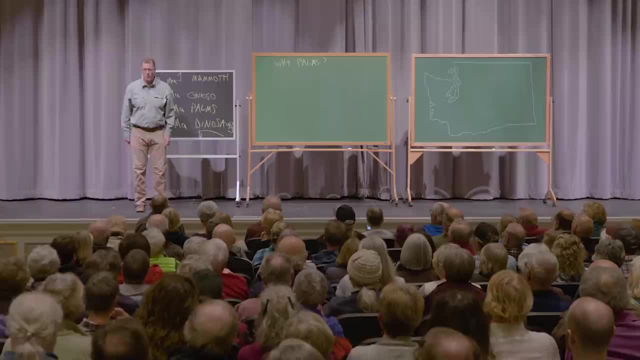 Well, we know that palm fronds and palm trees like hot and humid conditions. We're from Central Washington. If we go on a spring break trip, we're going to take a bunch of pictures of palm trees to prove we're in a warm, beautiful place. 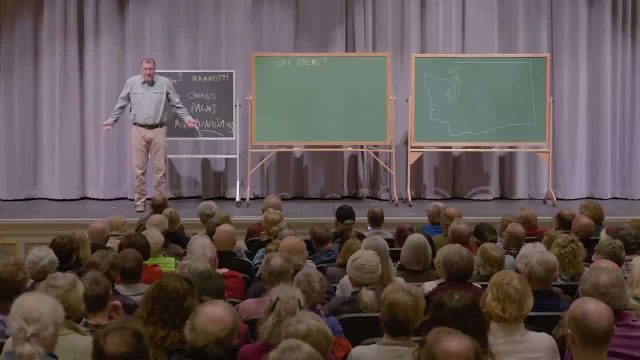 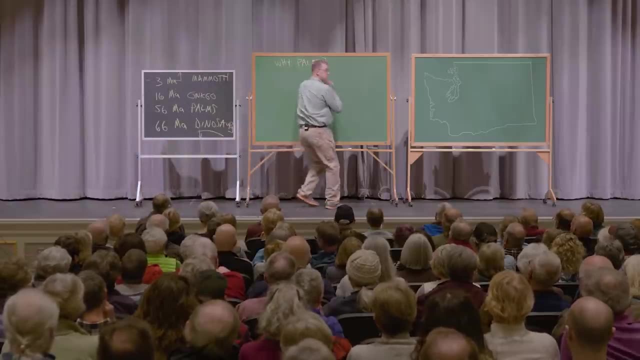 Like we made a good choice. Look at this: There's a palm tree Right, They're not here. I know Yakima is the Palm Springs of Washington, but there's no palm trees down there. Okay, So they're subtropical. Palm trees, palm meadows. they love subtropical conditions. Let's make it as simple as possible. And for our purposes tonight, let's just say: And for our purposes tonight, let's just say: But we need hot and humid conditions. We need temperature hotter than current day in Central Washington And we sure as hell need a bunch more precipitation if we want to grow palm trees here north of Ellensburg. Well, I want to bust a couple of myths. I've been out with a lot of people through the years and I keep hearing these two stories. 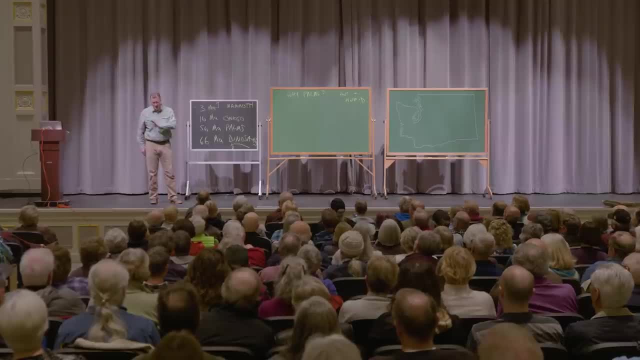 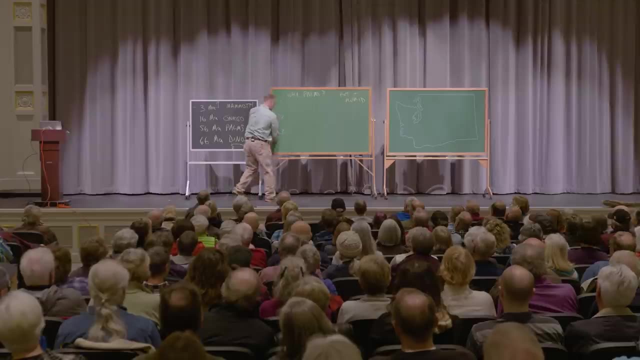 Kind of these folks that have all the answers you know, And both of these stories are wrong. There's a third one that actually is accurate and what we want to hit hard tonight. So one, two, three. Why was it hot and humid here 56 million years ago for these palm leaves and other things? 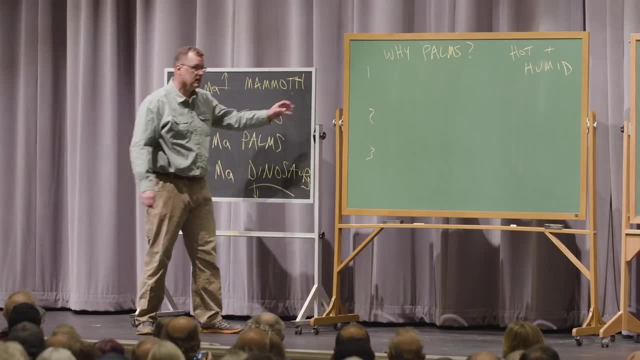 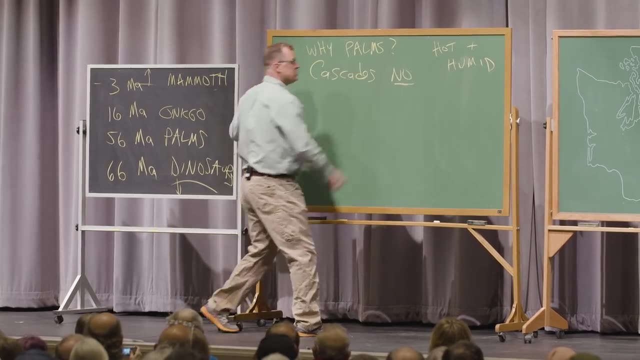 There were big swamps, Swamps recorded in these bedrock layers north of town. One talks about the Cascades And, in fact, mentioning that there was no Cascades at the time. And so far, so good. We know the Cascade Mountains, don't we? 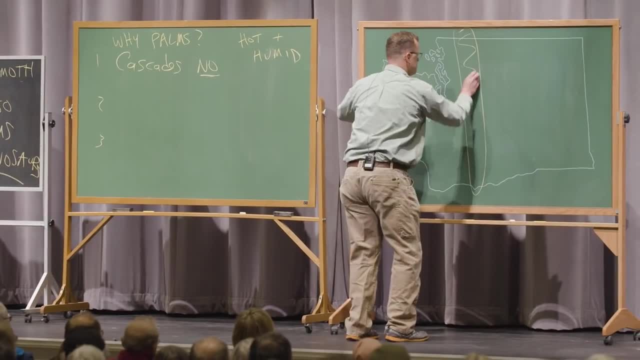 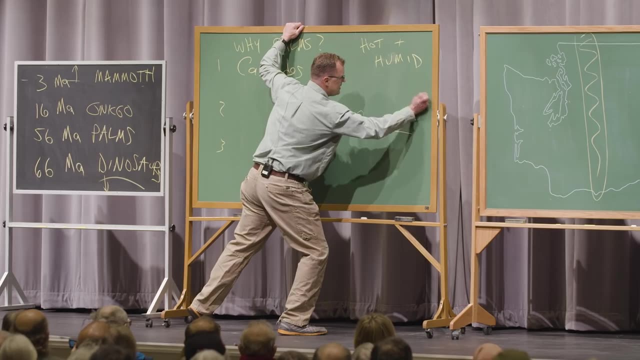 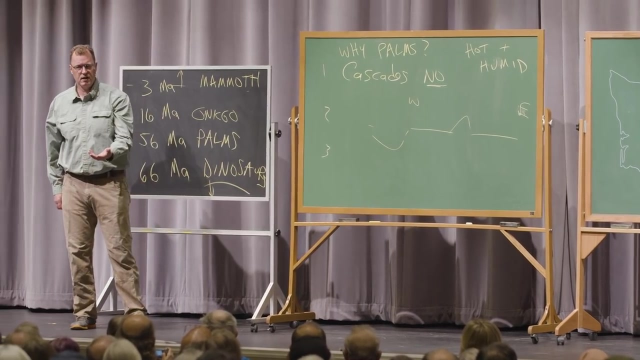 The Cascade volcanoes right here. These are the Cascades, And if I draw a picture Here in side view, of the Cascades, where this is east and this is west and here's the Pacific Ocean offshore, We know about the rain shadow effect, don't we? 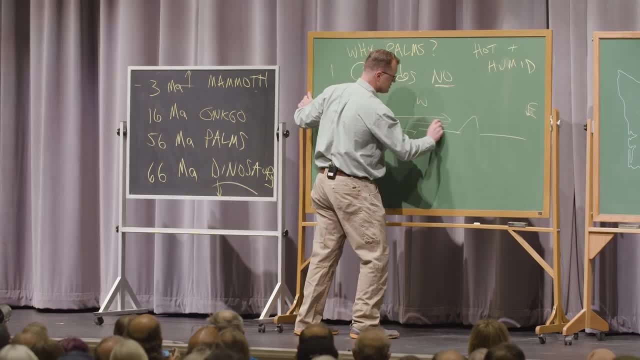 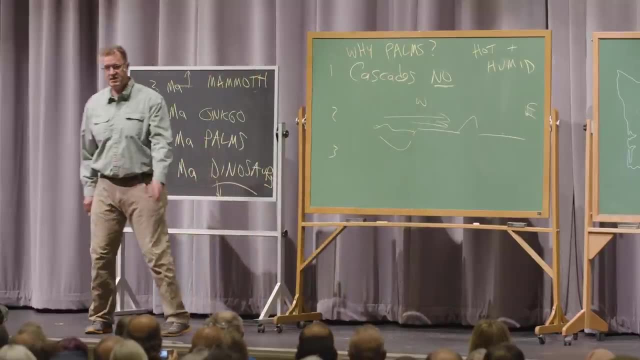 And the idea is that we get a bunch of moisture in off the Pacific Ocean. Seattle gets a lot of rain And over here in Ellensburg, at the Morgan Auditorium, we don't get nearly as much rain. We get less than 10 inches of rain a year here in Ellensburg. That's because of the rain shadow effect, the fact that these air masses with moisture in them have to get up and over this barrier, the Cascades, and by the time those winds are over here, they've lost most of their moisture. So the idea is: oh, we got palm leaves in central Washington. Well, those palms are from such a long time ago that the Cascade Mountains were not here, And a bunch of moisture could get all the way over to eastern Washington. That's true So far. the Cascades have a 40,, 4-0, a 40-million-year history. The Cascades are younger than these palm fossils, So so far I'm in. We are getting a bunch more moisture, much more precipitation in central Washington. But what's the problem? We need temperature, We need much warmer conditions, We need tropical conditions in Washington. 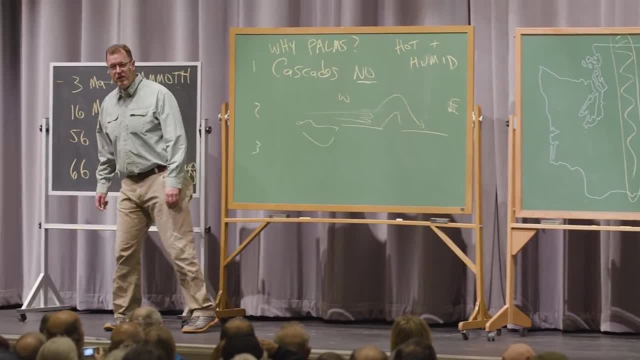 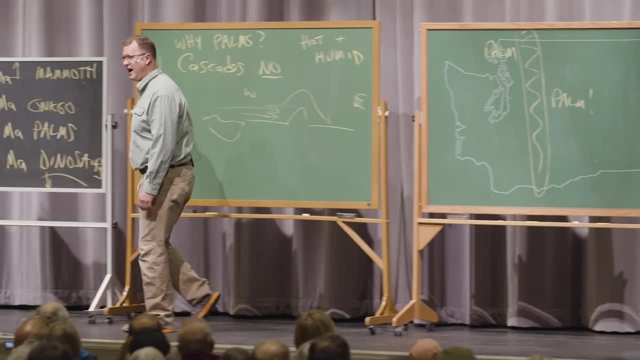 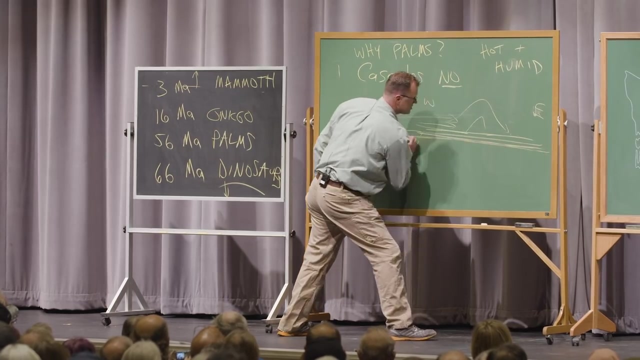 And just not having the Cascades is not going to do that. Plus there are just as many palms, Plus we've got the Cascades. on the other side of the Cascades And in fact those sandstones and shales used to be continuous beds. 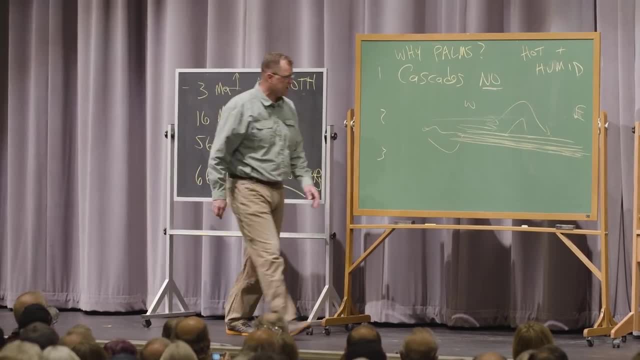 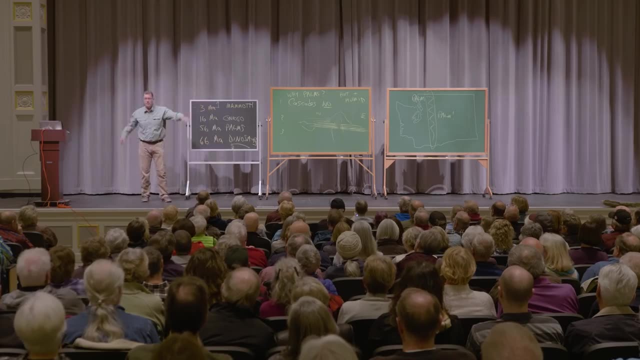 In other words, they're older than the Cascades and they continue across that region And the Cascades have essentially grown up through the middle of those two sedimentary beds. So palm fronds in Bellingham, palm fronds here, same beds predating the Cascades. 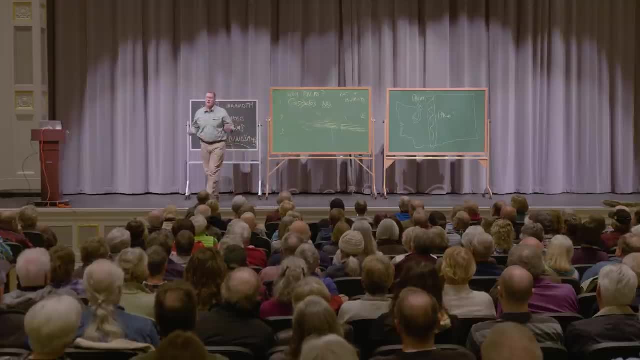 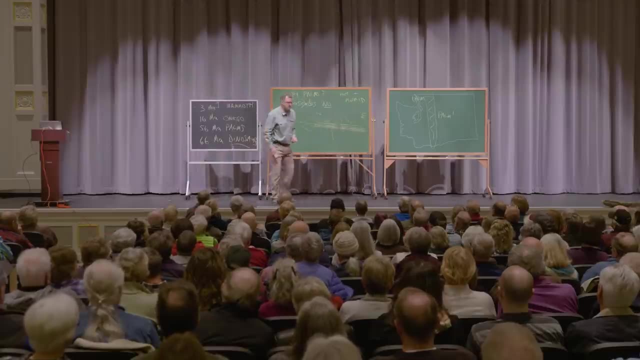 But to say that the Cascades were not here and that's why we had palm trees is not the way to go. Next one: that is wrong. This is mean spirited. I don't mean to peddle it this way, but I guess I am. Have you caught yourself saying this to? 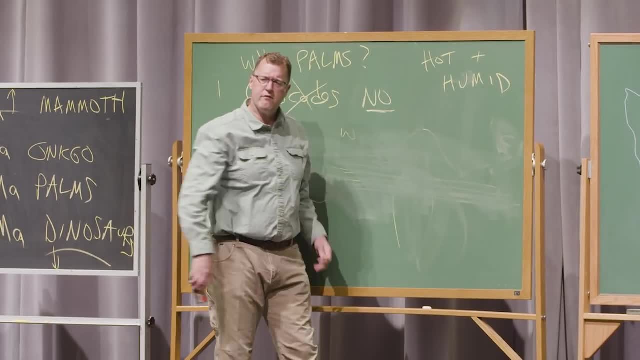 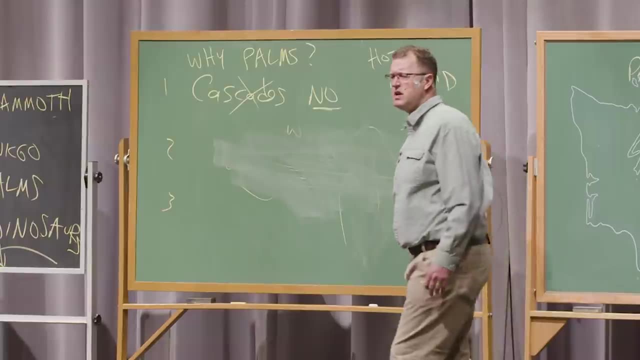 somebody. Oh yeah, we got palm. we got palm fossils around here. Have you ever heard of something called continental drift? You want, you want subtropical, You want, you want it hot and humid here It's real easy. We go back in time and North America used to be at the equator. 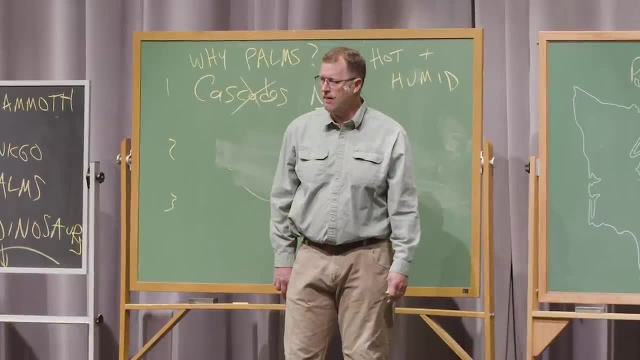 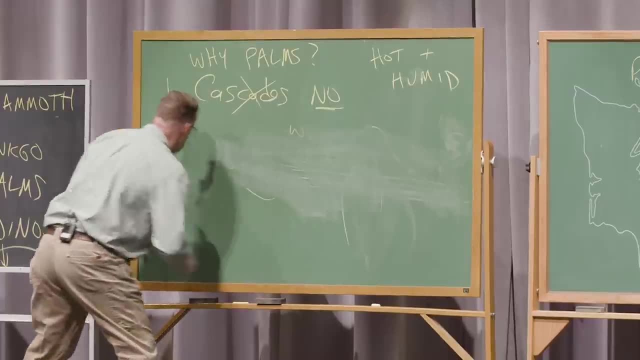 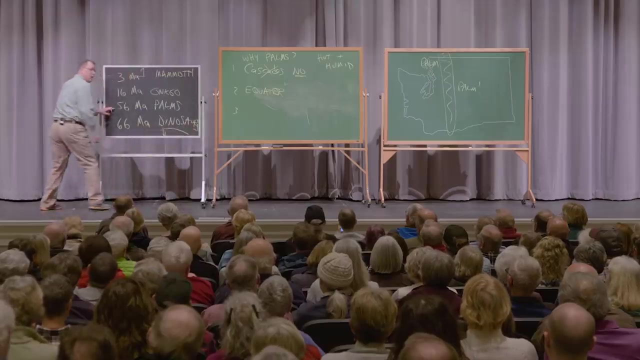 Case closed. That's nice and convenient. It's wrong, but it's nice and convenient. How do we know that's wrong? How do we know that North America, during this time of our, of our palm fronds, was not at the equator? Well, let me show it to you graphically. 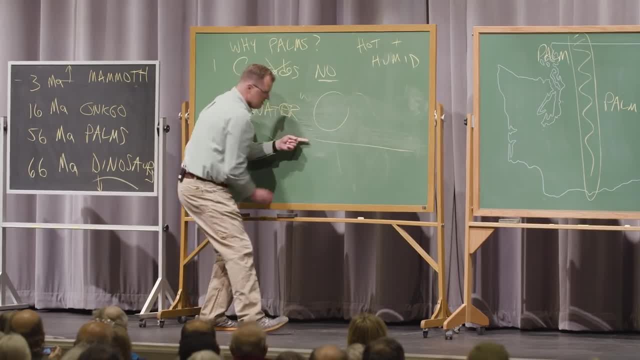 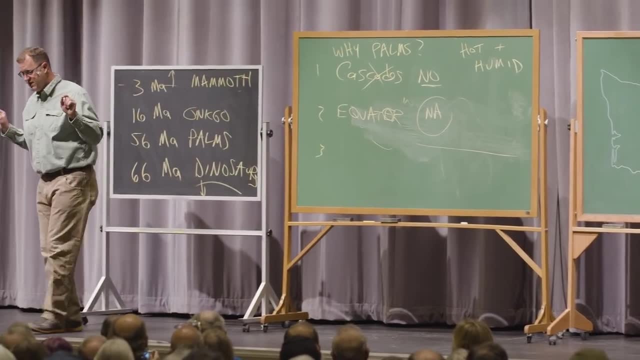 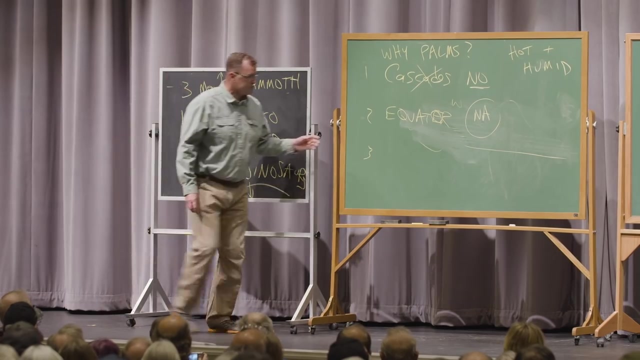 So here's the concept, Here's the equator. North America today is completely north of the equator. The latitude here is 47 degrees north. So if you are a proponent of idea number two, you say: to explain the palms, we need North America. 56 million years ago to be partly in the Northern hemisphere, partly in the Southern hemisphere and to have subtropical conditions and even tropical conditions throughout much of North America. That is incorrect, because we know precisely where North America was 56 million years ago And it was not at the equator. 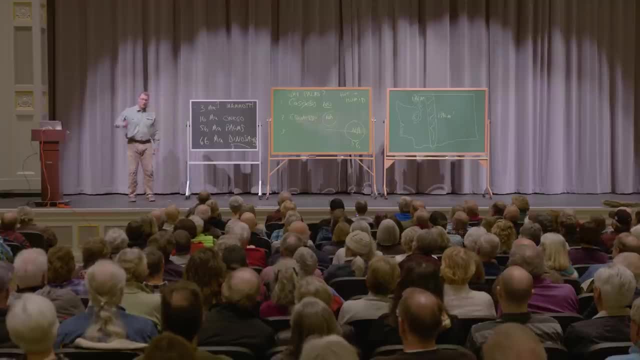 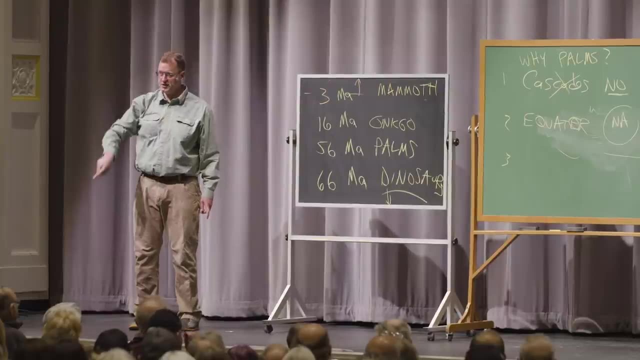 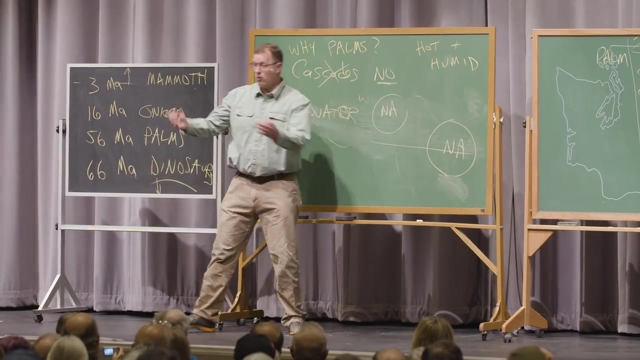 North America 56 million years ago was farther north than it is right now. We were further away from the equator than we are now. We weren't straddling the equator. I'll show you some beautiful animations in a bit to back that up. North America was straddling the 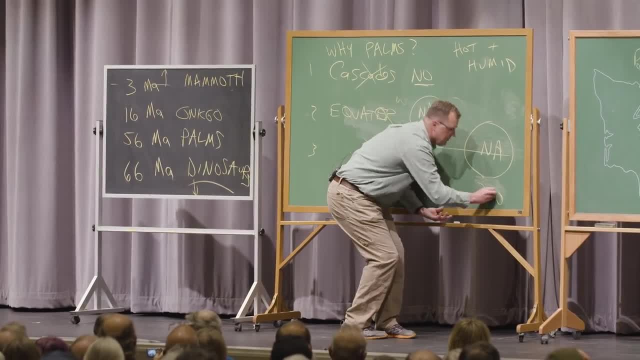 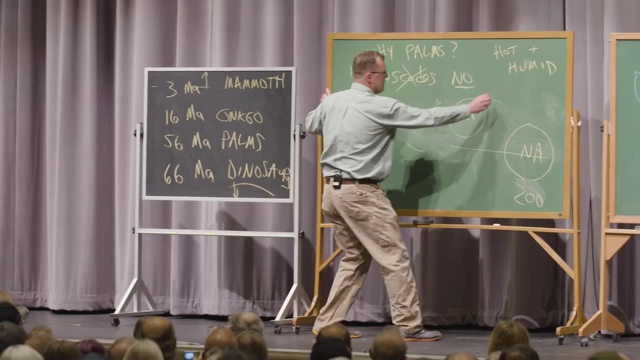 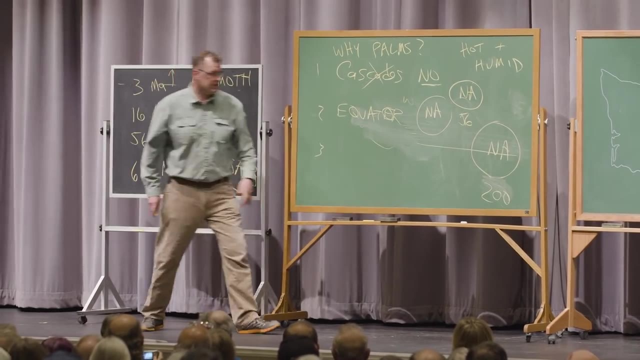 equator long ago. but that was back during Pangea time, That was back during the last supercar And that was the continent where Florida was in the Southern hemisphere. But if we put in North America 56 million years ago, it's farther north than it is today. So North America has done this. 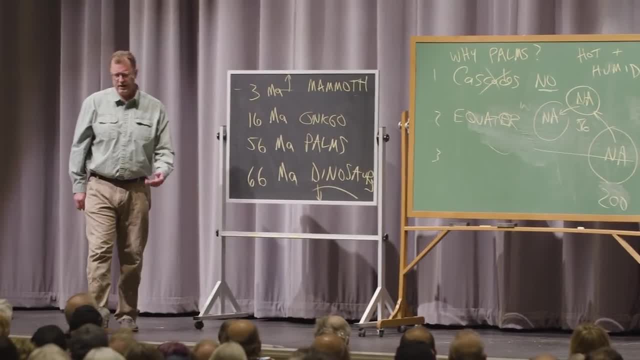 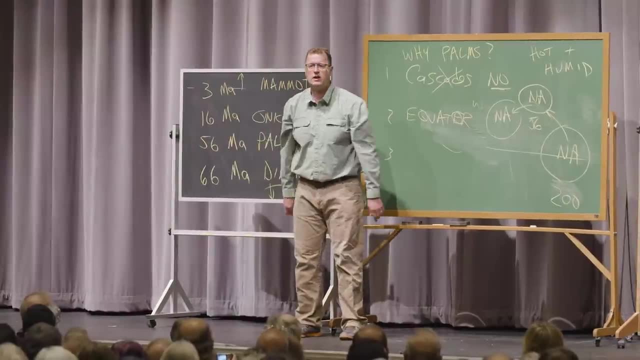 and then this in the last 200 million years, And you're like: well, how do you know that We have ocean floor basalts of different ages? We have ways to reconstruct where these continents used to be located, at different spots at different times. Nobody's arguing that when you look at the, the region, 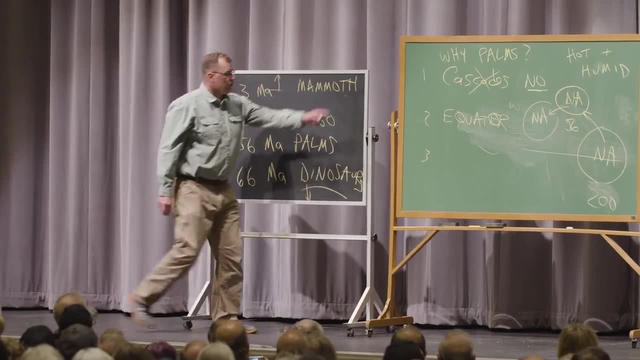 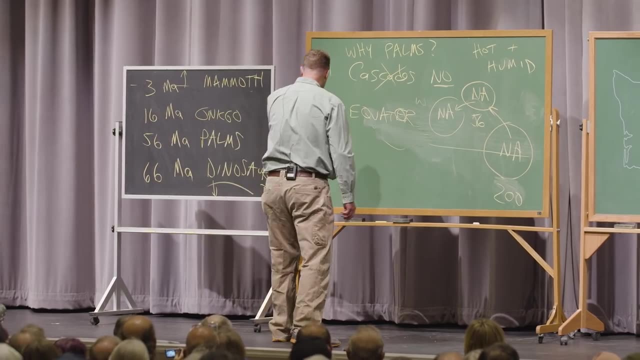 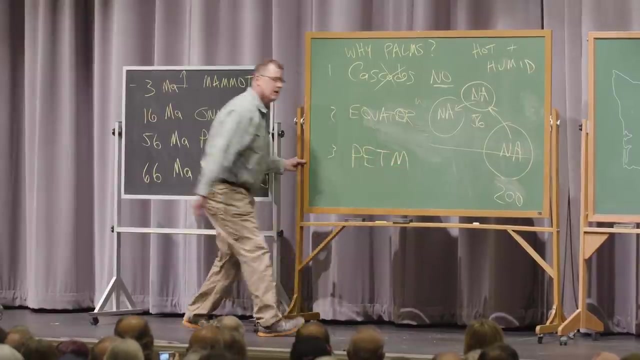 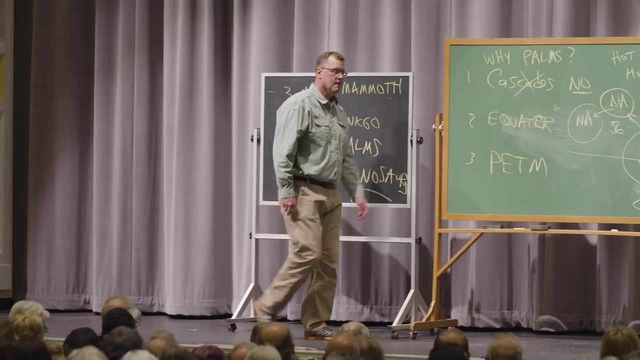 The research post-Pangea. So if one is incorrect and two is incorrect, what is the answer? I came for the answer you say. The answer is this: Petum P-E-T-M. It turns out that our palm fronds in Washington. 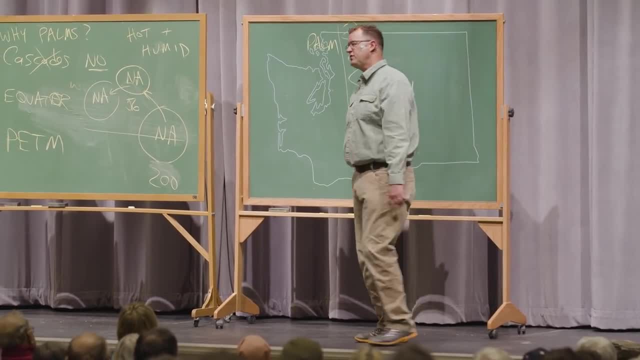 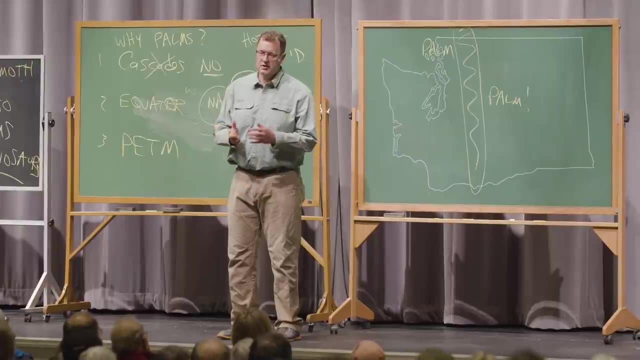 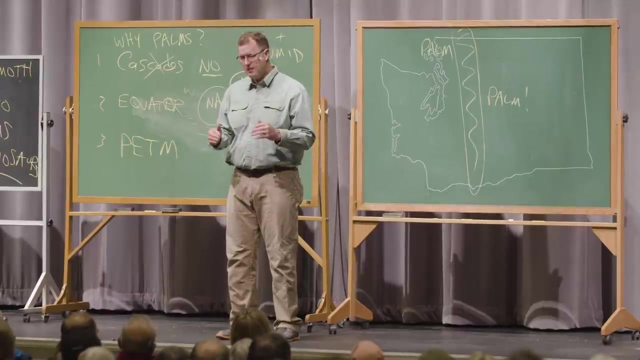 are not a Washington story. They're not even a Pacific Northwest story. It's a global story. There's a bunch of new evidence now that, starting about 56 million years ago, there was a dramatic increase in global temperatures. It happened very quickly. A bunch of carbon was pumped. 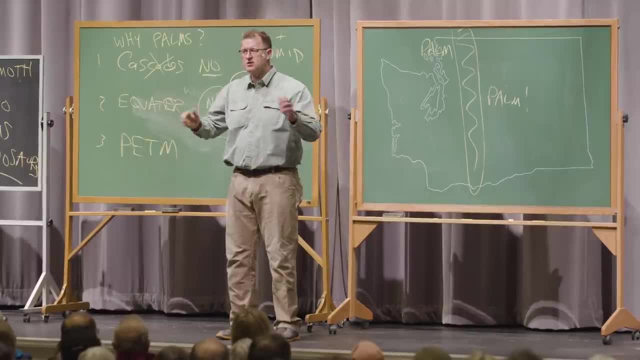 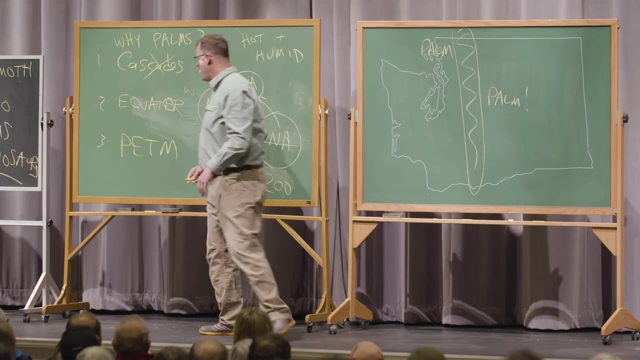 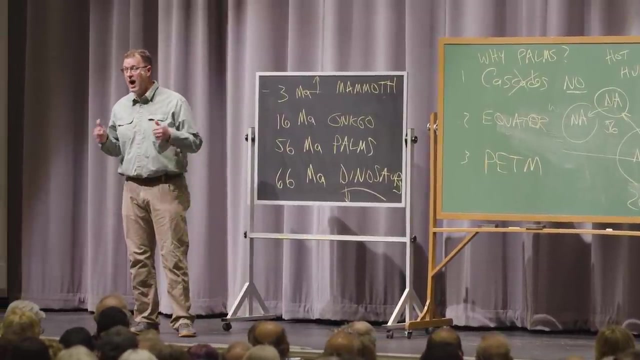 into the atmosphere and we have plant fossils, We have sediments on the ocean floors, We have all seven continents recording this dramatic P-E-T-M. It's called the Paleocene-Eocene Thermal Maximum. That's a mouthful, It's a hot time. The Paleocene-Eocene Thermal Maximum. It's still a bit of a mystery why that. 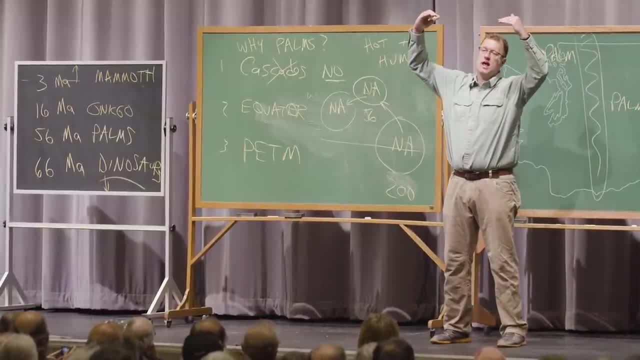 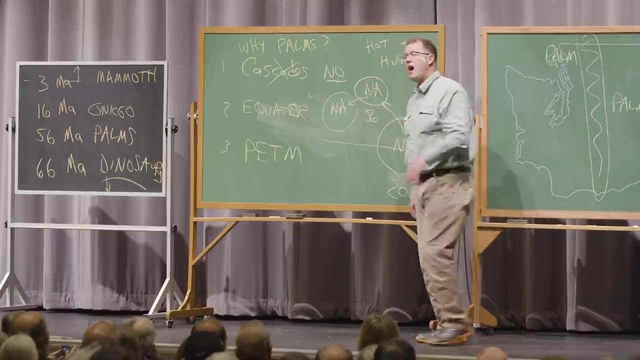 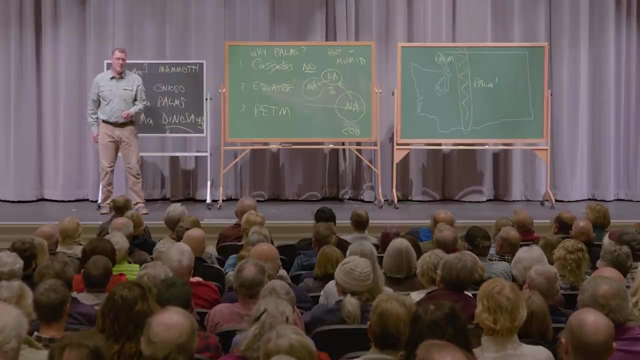 event happened. Why? that sudden spike in temperatures lasted a couple of 100,000 years and it ended pretty much as quickly as it began. And we as a globe have not been as warm since that time million years ago. Are you hearing what I'm saying? I'm saying that our palm fossils just north of 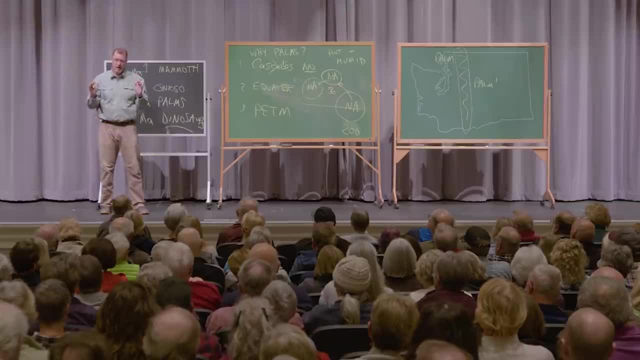 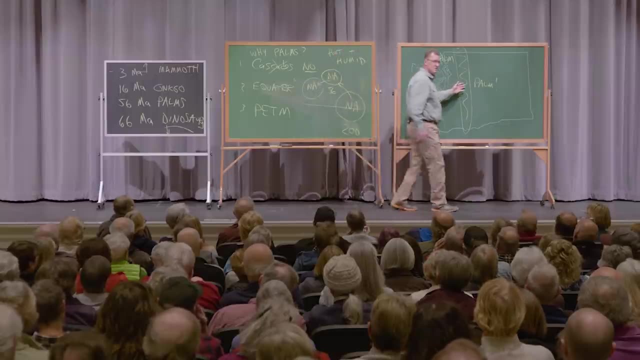 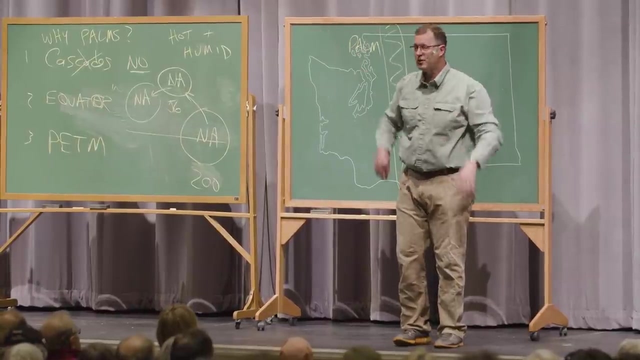 town are part of a global warm event. I've got a couple video clips to show that as well. but we have palm trees at this time. We have palm fossils at this time in the Arctic. We have palm fossils around the world at latitudes that make no sense with their current global position. So that's the 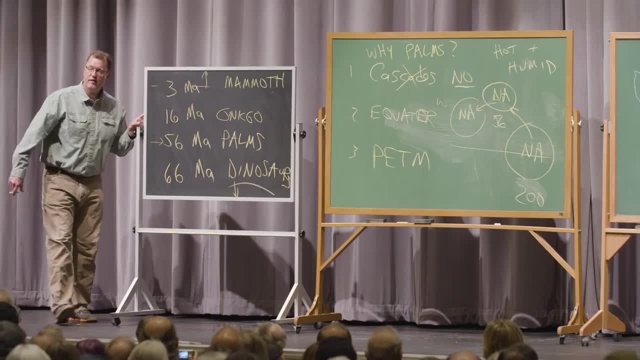 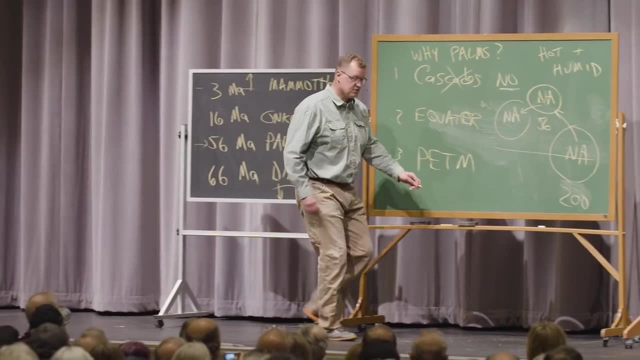 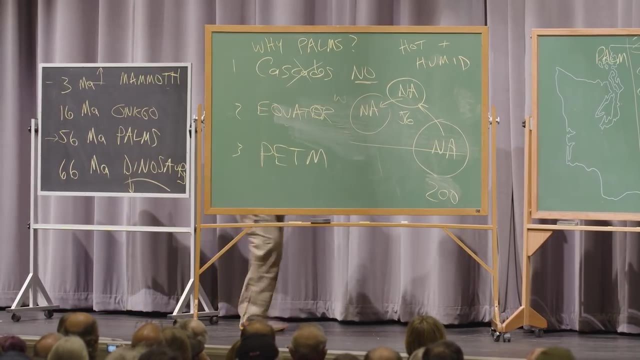 first major message tonight: Some of these plant fossils are telling us about a global climate history, and we'll leave it at that until we get more images to look at in just a bit Wonderful. Let's switch gears. Let's actually do a little razzle-dazzle here and flip the chalkboard around. 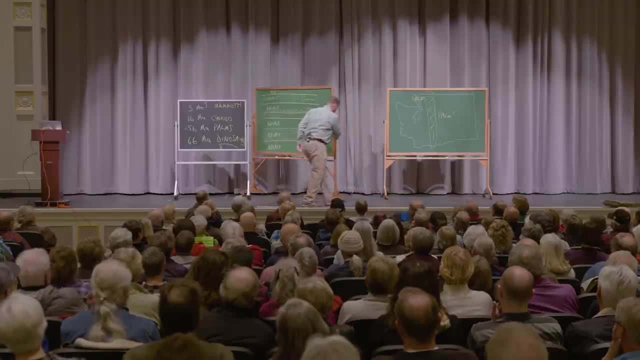 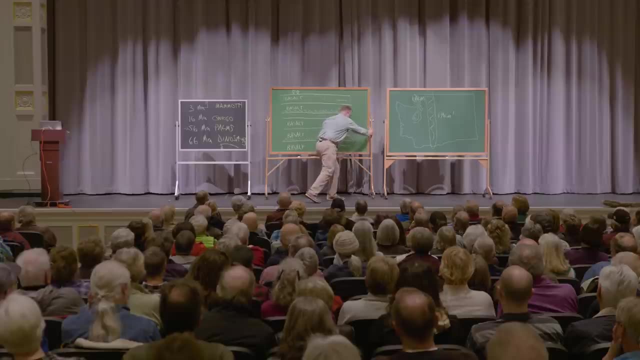 I was ahead of you now. I was in here washing the chalkboards and drawing out something because I knew I wanted to make sure we got to enough time to make this all work in front of you. So you with me, We're leaving the time of the palm fronds temporarily. We'll have all sorts of 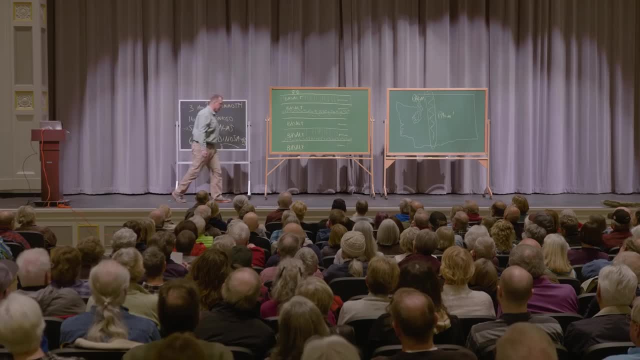 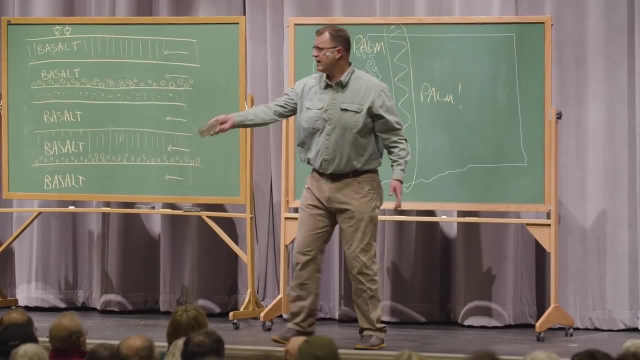 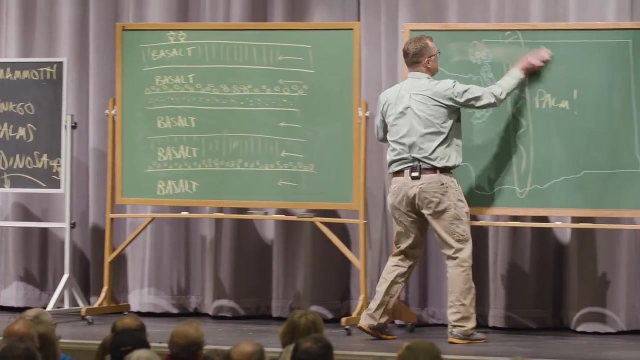 visuals to look at. but let's go closer to present day. Let's go 16 million years ago and go to the time of what kind of trees? Ginkgo trees? What kind of rock Basalt? Now we're out in the desert, We're leaving our current Wenatchee National Forest and we're going out into the 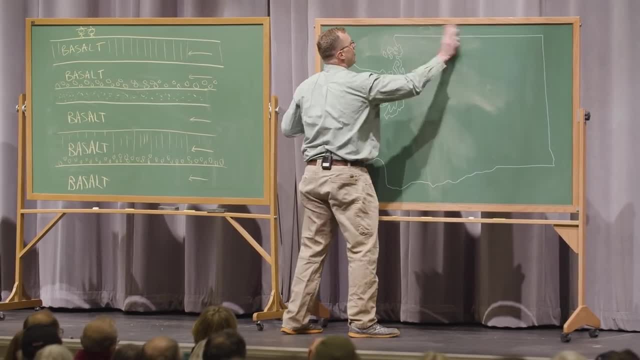 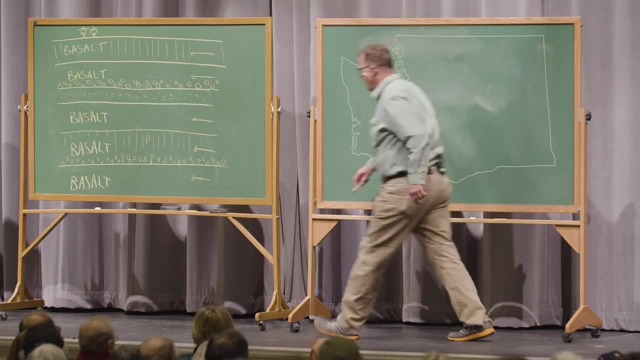 desert And many of you are local and many of you know about the Ginkgo Petrified Forest State Park. That is our focus now for the next, for the next 10 minutes or so, Okay, wonderful. P-E-T-M. 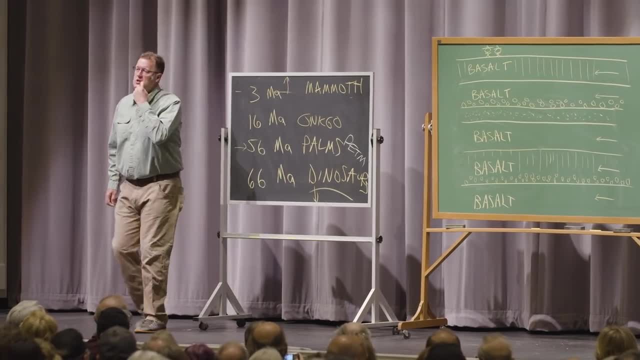 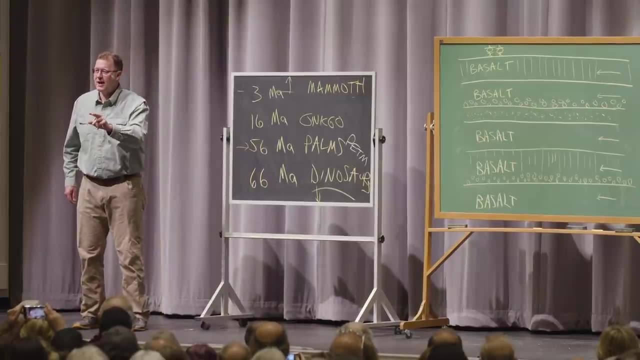 You know what? That's too awkward. Let's come up with something else. Let's, from this point forward in this lecture, let's call that that hot time: 56 hot. Okay, like I'm a quarterback, all right. Like I'm, like I'm on the line of scrimmage, I'm auditing audible here- 56 hot. 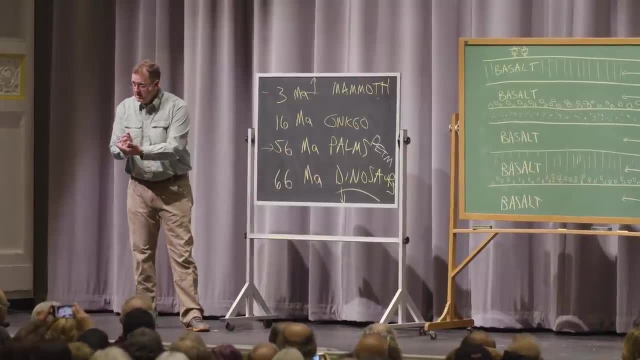 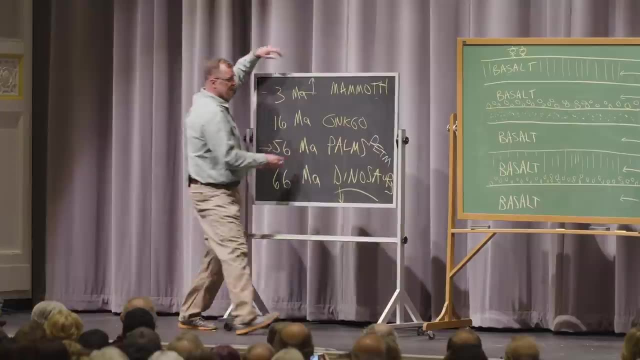 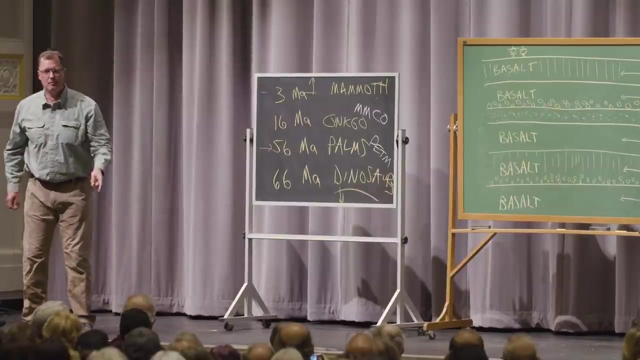 56 hot. Okay, So 56 hot 56 million years ago, global warm time. Now there's another one of these climatic changes: 16 million years ago, M-M-C-O- also awkward- mid-miocene climatic optimum. This is less. 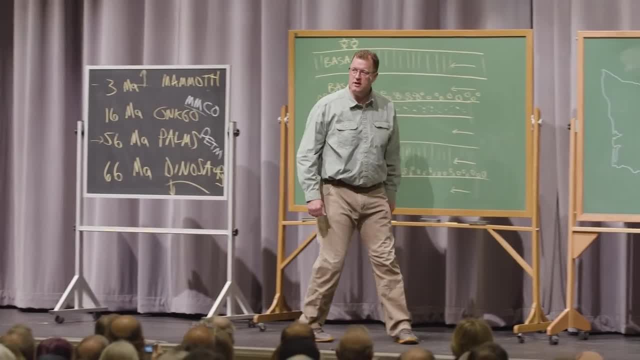 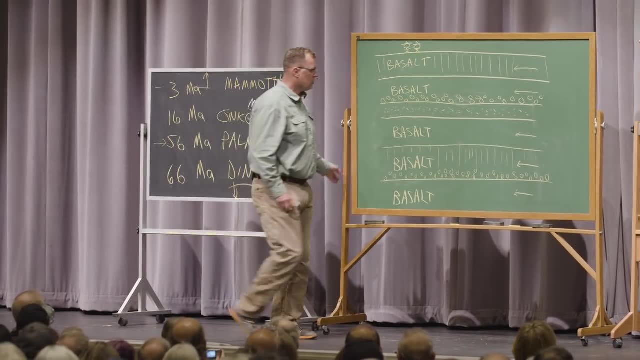 important, so I'm not even going to repeat it. We're not going to use it that much, But this is another time that we're choosing because there's this change. There's a kind of a mysterious change in global climate. Okay. 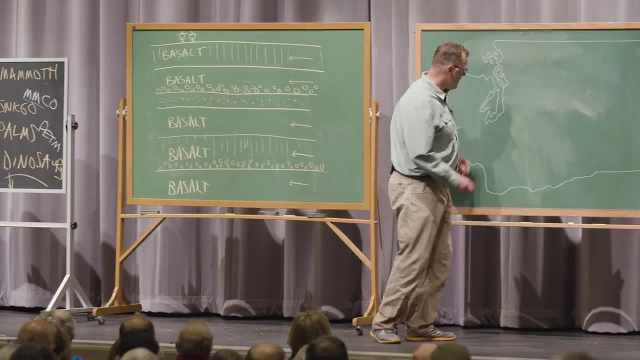 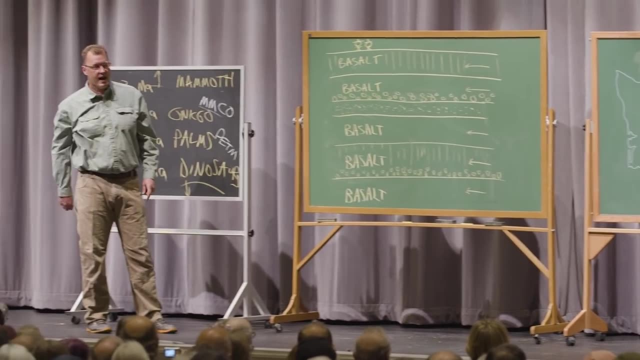 Out of Blewett. Pass You okay over there, All right. So Vantage is here. We are focusing on Vantage. This horizon goes over to Yakima Canyon as well. We have many. of you know this, we've had. 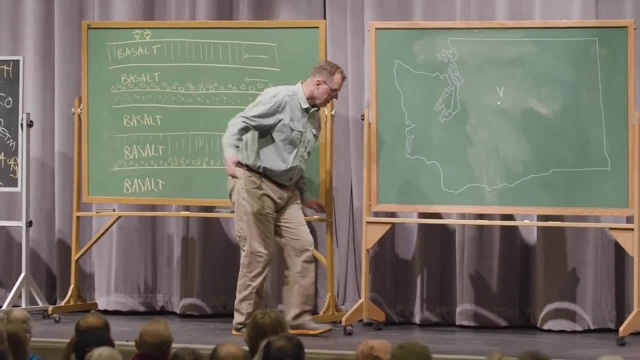 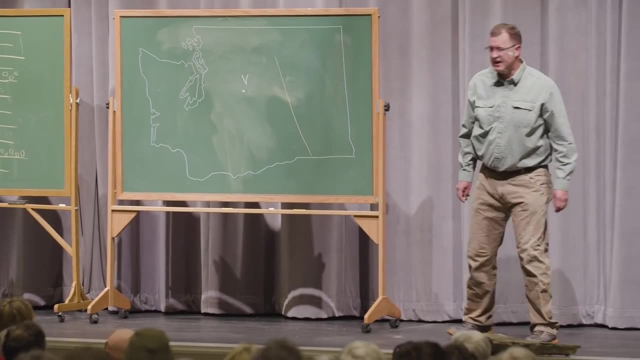 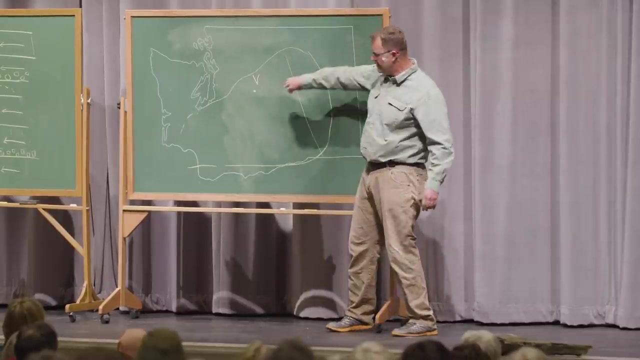 many lectures on this. This is the time of the great lavas. The great lavas where a huge fissure opens up over by Moses Lake 16 million years ago And, coming out of that crack, an amazing lava flow Comes out of the crack and generally flows to the west Parts of this Ginkgo lava flow. 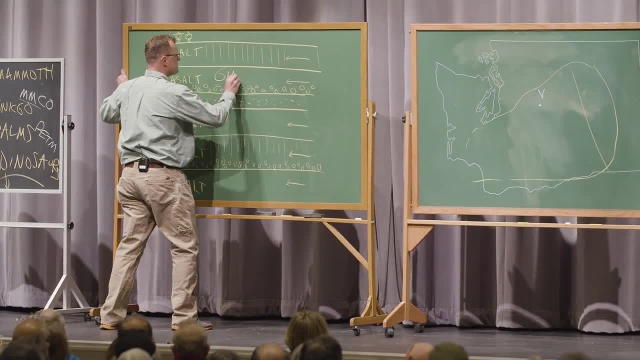 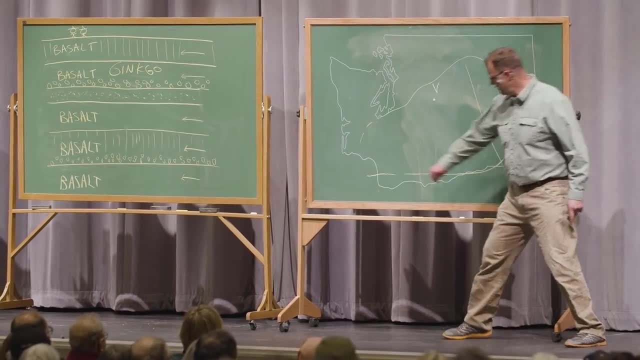 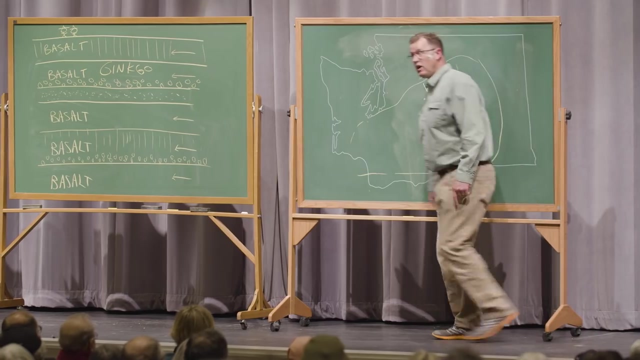 there I named it. The Ginkgo flow is the star of the show. Goes all the way to the Oregon coast. Parts of the Oregon coast are made out of lava rock that came from a crack near Moses Lake. I'm not making this up. And the Ginkgo lava flow is important to us tonight because, if I use white 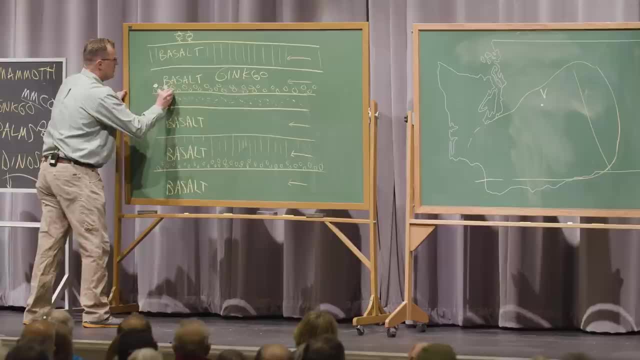 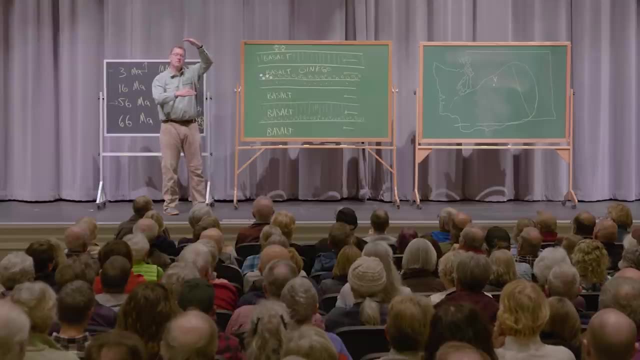 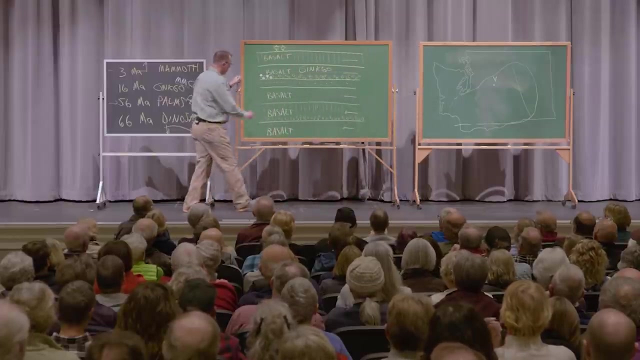 it's the Ginkgo flow. One basalt lava flow out of a stack of 300 of these flows, And each flow has their own crack. by the way, We're just zeroing in on one of 300 basalt flows And it's got all. 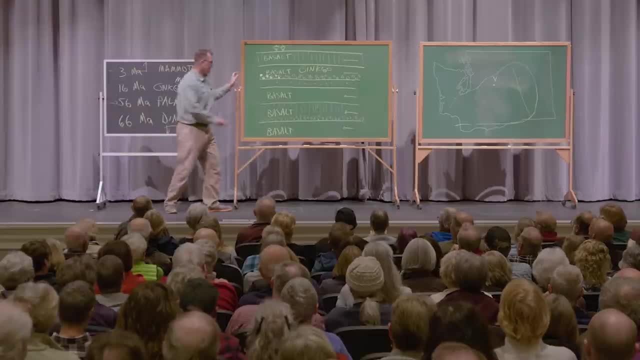 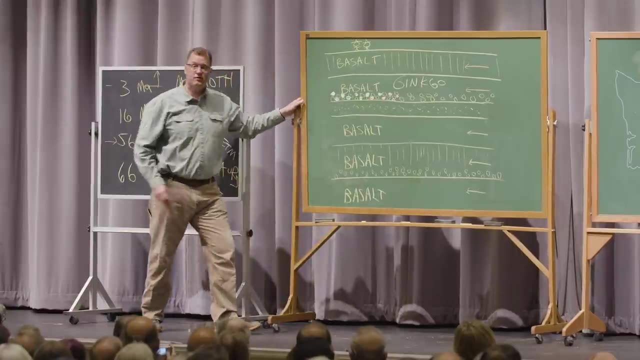 the wood. It's got all the tree trunks in it. It's got all the tree trunks. So these white circles are logs, Petrified logs, And there's a major mystery that remains with these logs. And that's what I want to. 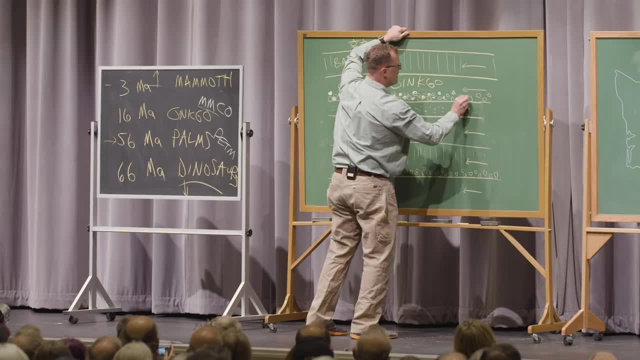 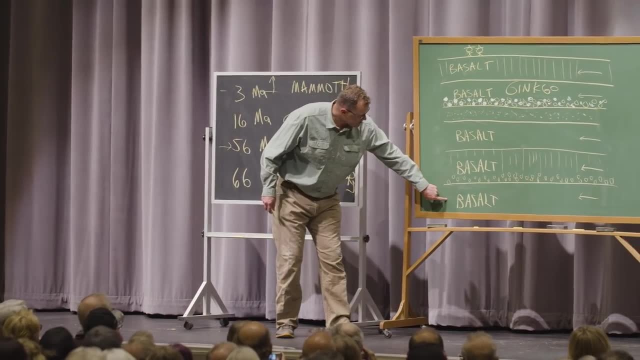 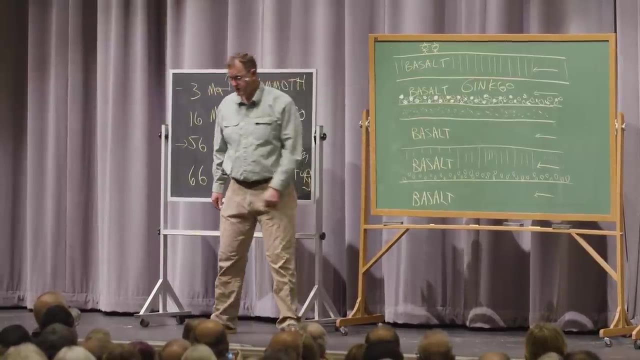 get to before we turn our attention to the visuals. So you're like, I thought these other circles were the logs. I was way ahead of you. These are not logs. So here's one basalt flow, another another, another, another. I've got five on this sketch in cross-section. Here's people walking around on the. 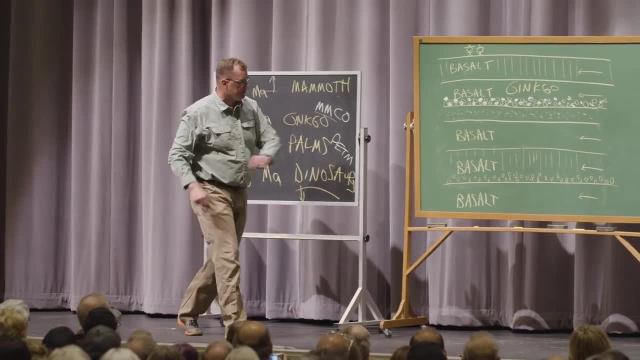 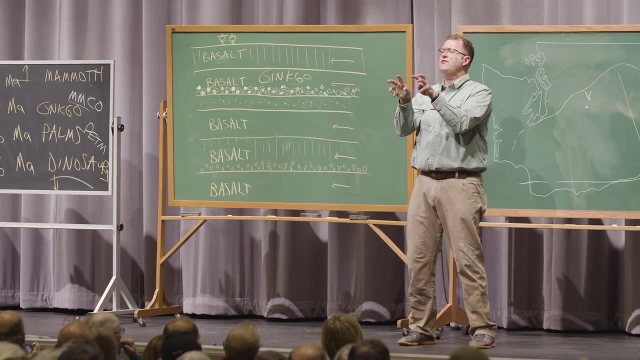 surface And some of those basalt lava flows have these circular features at the bottom called pillars, Pillows, And pillows are these strange kind of circular looking features. They look like brown basketballs in cross-section, But I'm doing this with my fingers because pillows are actually. 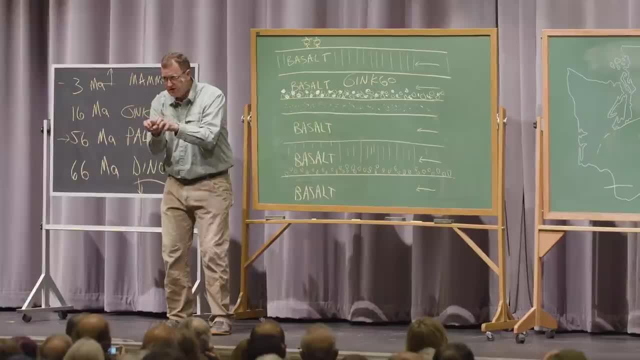 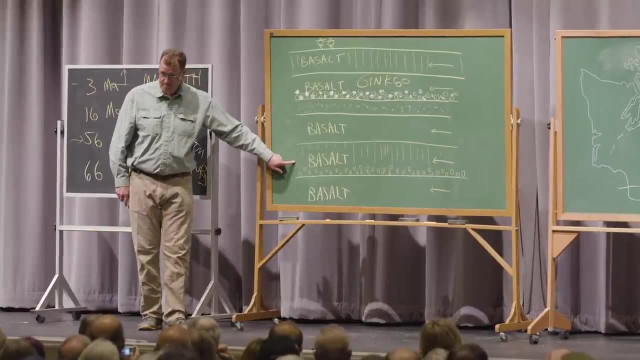 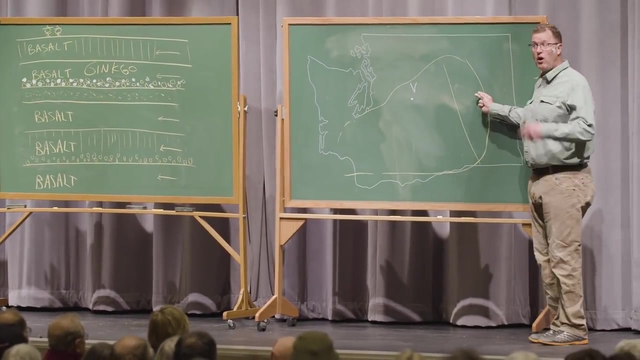 crackling fingers or crackling worms of basalt going out into water. That's a key part of our story. So this flow came in. It has pillows at the base. That means there was a crack over here in eastern Washington. It produced some basaltic Hawaiian-like lava. 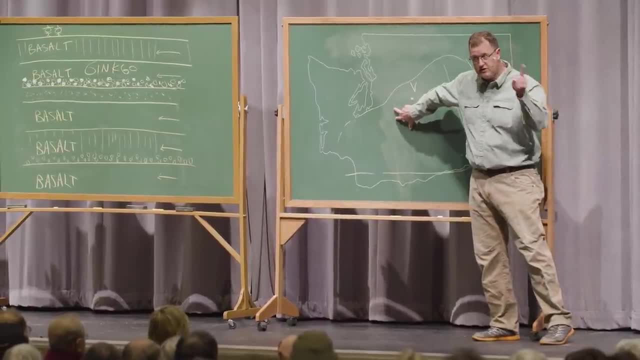 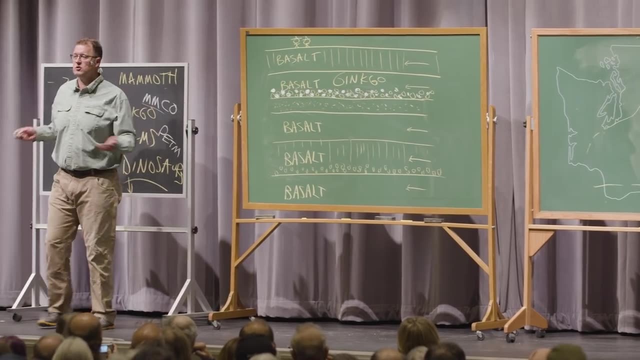 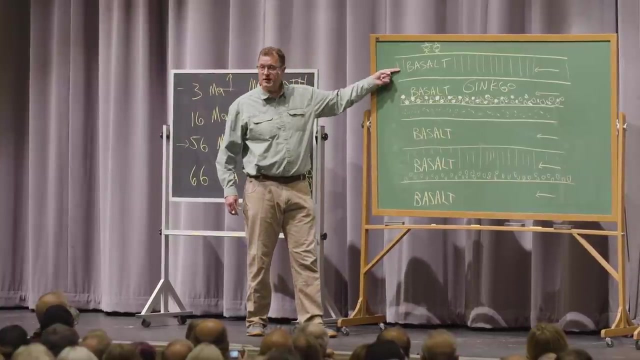 It flowed into water in central Washington. Pillows mean water, But not all the basalts have pillows. Here's another basalt layer: lava flow. It doesn't have any pillows at the base, which means it flowed over dry land. And then another flow, the Ginkgo flow, has pillows, And then this one. 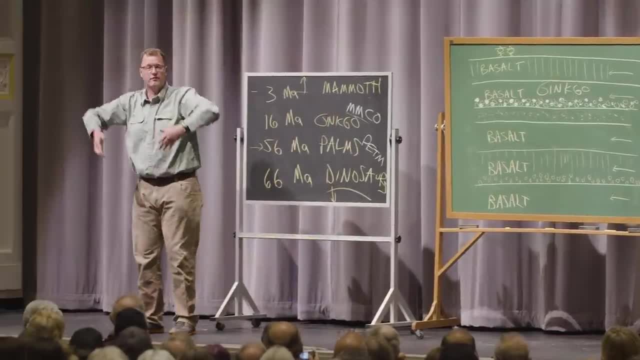 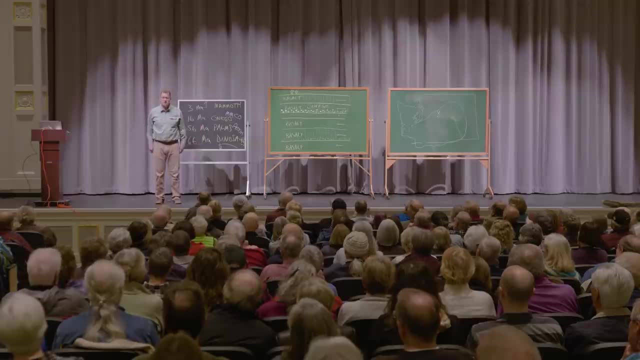 does not. By the way, some of the basalts have wonderful vertical cracks to form columns that many of us know. Other basalts don't have columns. They don't have cracks. This is a mystery, But we're not talking about that. We're talking about the basalt layer lava flow. It doesn't have any pillows. 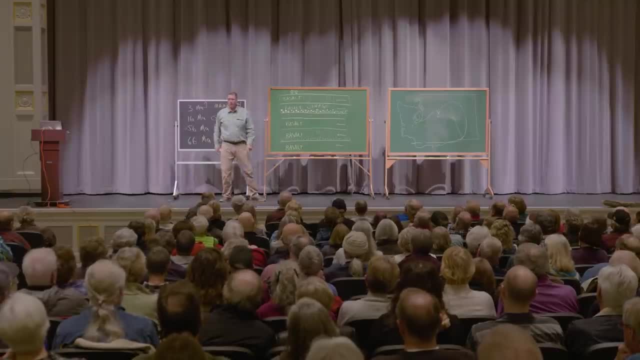 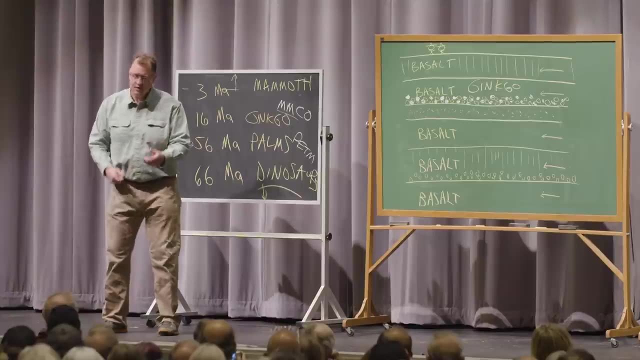 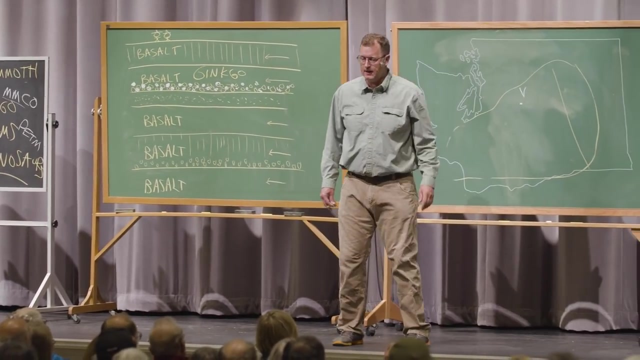 We're not talking about that tonight. We're talking about the Ginkgo flow yielding- and I'm not exaggerating- thousands and thousands of tree trunks that are in the lava flow. Now, before we quit, tonight, we're going to feature a gentleman by the name of George Beck, And he was the geologist. 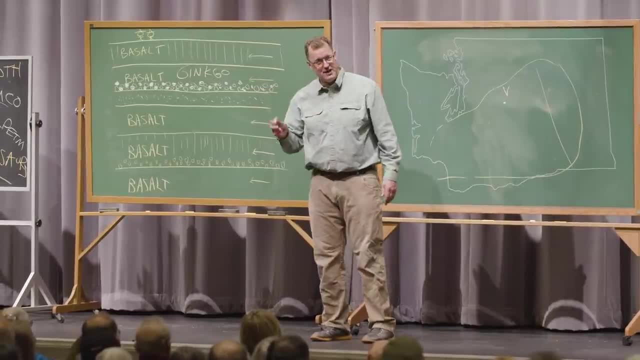 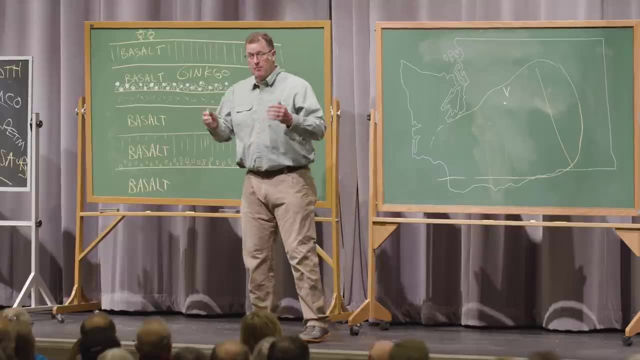 at the college here in town from 1925 until 1959. And his claim to fame was not only teaching students and mentoring students, but also teaching students and mentoring students. And he was a geologist and he was a nice fellow and he came to us one day. he came down to us at work and he 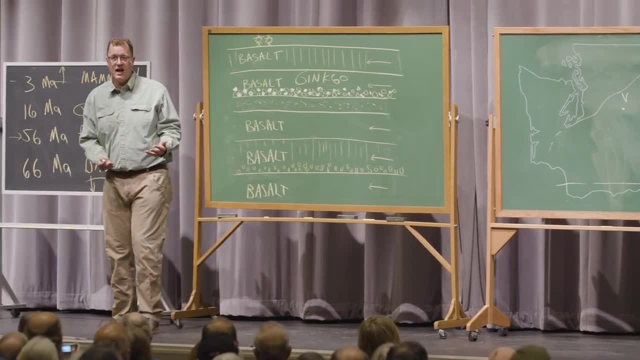 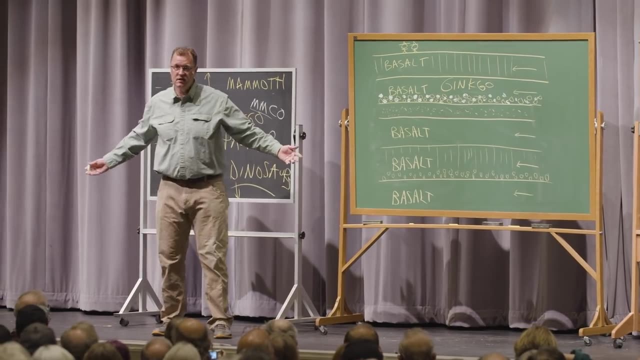 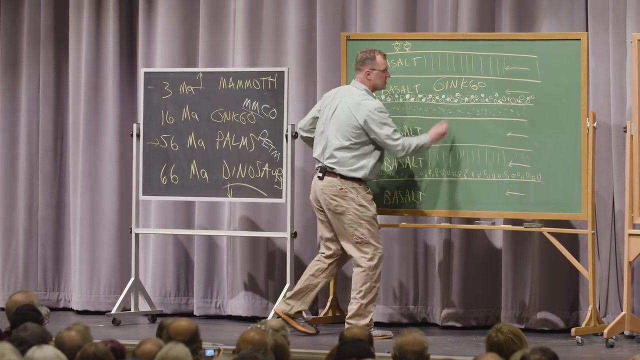 showed us a lot of tonight is coming right from George Beck's research. So he was studying all these logs that were you pulling right out of the base of the Ginkgo flow And he was a laughingstock. That's maybe too strong. 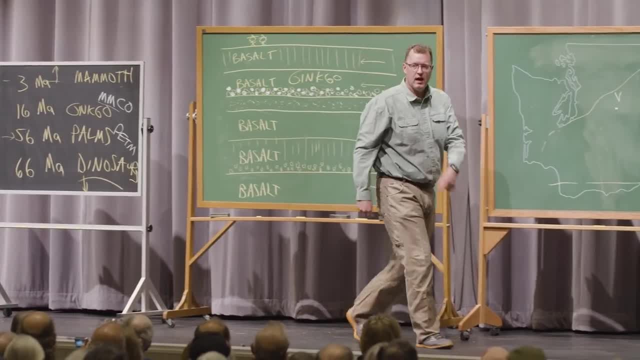 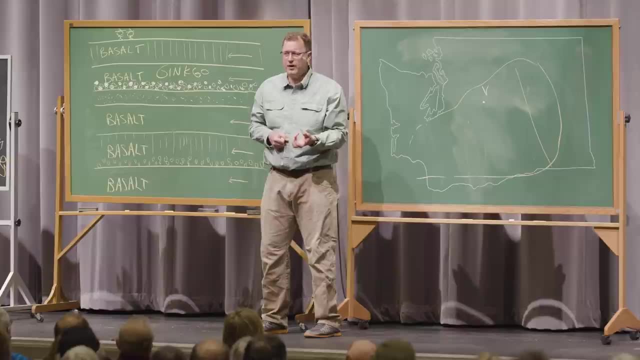 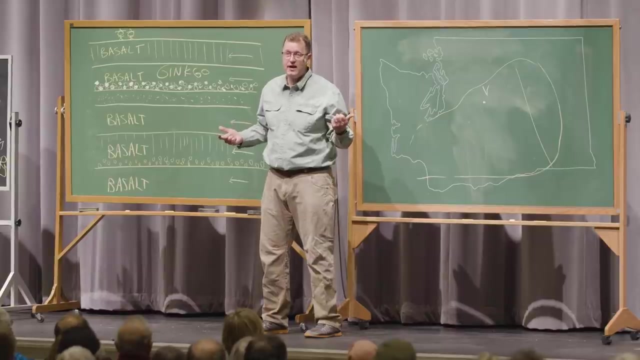 be too strong. but he got challenged by a lot of paleontologists around the world when he started publishing papers. They say, George, you can't pull petrified wood out of lava. That's impossible. And he says: why don't you take a trip over here to Ellensburg and I'll show you We'll go out to? 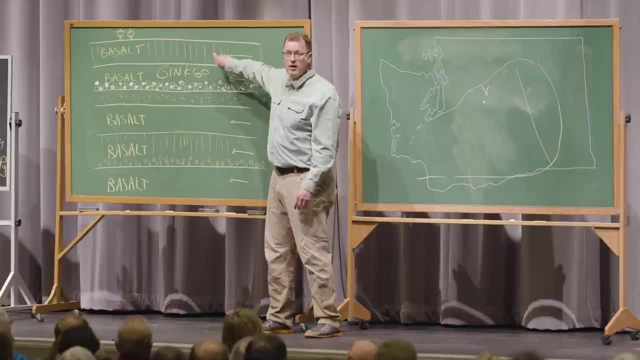 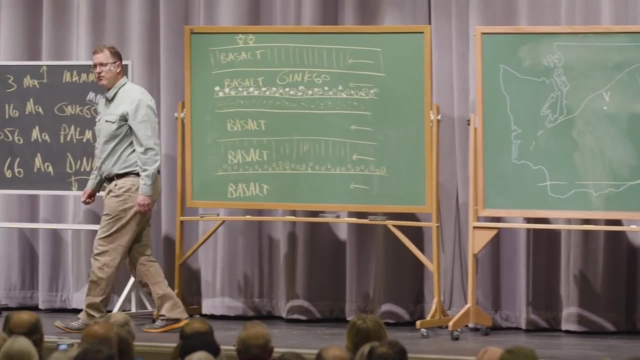 Vantage. I'll show you. There's no wood below, There's no wood above. There's wood right in the pillow zone of the Ginkgo flow And they're like: well, how did the log survive? Why didn't they? 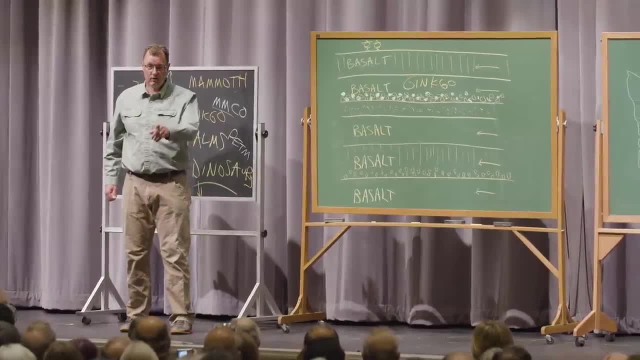 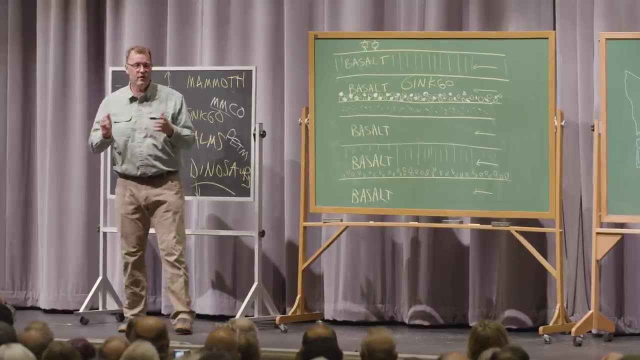 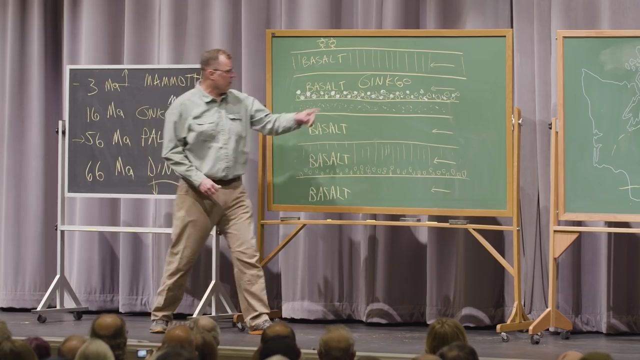 just burn up in the heat of the lava? You know the answer. There's pillows and logs together. And what do the pillows mean? Water. The water is there to protect the wood. The logs were waterlogged And there was all sorts of steam and other drama when the Ginkgo flow came from the 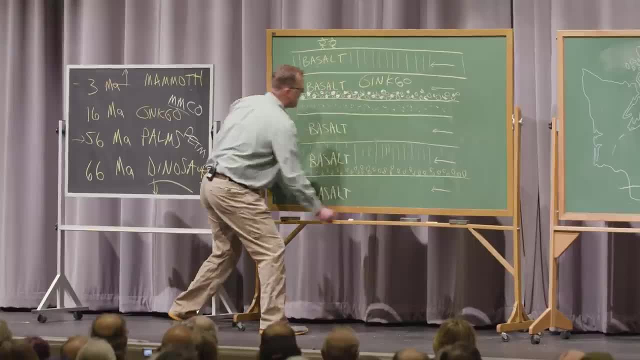 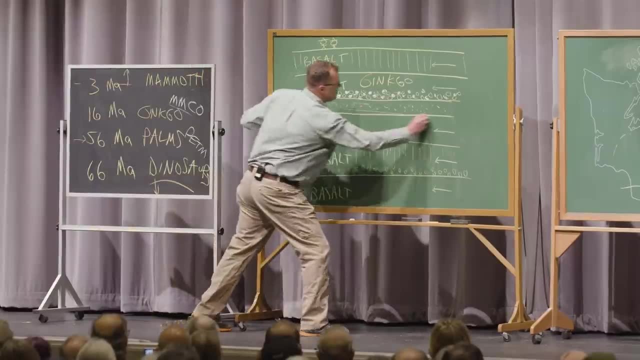 east and flowed into the area. So with a lot of the visuals tonight, we're going to focus on the wood at the base of the Ginkgo lava and this thing here, Which is not a lava flow, but it's a layer of sediment, It's a layer of sand, essentially. 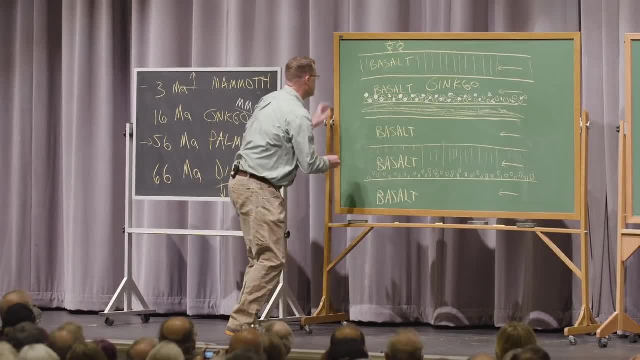 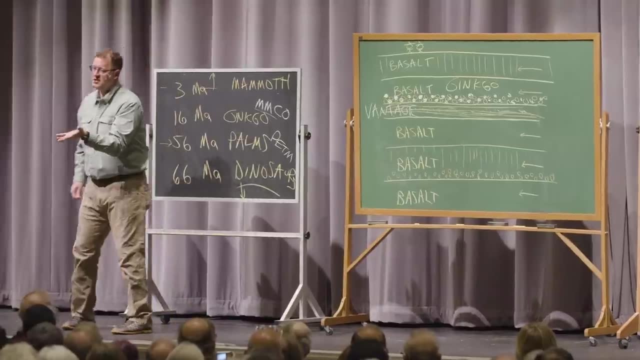 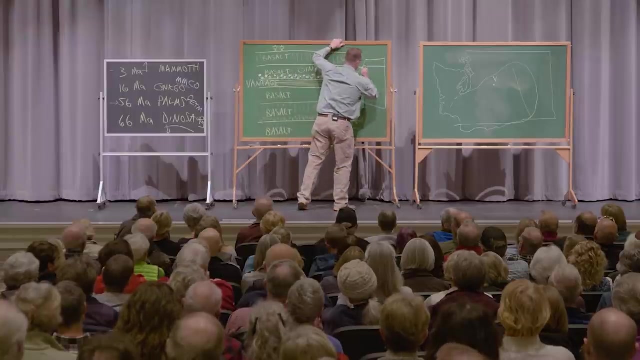 called the Vantage sediment. The Vantage sediment. We'll see a bunch of images with the Ginkgo lava flow directly on top of the Vantage sediment And there's been a lot of work recently. Let me enlarge the Vantage sediment for you here a little bit, if you'll allow me to do that. 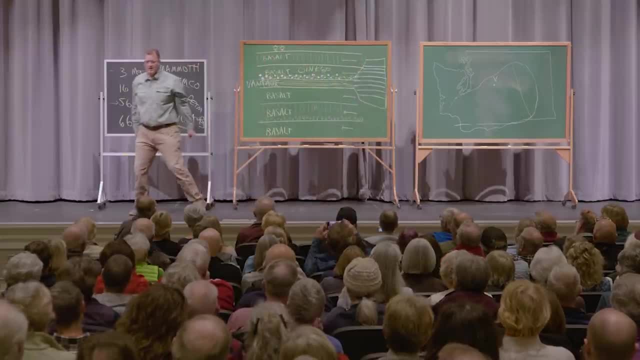 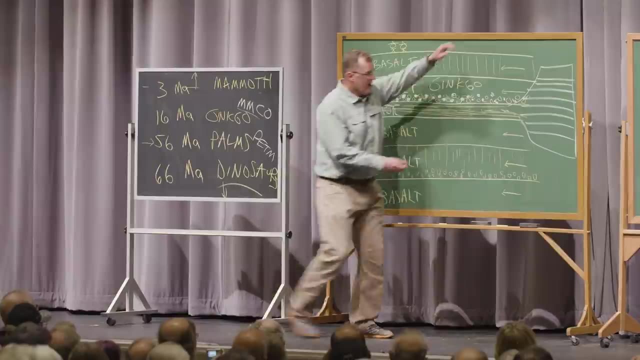 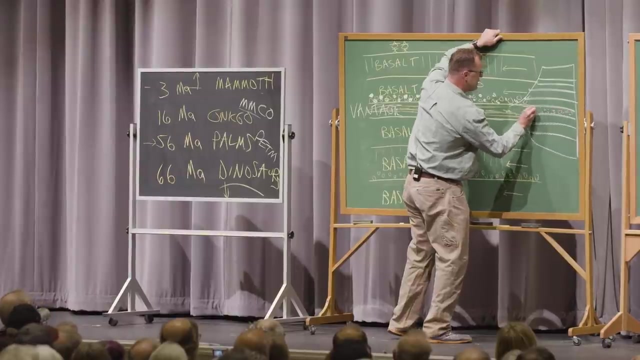 In many places the Vantage sediment has many layers And they're called graded beds, which means that each of these little beds in the Vantage horizon have sand grains at the bottom- I know it looks like pillows now, forgive me- And then we get finer and finer sediment as we go up. That's a graded bed, One sedimentary horizon. 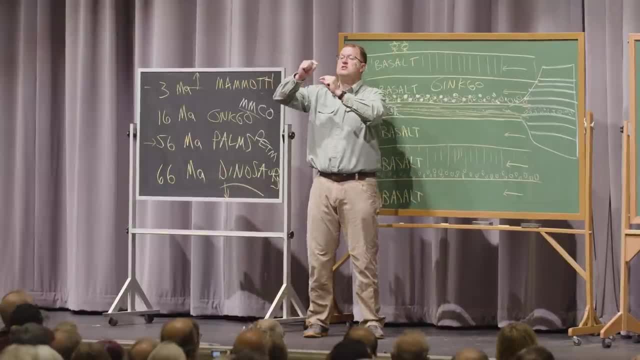 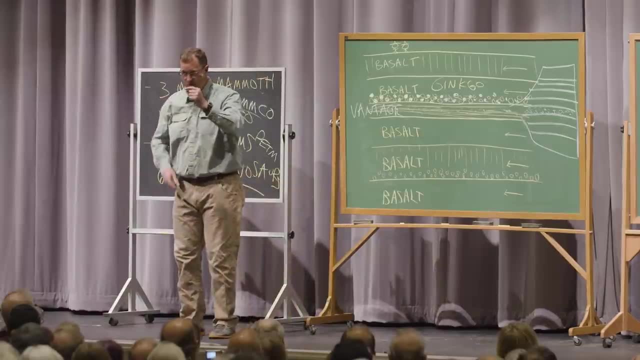 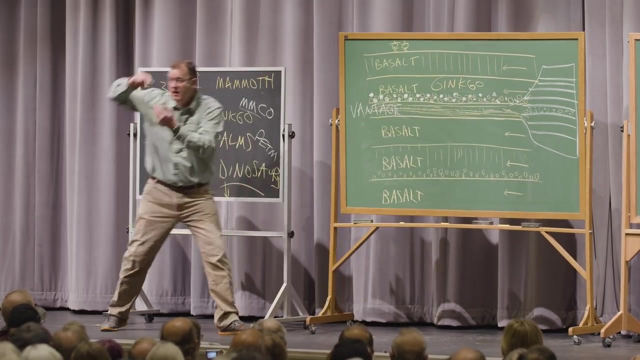 within the Vantage sediment that goes coarse to fine sediment. Then we jump to the next one of these mini beds. Same thing, Coarse to fine, Next one, Coarse to fine. Something is happening repetitively, whatever terrible grammar, within the Vantage sediment. 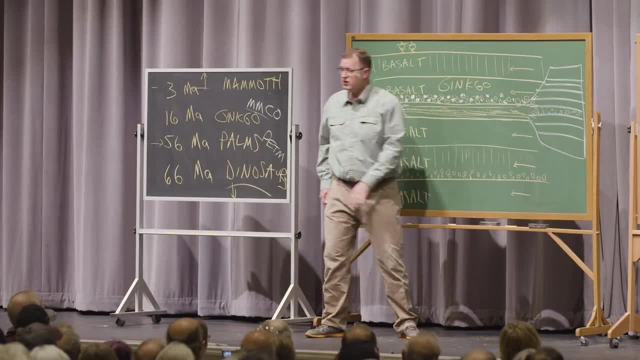 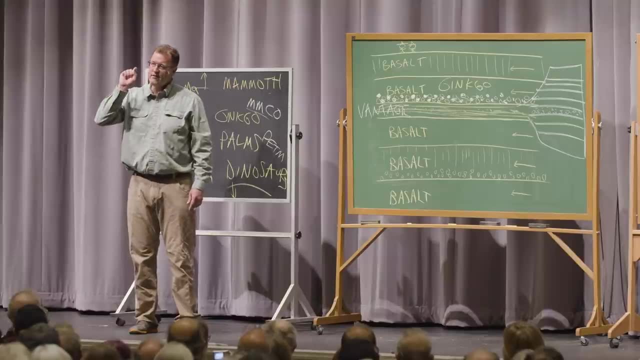 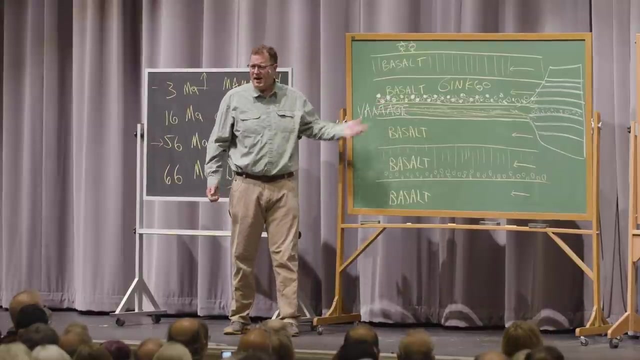 Do these little miniature beds have anything to do with these logs? I'm beating around the bush. Let me hit it right on. We still don't have a for sure answer why we have all of these logs sitting together. And you're like: what are you saying? What's so hard? You got logs, You already. 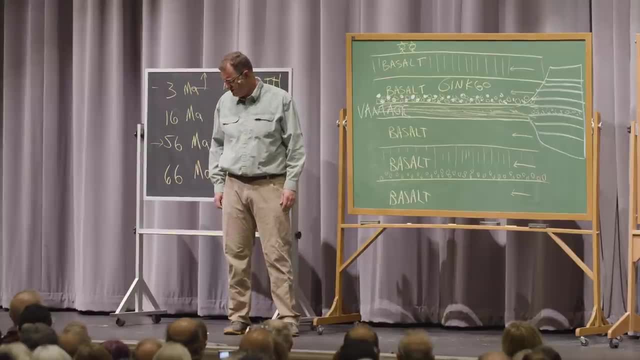 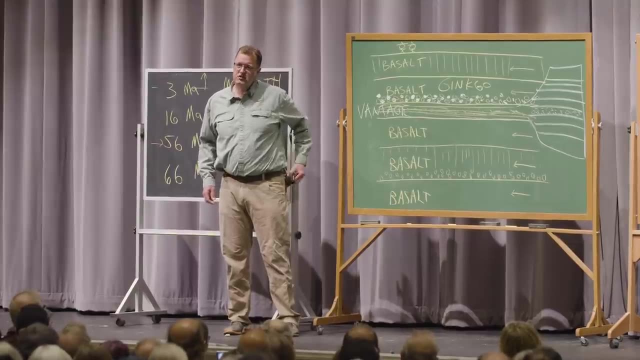 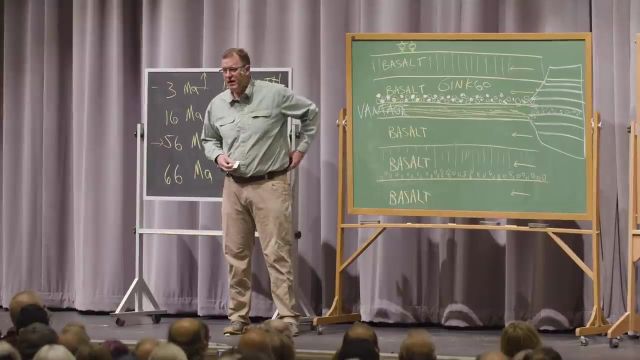 talked about it. The pillows are there, The water protected the logs. There are two dozen different kinds of species of logs sitting together. He goes to his wallet And in between the Safeway Club card and the Fred Meyer card, he pulls out a cheat sheet. 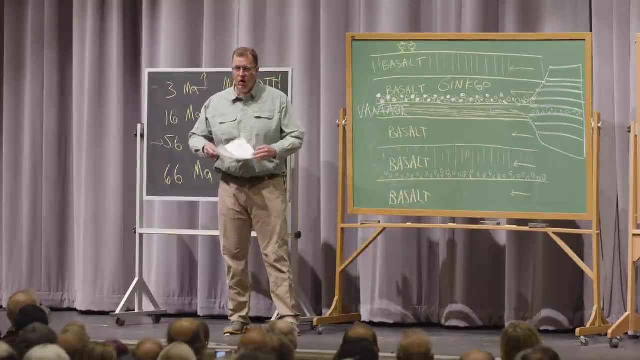 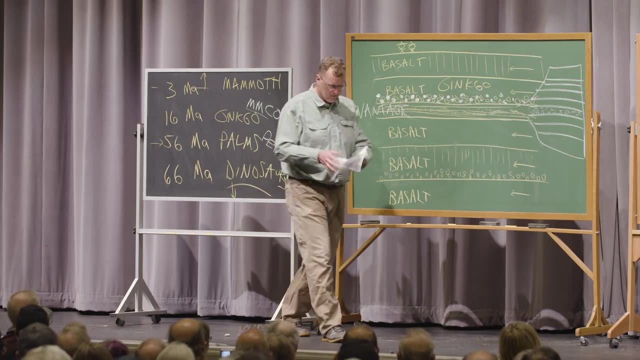 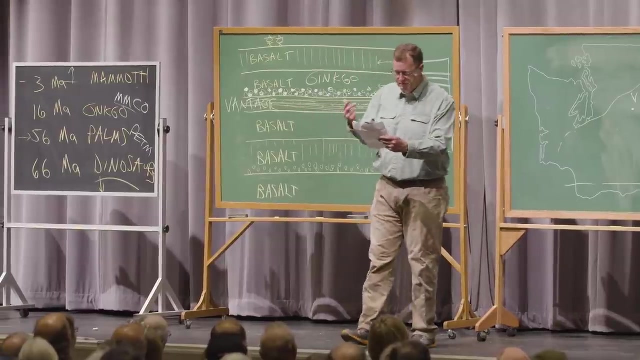 Let me tell you very quickly all the different kinds of tree trunks that are sitting next to each other in the lava flow. This is a freak show: Cypress, hickory, walnut, elm, oak, birch, beech, tupelo gum, sweet gum, cedar spruce, sequoia. 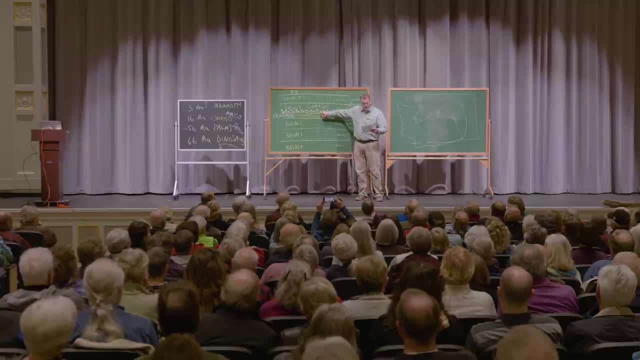 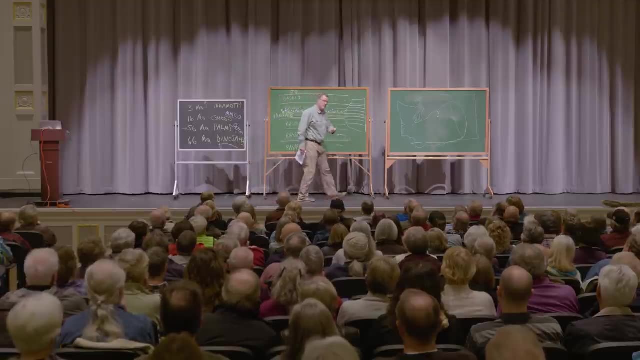 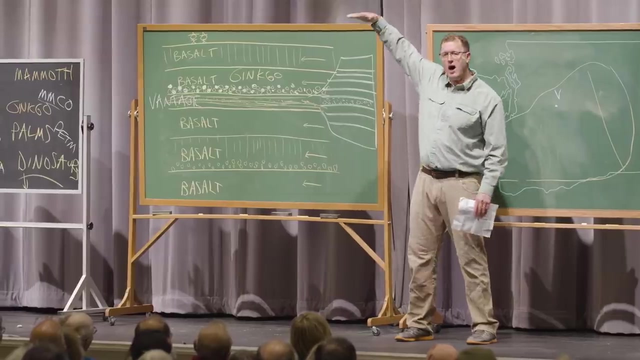 chestnut, Douglas fir, ginkgo, maple pine, All right in this layer. Now you know about trees. Not all those trees can live in peaceful harmony right next to each other, locking arms right. Some need uplands, Some need swamps, Some need something. 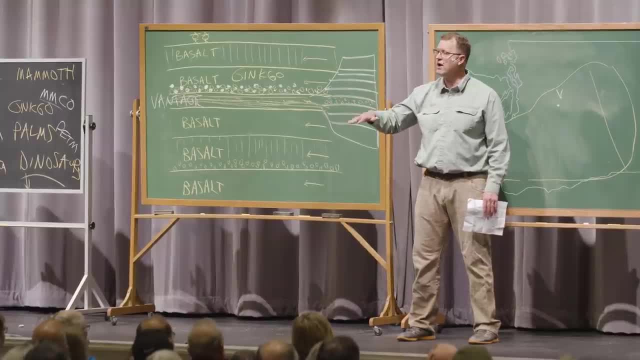 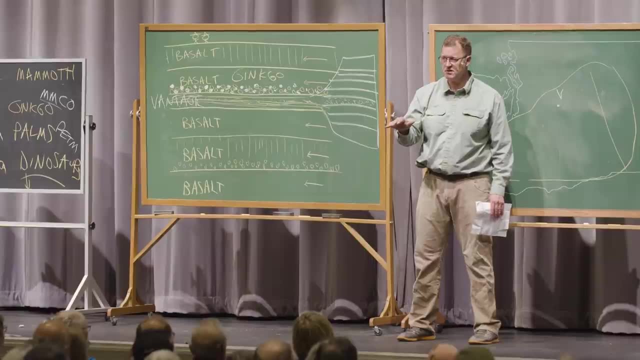 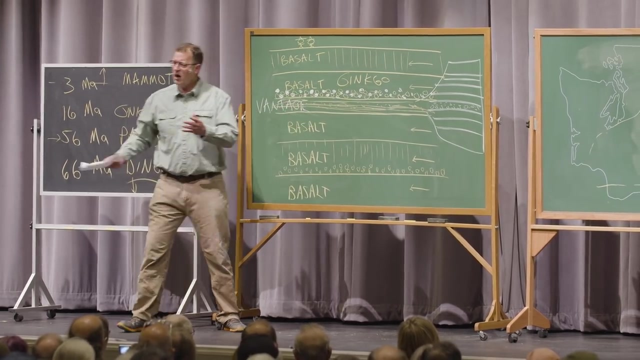 in between. These have to have been brought from a long distance. These tree trunks had to have been transported tens of miles, And the mystery is: where did they come from? Let me give you a little bit more about the wood. It's called the Ginkgo horizon and I focused on the Ginkgo trees, but 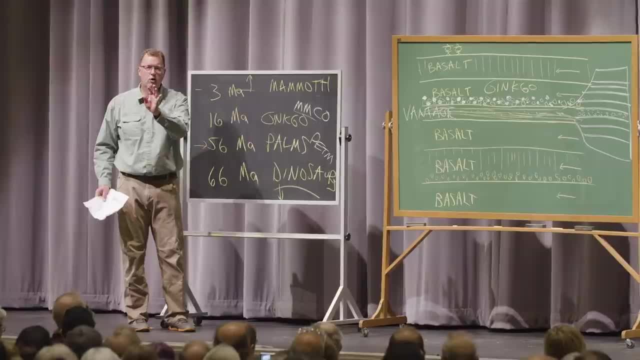 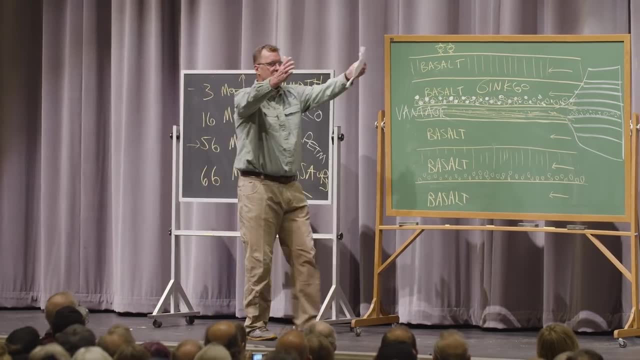 they are rare. There's hardly any Ginkgo logs in the base of the Ginkgo flow. That's maybe a surprise to you. You're driving on I-90, you see a brown sign that says Ginkgo- petrified forest. 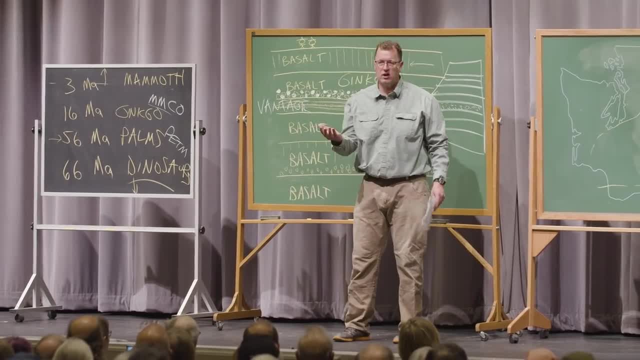 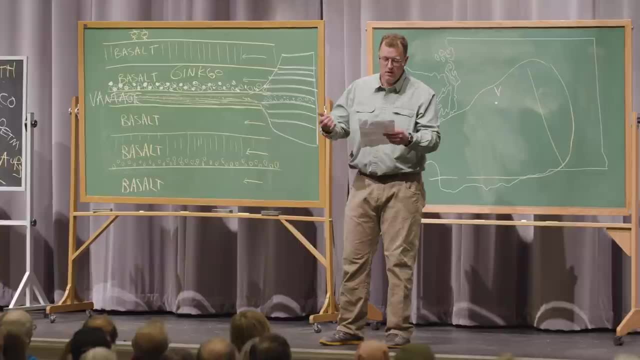 Hell, let's take this exit and see what this is all about. There's hardly any Ginkgo wood. Of the logs exposed at Vantage, 50% of them are Douglas, fir and spruce, 20% are elm, 5% walnut, 5% sweetgum. 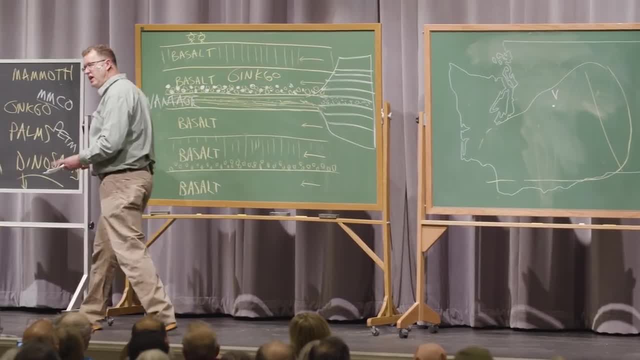 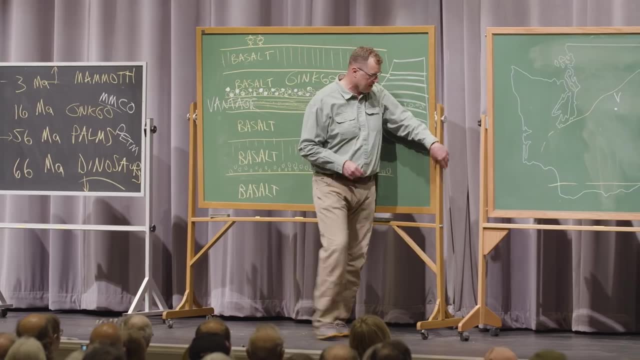 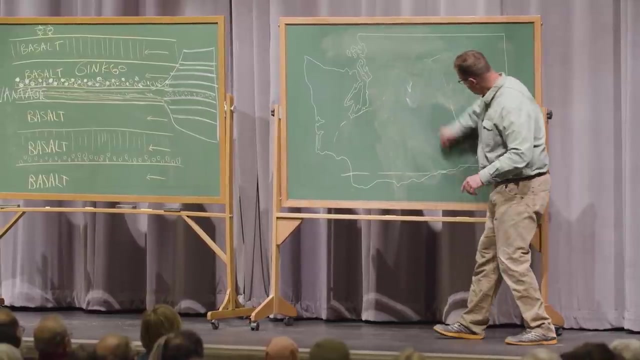 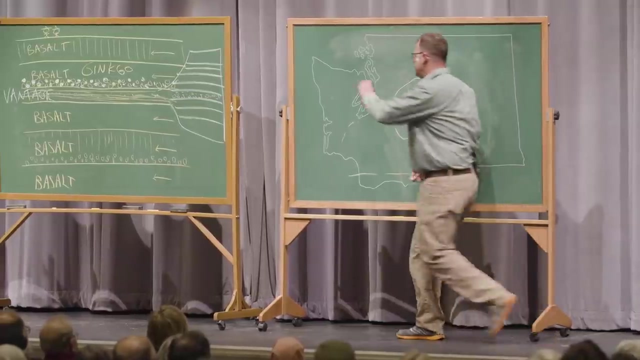 5% oak, 5% locust, rare Ginkgo. So the idea is we need to do something to get all these logs here Here in central Washington. and the last concept for the chalkboard is: after many of the lavas were developed, there was a lake called Lake Vantage. 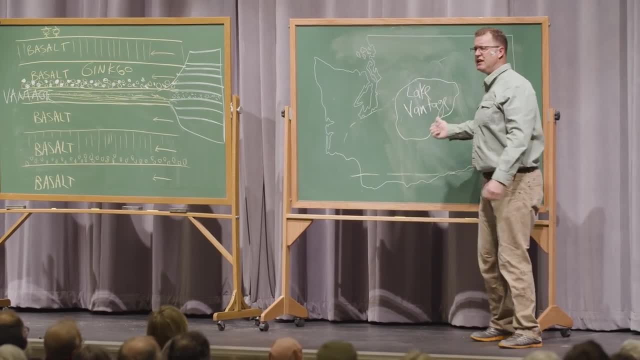 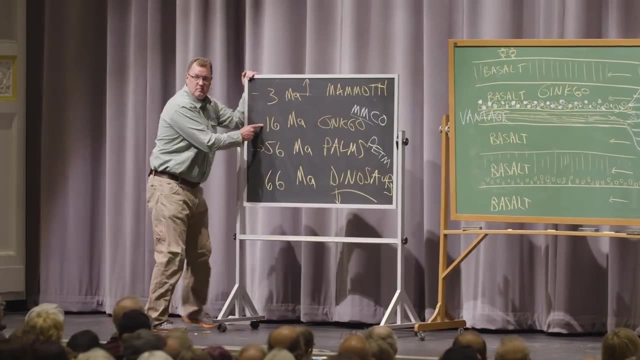 And you're like, well, wait a minute. now I've heard about this lake in central Washington during the Ice Age, and all the water got stopped at Wallula Gap. Remember: now we're at 16 million years ago. The Ice Age hasn't begun yet. We are pre-Ice Age. This is 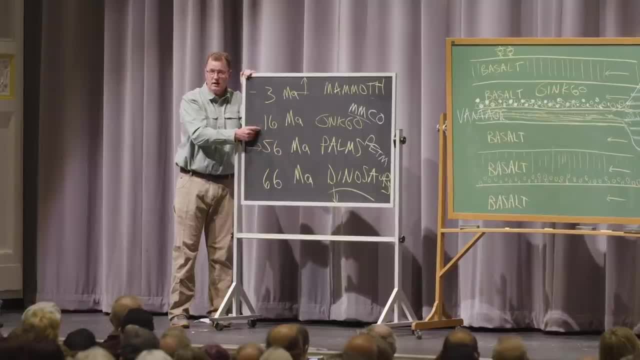 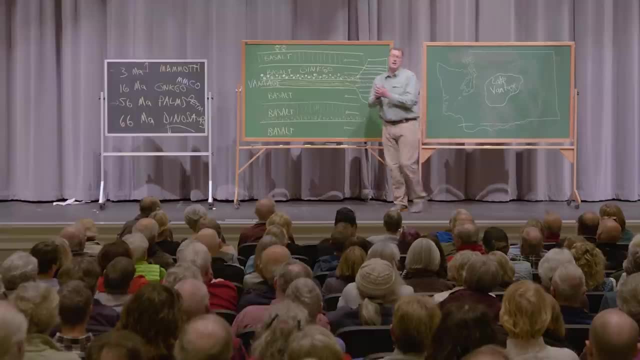 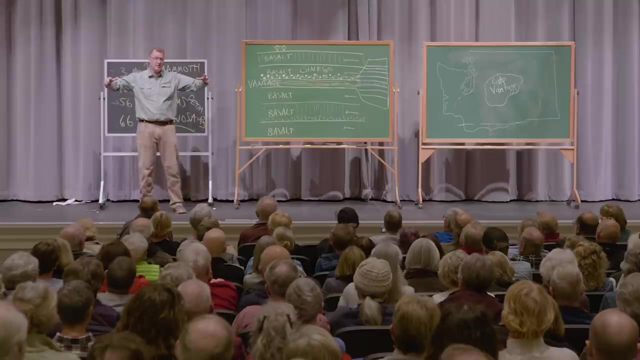 not Lake Lewis. These are not the slack water sediment beds. This is an older lake from the great flood basalt time And this lake probably existed because one of the earlier lavas blocked a bunch of rivers, maybe blocked the Columbia for a while and developed Lake Vantage. We need Lake. 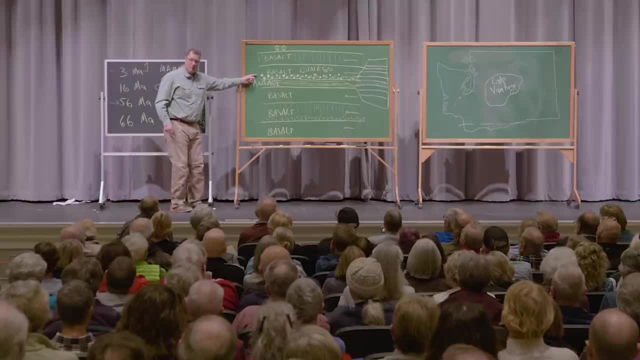 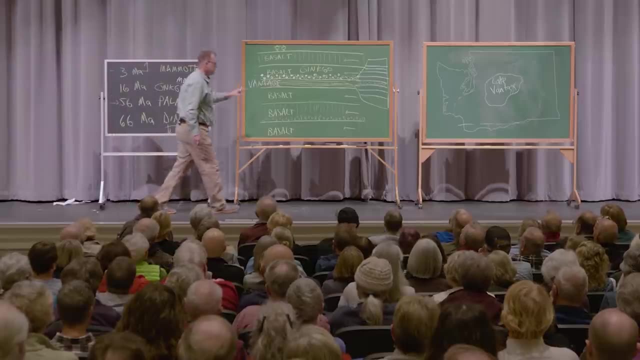 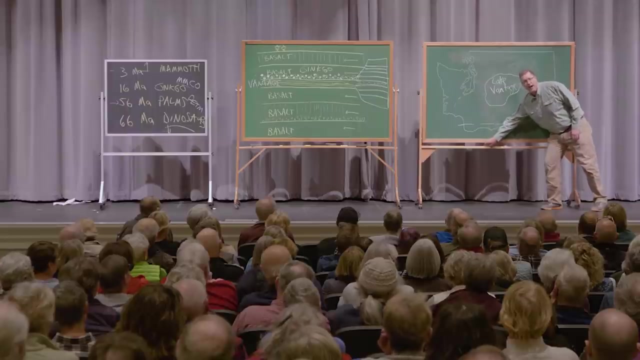 Vantage here Why We have pillows. When the Ginkgo flow comes in, it's going to plow right into this temporary freshwater lake called Lake Vantage. But you hear what I'm saying, I hope. Where are the logs coming from? The guy George Beck back in the 30s. 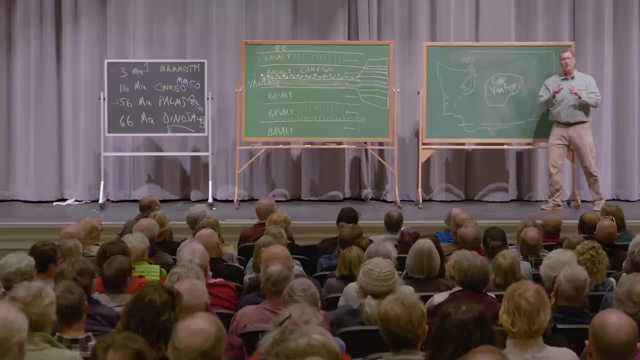 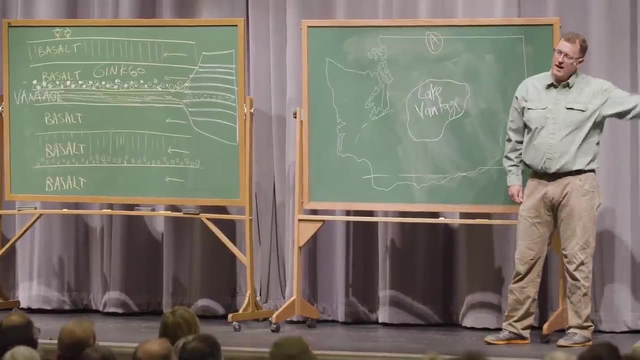 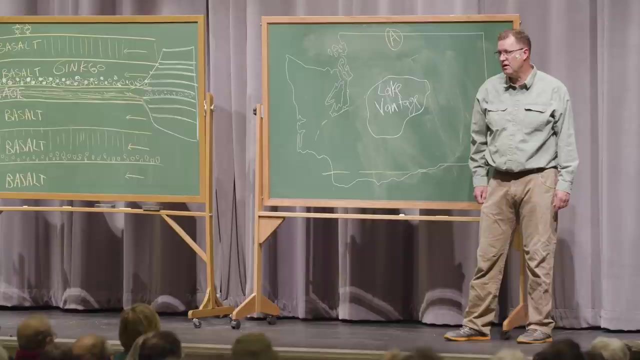 had a pet idea And most of his papers follows through on his idea. He thought all those logs that are petrified right here in Kittitas County are from the Okanagan and maybe some in British Columbia and that there were periodic floods, not ice age floods. 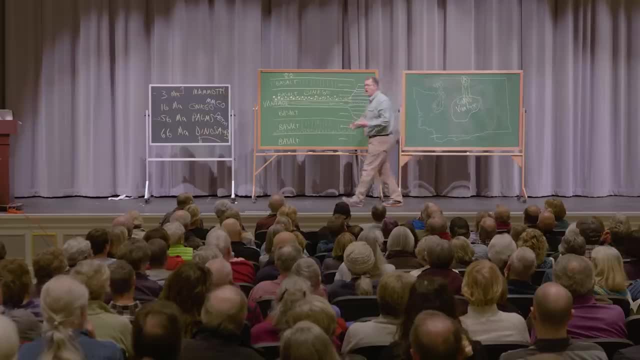 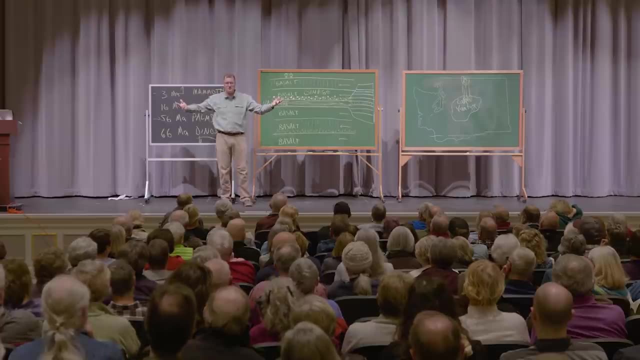 periodic floods, river floods, that would get a big old log. It's got to be a big flood. We're carrying huge logs. They're not petrified yet, by the way. They're now just tree trunks- living tree trunks, dead tree trunks. Let's carry them down to central Washington. 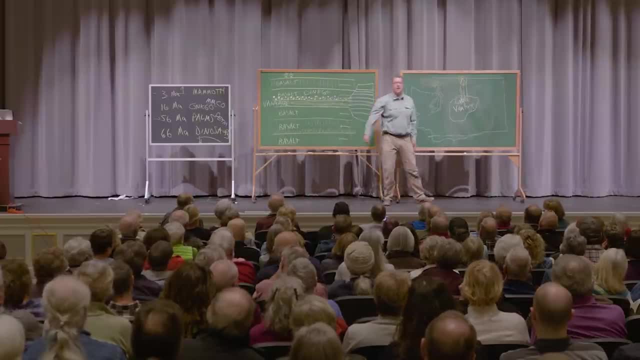 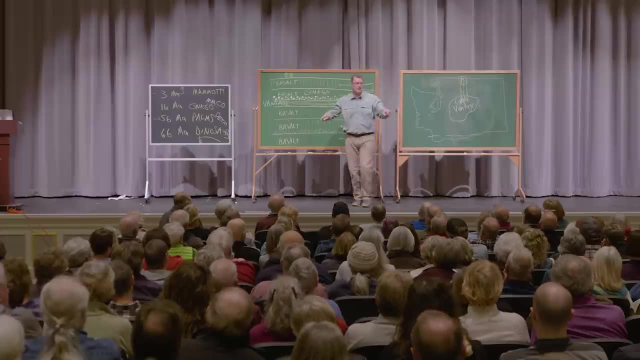 But Beck kept talking about this river of the north bringing all this material south and dumping those logs into Lake Vantage, kind of like today's Spirit Lake up by St Helens. All those dead logs have been there since 1980, floating, and some have sunk to the bottom maybe. 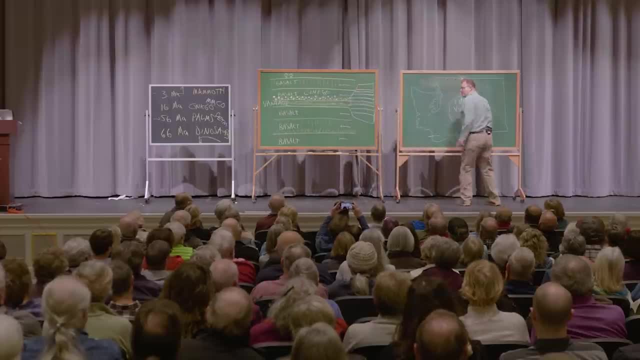 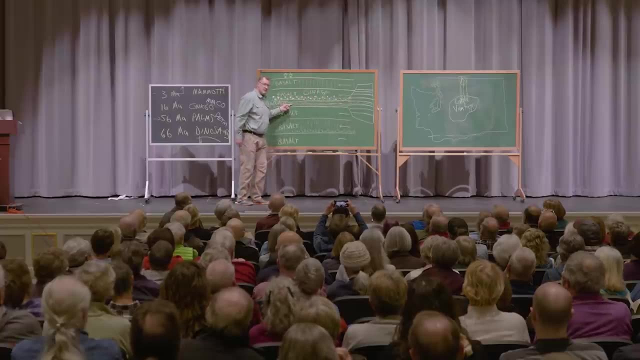 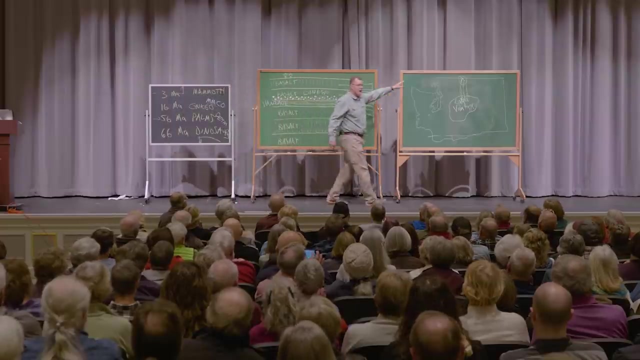 Same idea here. There is some geologic evidence for the logs coming from the north. Much of the sediment in the Vantage sediment has muscovite in it, And muscovite is a mineral that is common in rocks in the Okanagan and not common in southern. 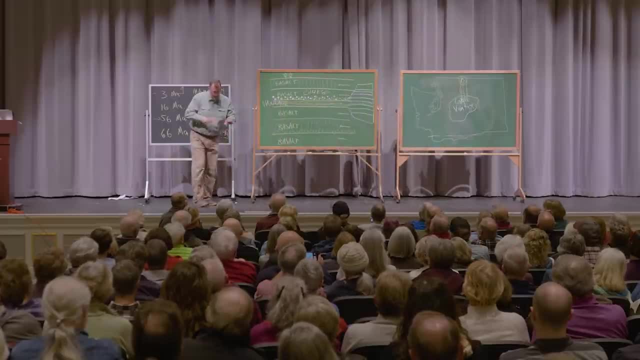 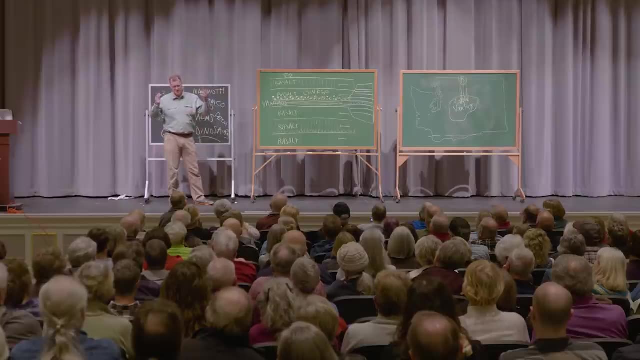 Washington. There's a couple other evidence as well. There's some paleocurrent indicators as well, But in the last 30, 40 years there's been a new idea, if you can call the last 30,, 40 years new. 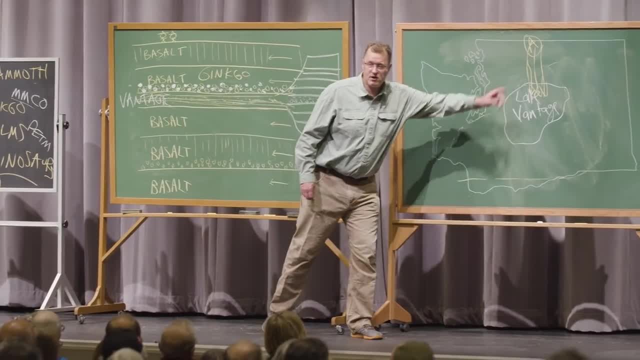 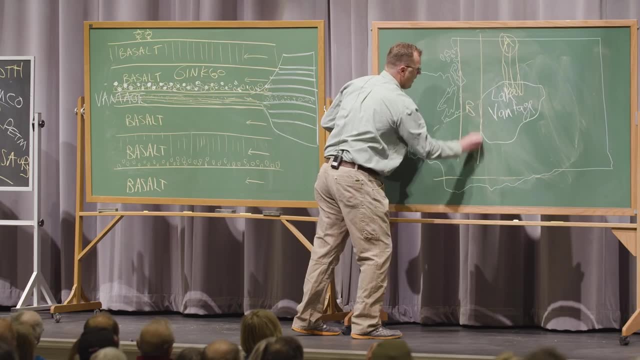 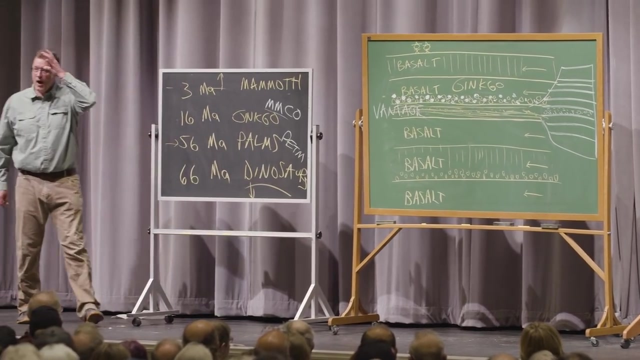 And you may have heard this one- Instead of Beck's Okanagan source for the logs. some geologists have said: why can't we have volcanic eruptions in the Cascades? We've got the Cascades now, We're 16 million years ago. Why can't we have a volcanic mudflow come out of the mountains, come out of? 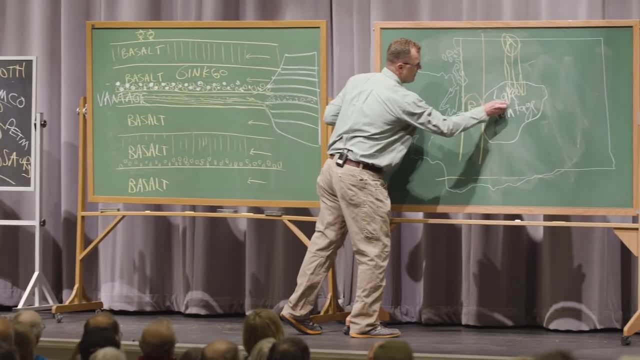 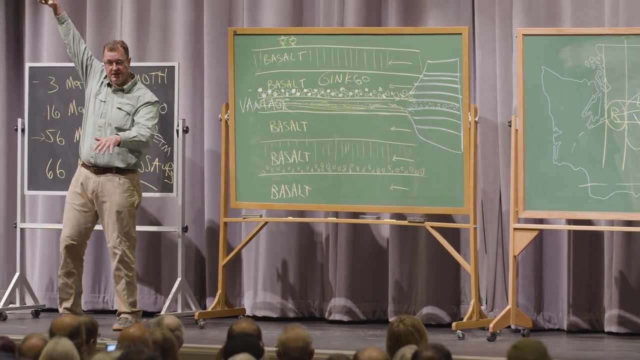 the Cascades and bring logs from the Cascades and dump them into Lake Washington. We can even have more elevation differences. Think of the elevation difference from the high Cascades down to here and all the different trees that we have at different elevations. 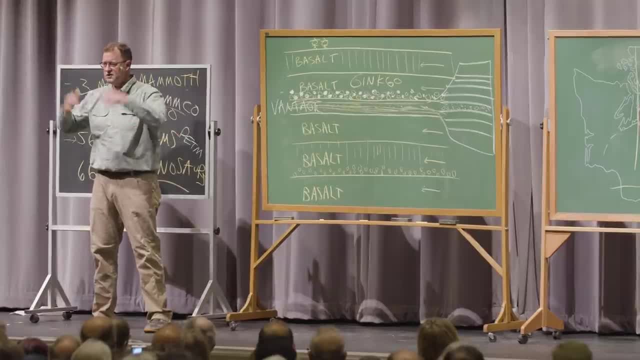 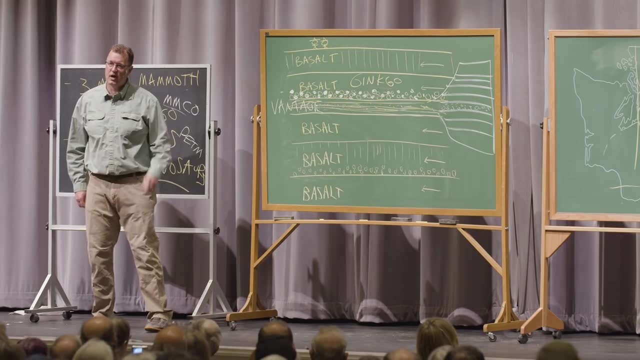 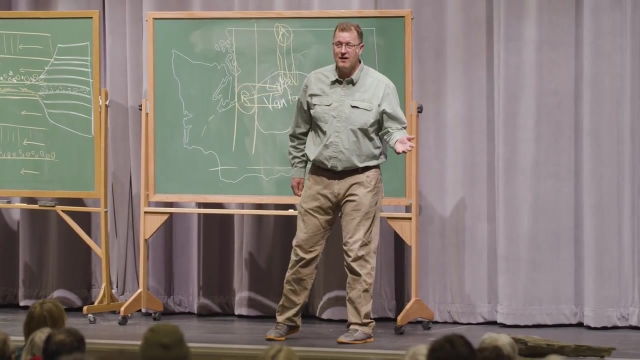 Can't we have a lahar, a volcanic mudflow, pick up a bunch of those trees at different elevations and bring them down and dump them in. So right now, those are the two competing ideas. Are they Okanagan logs or are they Cascade logs? Are they both or is it neither? That's where we are in the 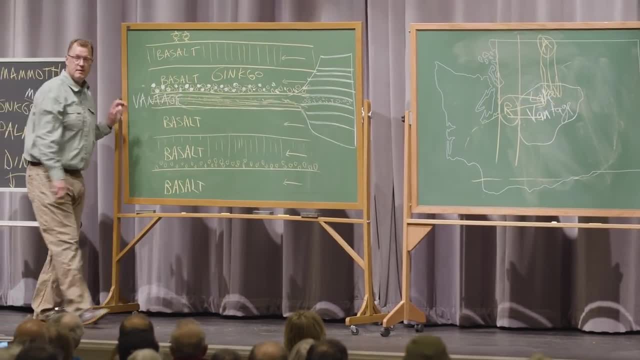 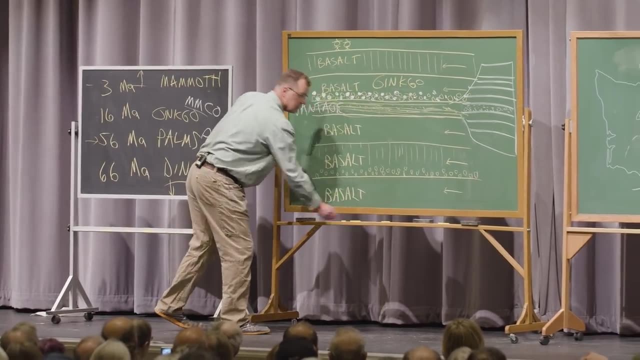 research, And so there's a lot of attention given to the vantage sediment, looking for clues of the Okanagan versus the Cascades, And then, of course, there's continued work with the logs themselves. This is the last thing I'll say. with the chalkboard, Some pumice has been found. 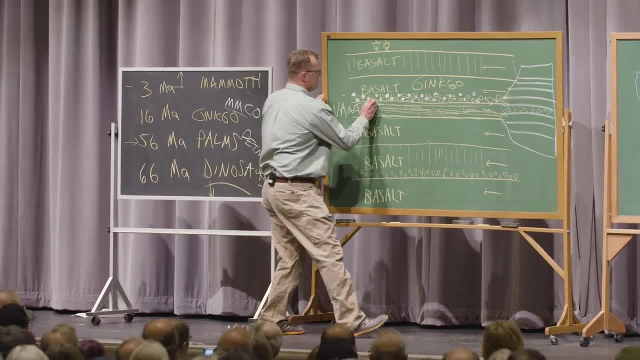 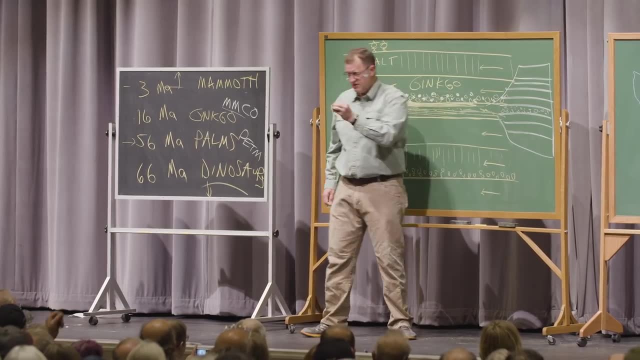 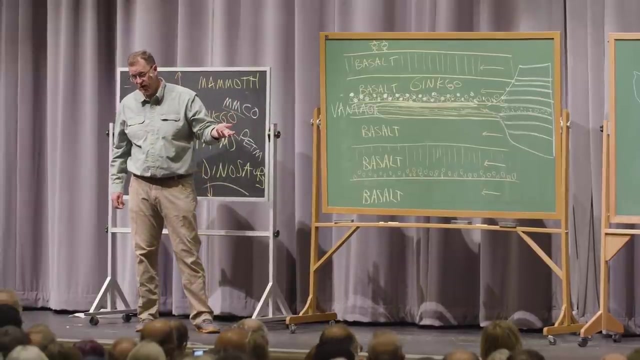 right at the base of the Ginkgo. So right beneath the logs, right at the top of the vented sediment, there's some pumice. That helps confirm that we have a Lahar story, that we have a Cascade story instead of an Okanagan story. But here's my biggest point. 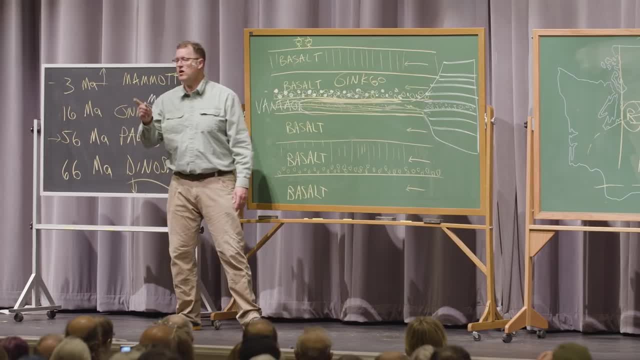 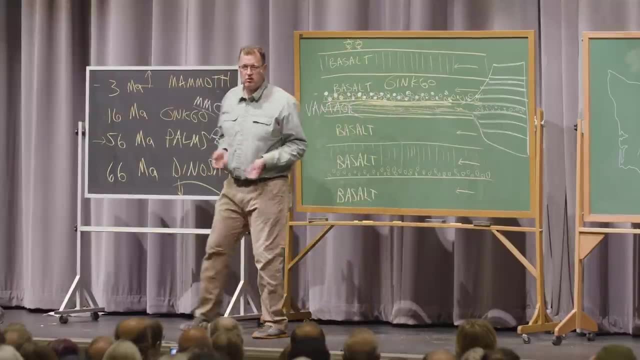 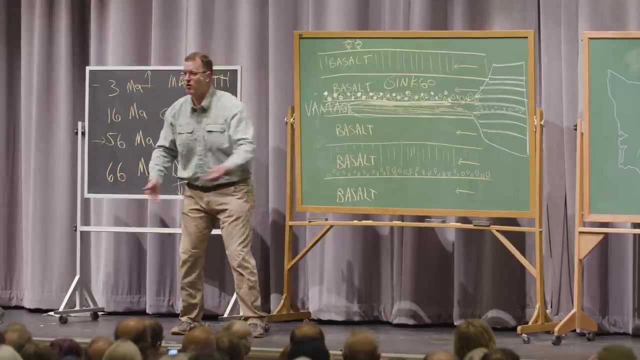 before we quit the chalkboards. There are no logs in the vented sediment itself. If the vented sediment is the quote-unquote key to unlocking this mystery, why don't we have a bunch of logs or woods or branches or acorns or anything in these 15 repetitive debris flow? 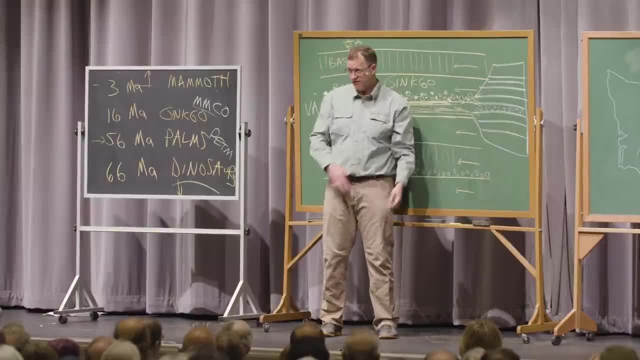 things. If you're a Cascade person, you want each of these to be distal parts of a Lahar. If you're an Okanagan person, you want each of these to be distal parts of a Lahar. If you're a Cascade person, you want these to be these river floods coming down, But there's no. 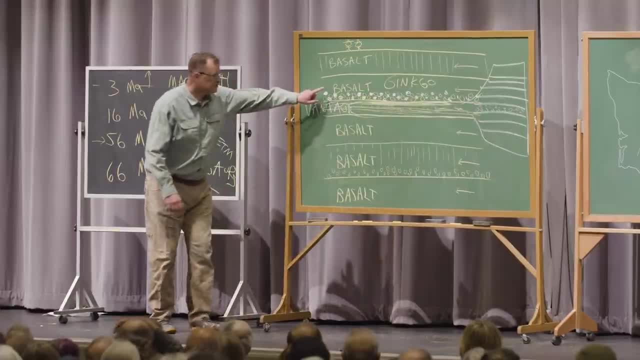 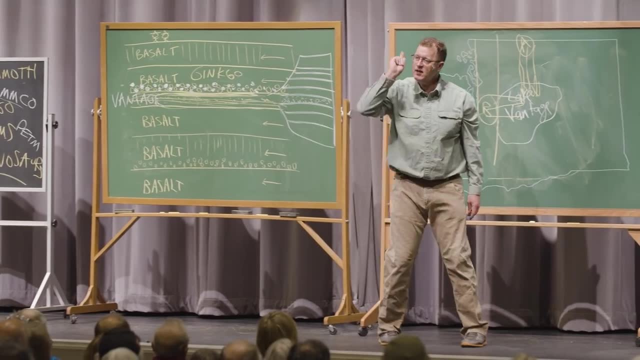 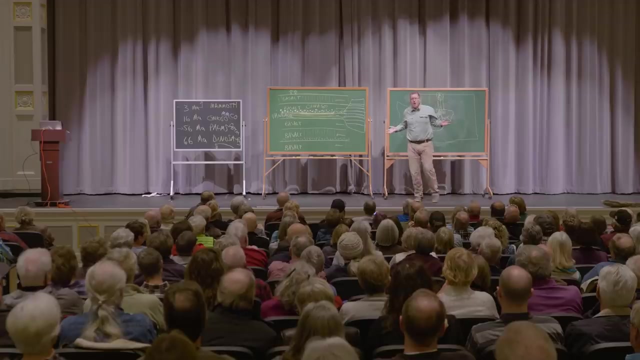 wood in this stuff. The wood, the logs are all up within the pillow zone. No roots, None of those trees were in place. Every log at vantage was moved. And from where Is this life and death? No, Are people's lives at stake? No, they're not, But it is a tantalizing mystery that continues to be. 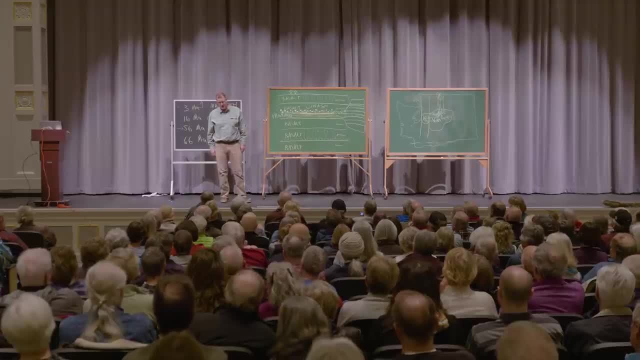 worked on by just a handful of paleontologists. This is the time of the night where you turn to your neighbor and say I love plant fossils with all of my heart And that will give us a chance to turn on the screen here. Thank you, I brought. 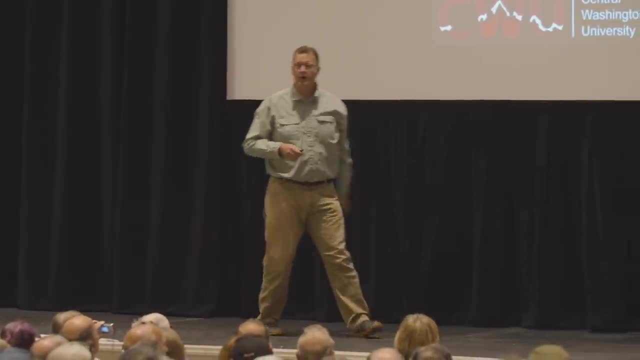 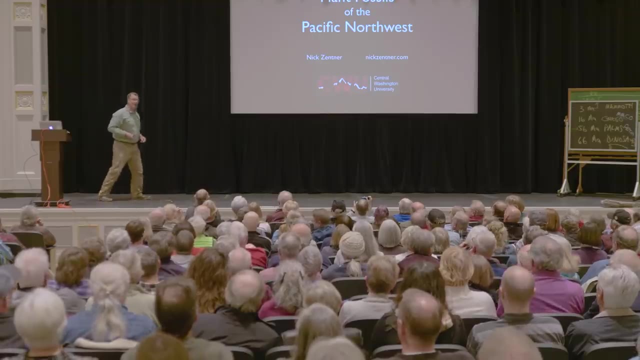 a plant fossil with me tonight and it's up here on the front. It's a beautiful palm frond, collected by George Beck himself, so I'd be happy to show this to you after the lecture. Let's go ahead and really sink in to all these visuals I have planned for you. That's a dinosaur. Where is it? That's an. 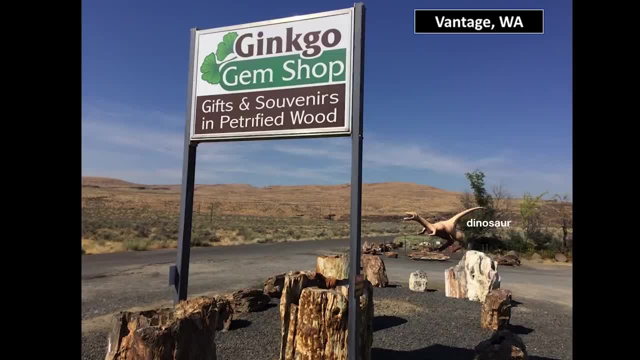 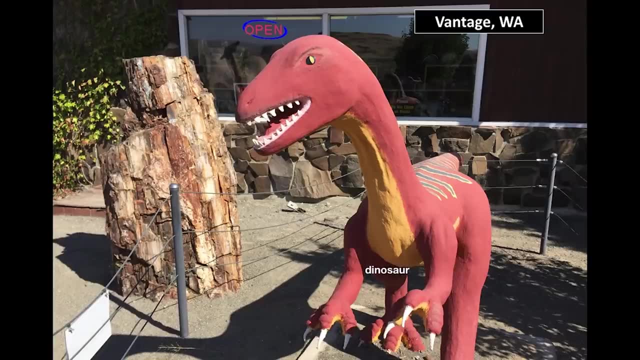 advantage. That's confusing. Oh, I guess if we're outside of the state park and we have our own little gem shop, we can do what we want. So we'll put a dinosaur that has nothing to do with ginkgo- petrified wood- next to ginkgo. 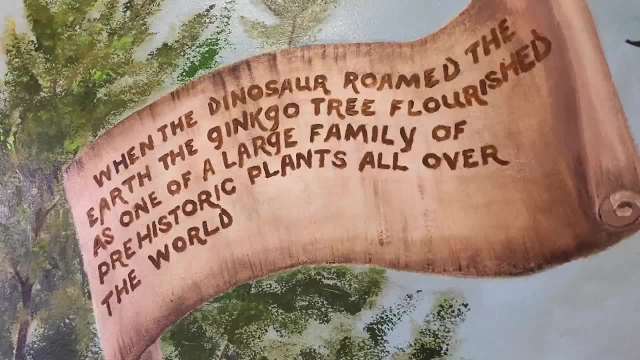 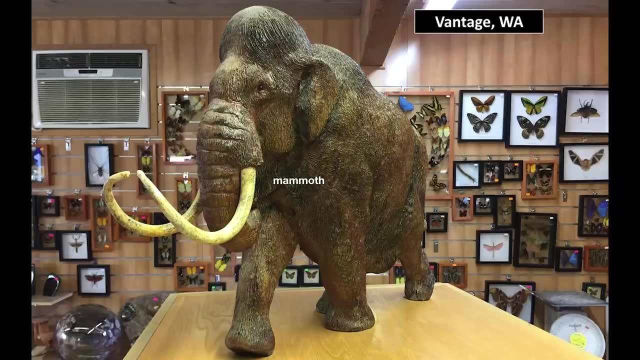 petrified wood And inside of the gem shop. when the dinosaurs roamed the earth, the ginkgo tree flourished as a large family of prehistoric plants all over the world. There it is. It's written, It must be true. We have a mammoth, Also confusing. This is all in the same place, Oh, but now we're. 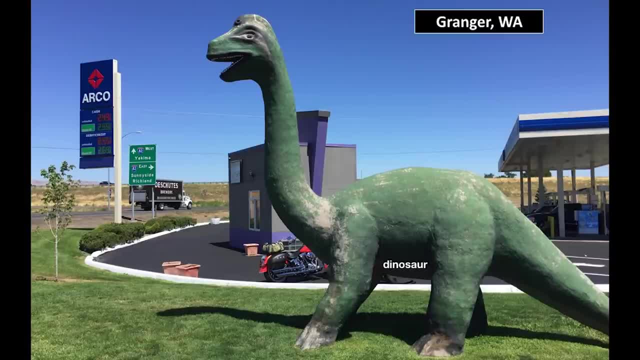 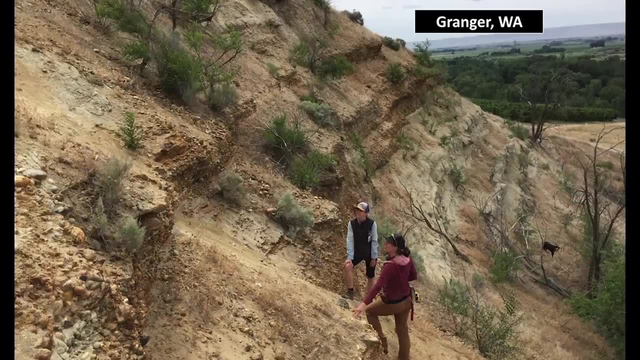 in Granger. Sure, We've got dinosaurs all over the place. We've got a dinosaur. We've got a mammoth All over the place in statue form. there's not one dinosaur bone down below. These are the beds at Granger that have produced mammoths, not dinosaurs. We know the difference now, Hopefully. 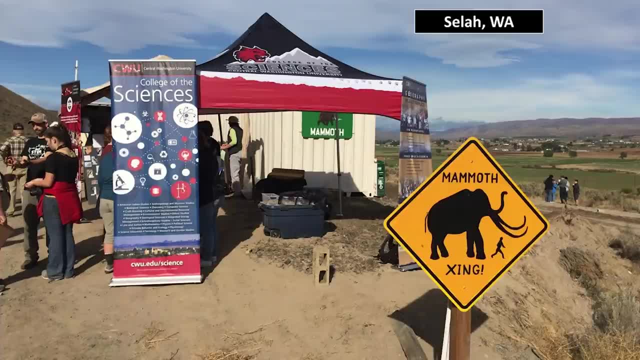 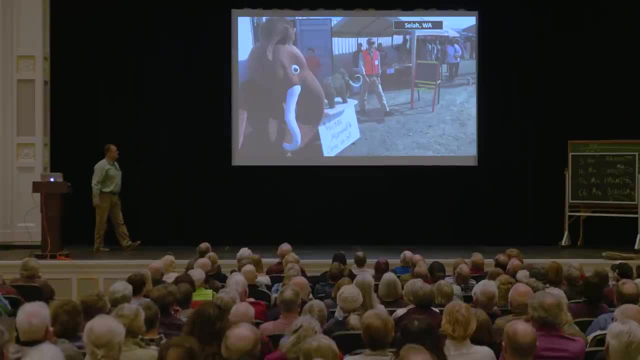 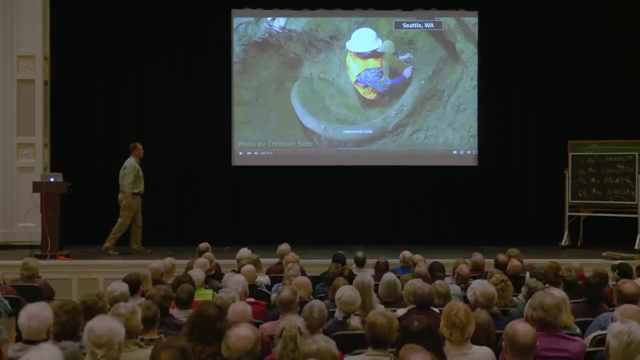 we can spread that word to others, But this is a mammoth site run by this school in town. Pat Lubinsky and others excavated a mammoth near Selah Washington And that is wrapping up now, but students have been actively participating in digging up parts of that mammoth at the WE-NAS. 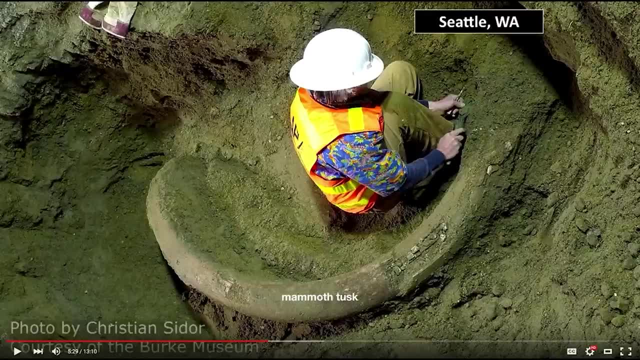 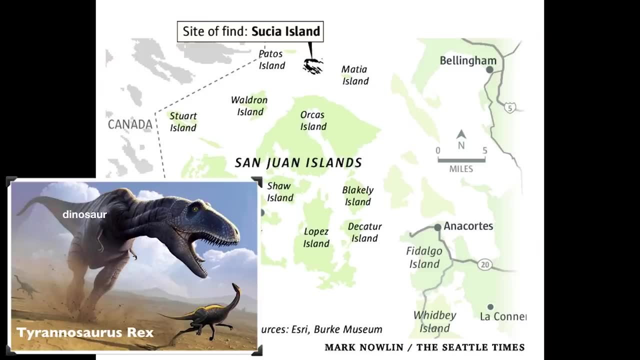 There's a tusk that was found in downtown Seattle. they were creating yet another block of Amazon buildings just a few summers ago. This truly is the only dinosaur that has yet been found in the state of Washington, in Sushia Island, San Juan. 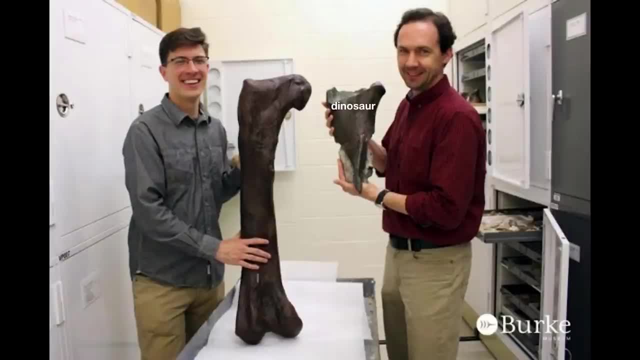 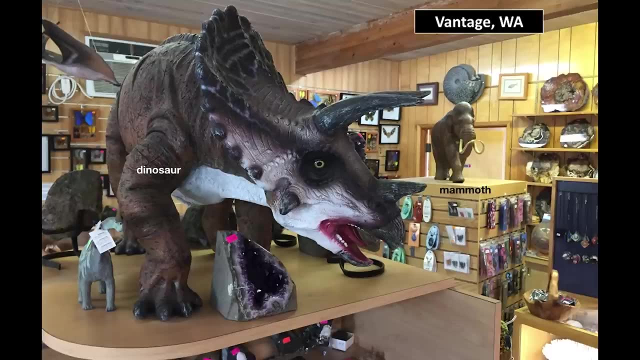 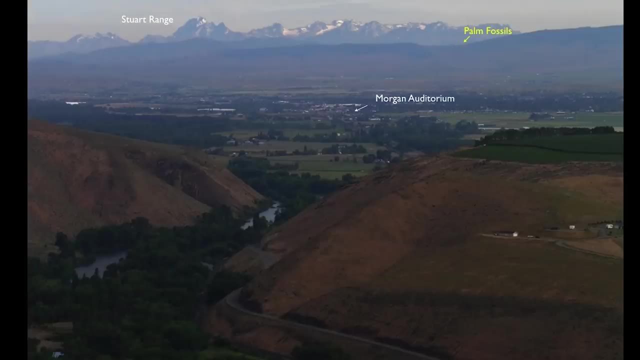 There's the fragment of the bone on the right and there's an appropriate-sized left femur of a Tyrannosaurus Rex. Dinosaurs and mammoths- not the same thing. That's not our topic tonight, but I feel better. Thank you for listening. So we are in the Morgan Auditorium. 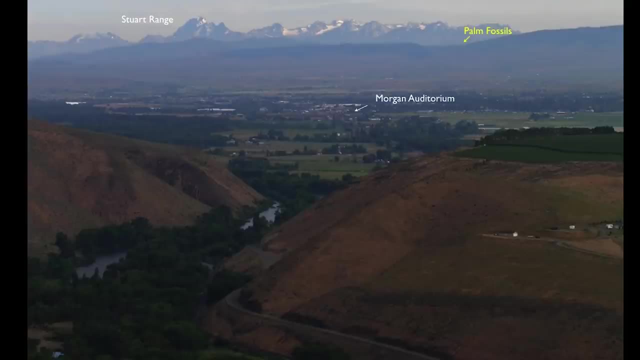 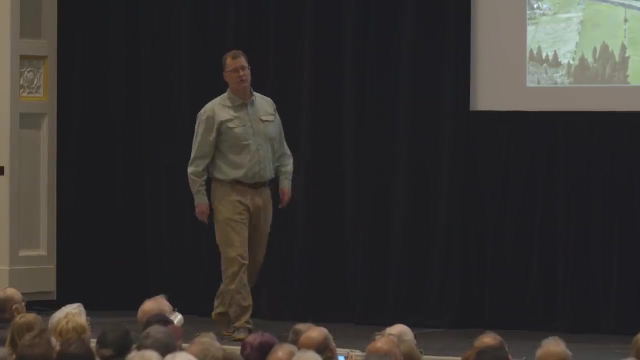 and I promised that if we headed north we'd head to the palm fronds. If we got to the Stuarts we'd gone too far. Same thing from Cle Elum. Cle Elum is 30 miles away. We could do the same thing. 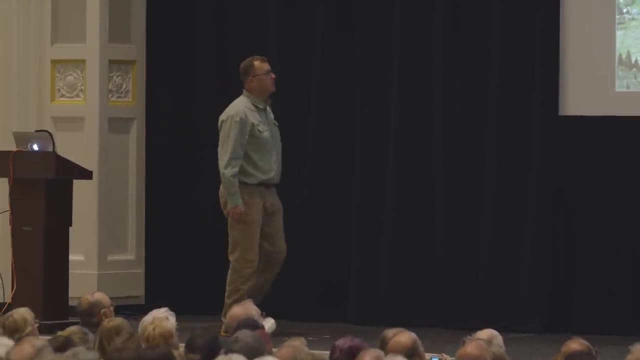 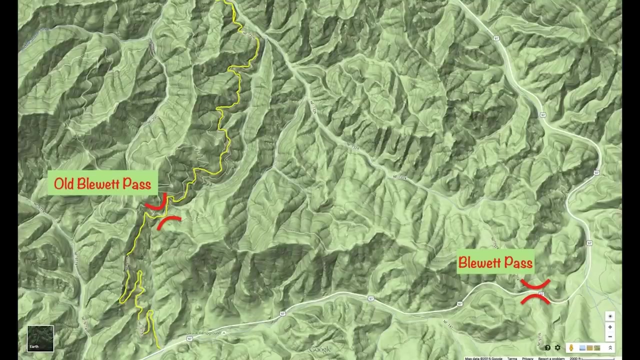 head north out of Cle Elum, head up past the Teanaway Community Forest and find the palm fossils. So up we go into those woods, into those dug firs and ponderosa pines, And one of the best places to look for palm fossils is on the old Blewett Highway, Blewett Pass, Most of us know. 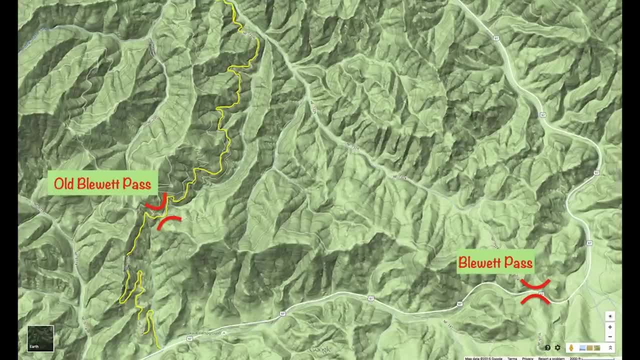 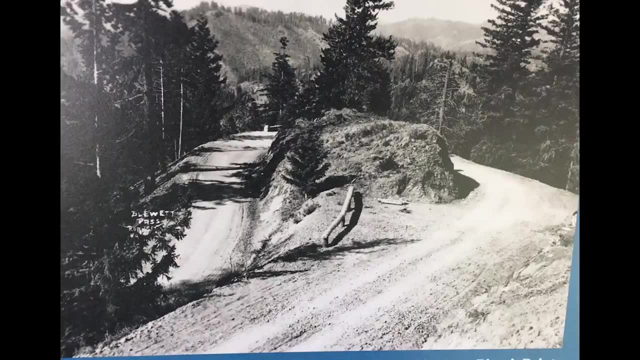 the area. but this is the new Blewett Road and it's difficult to stop. The traffic is loud, it's dangerous, but the old Blewett Road is still there And it was the main road between Seattle and Spokane back before the Depression. 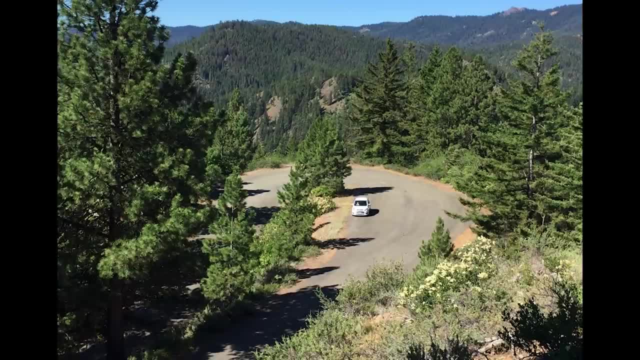 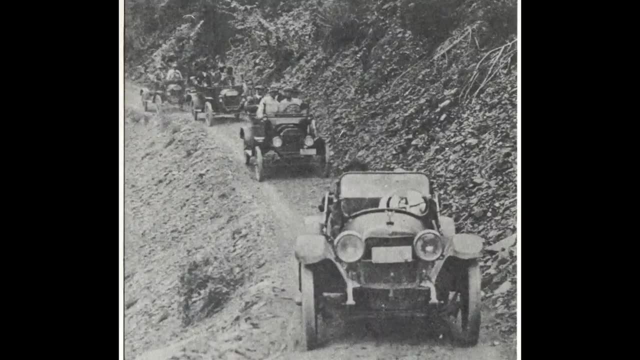 And that road is still there and it was last paved in the 1950s And, starting in 1956, all the traffic was sent over to new Blewett, And so it is truly a pleasant experience to be on this old road. Here's the old Model Ts. back in the Depression They would back up as they approached. 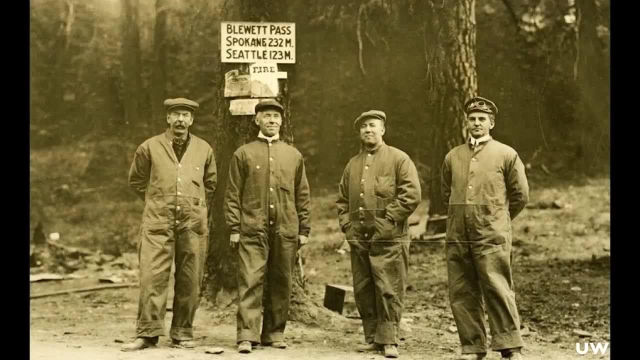 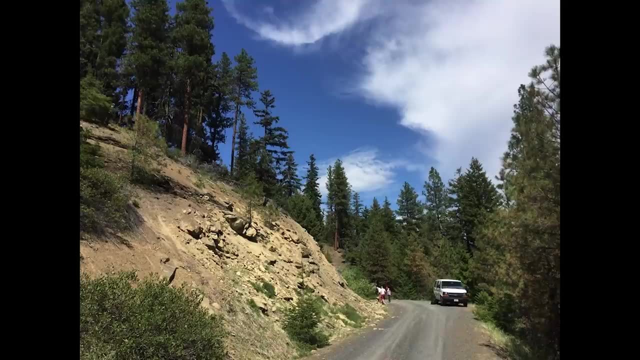 the steepest part of Blewett Pass And it was a landmark for many cross-state travelers before the 1930s. So it's a great place to study, to find, to discover and to explore. And it's a great place to study, to find, to discover and to discover. 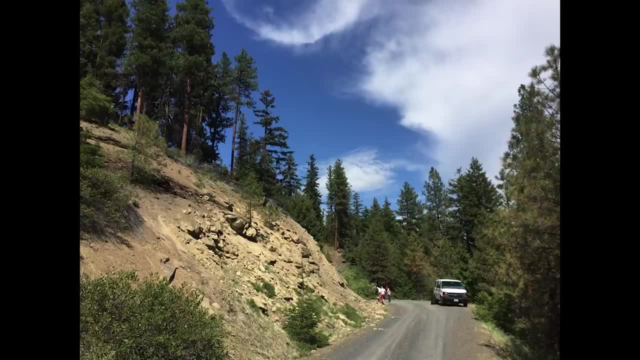 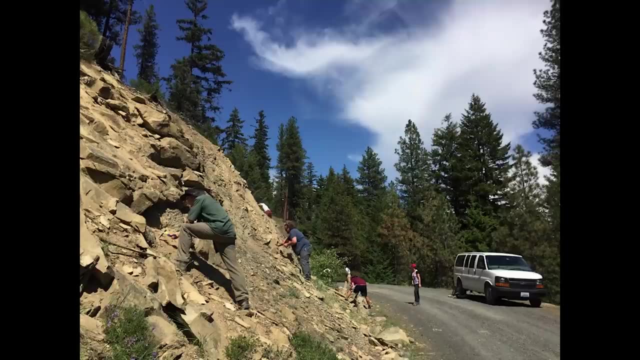 And it's all for free. You can park right in the middle of the road. You won't see anybody on a beautiful Sunday afternoon. I encourage you, if you haven't been up there, to look around. What are these layers? This is 56 Hot. This is the sandstones and shales with the palm fawns and other kinds. 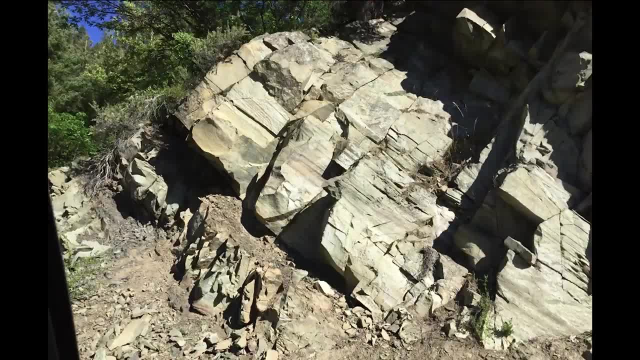 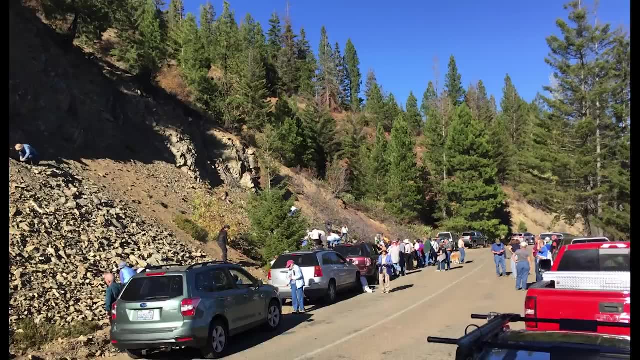 of plant fossils from that global warm time. Oh my God, are there any plant fossils left? Look, you got huge groups that are up there. I haven't taken them all. There's still plenty to look for. Many of you have been up there. 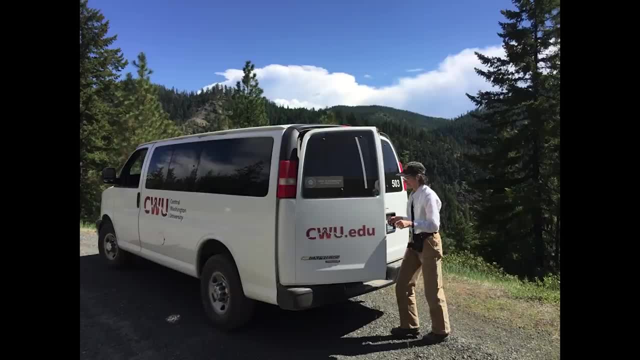 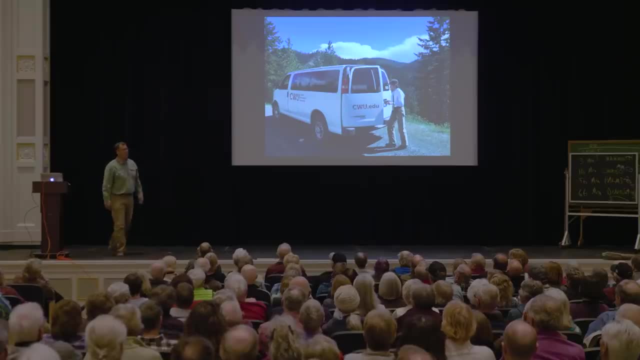 Hunting over the years And there's an unlimited supply- Wonderful. We've taken school groups up there as well And there's a long history of Central Washington University geology taking people to study and to collect. More about that coming in a bit. So this is a typical slab of 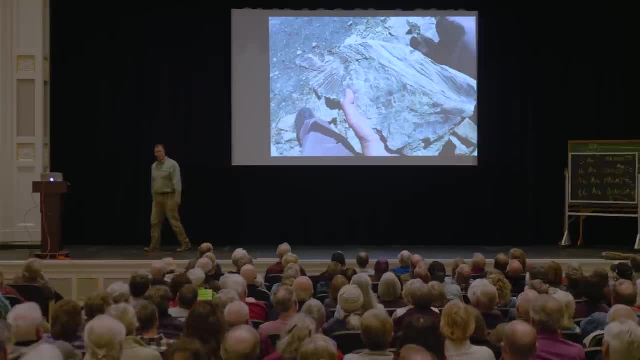 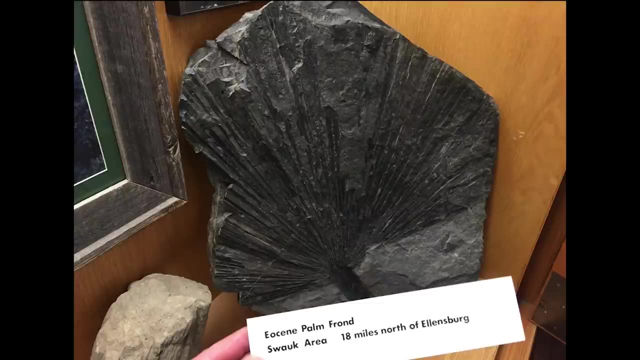 sandstone and or shale from the Swack Formation, And you can see what appear to be little fragments of palm leaves. And that is true, The fragments are there, But some of the beauties have been collected- This collected by George Beck himself, And I'm going to show you a little bit of a 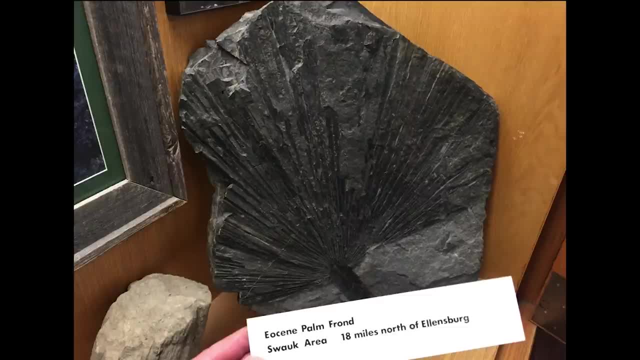 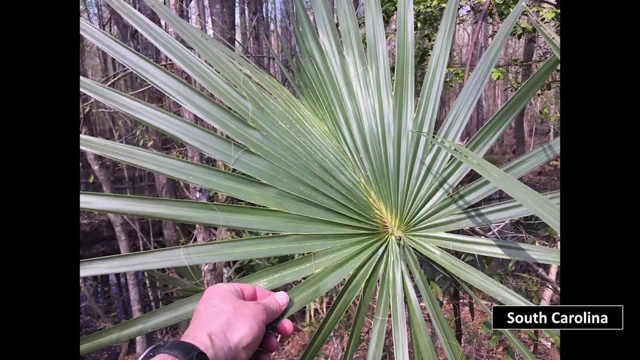 picture of myself in a display case that's right next to my office. I walk by this every day for the last 30 years And I'm eventually about to give a talk. Hey, it turns out I was on spring break with my wife a couple weeks ago. We just happened to go to Charleston, South Carolina. We just happened. 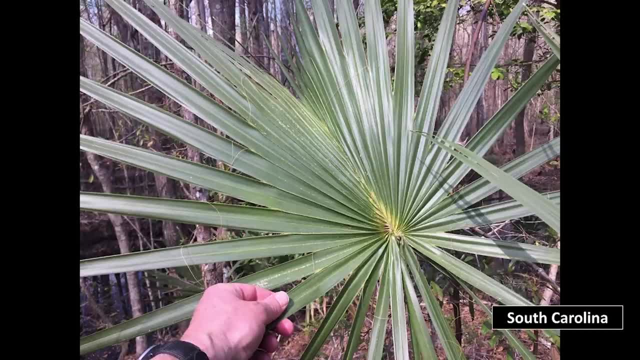 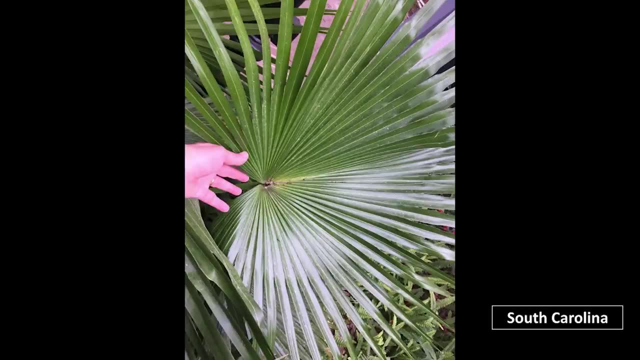 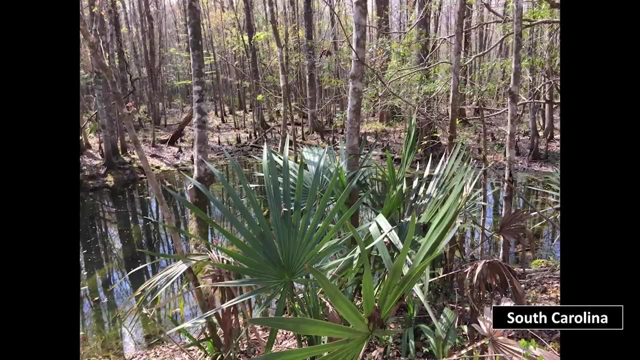 to be taking a little walk in the swamp. What a coincidence, Crazy. So they're beautiful, modern, analog to what Central Washington was like: The coastal plains and the hot, humid conditions with trees allowing us to have these amazing forests with swamps and cypress and alligators, and 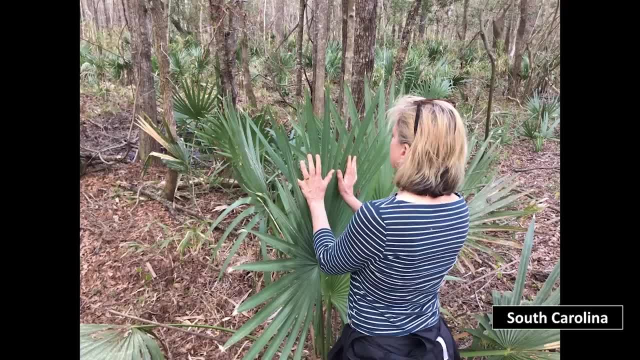 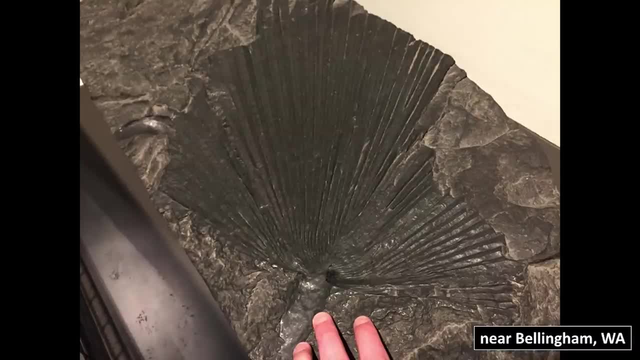 palmettos, Palmettos, a woman for scale, Back to the paleo, back to the 56 hot shales and sandstones. Now, if we're over by Bellingham, same beds, but they call it the Chuckanut Formation over there. 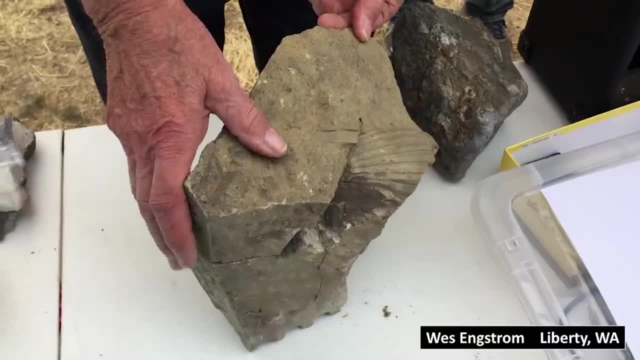 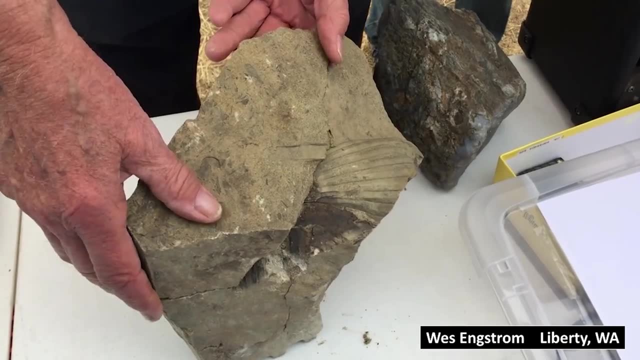 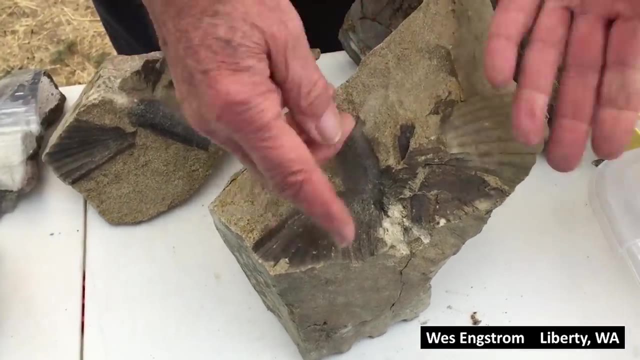 So West Angstrom, From Liberty Washington last summer I said when I found this on the surface, this part was showing And I just started hammering on it And luckily hammered in the right spot so that it opened up into a three-dimensional fossil. It just chipped a little bit off there, West Angstrom. 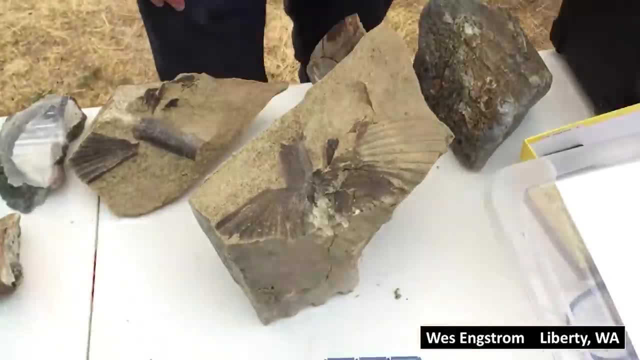 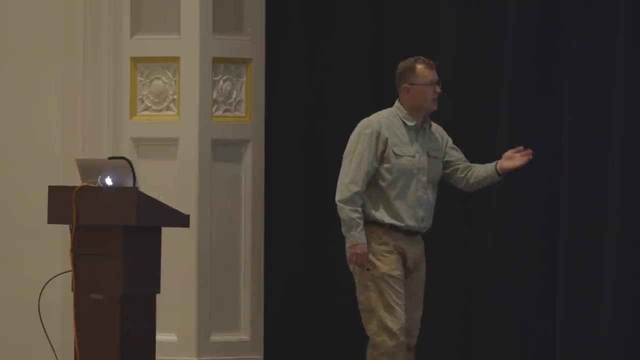 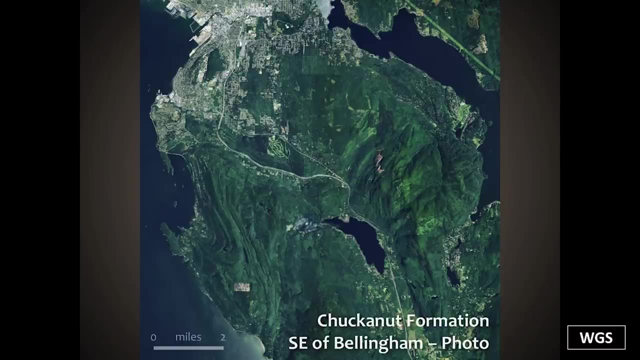 Fossil hunting, among other things. So more displays, impressions of palm tree trunks and other leaves from this walk near Liberty. Now if we hop over to northwestern Washington in the Bellingham area, it's a bunch of trees, it's a. 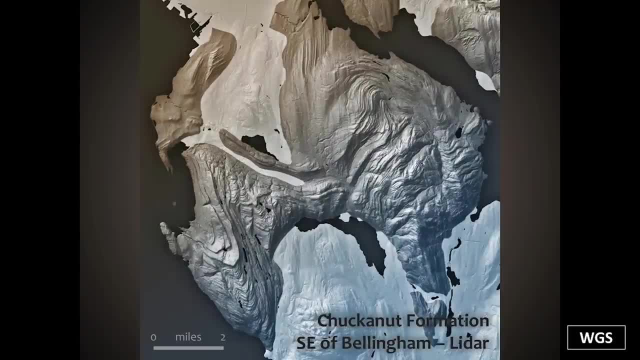 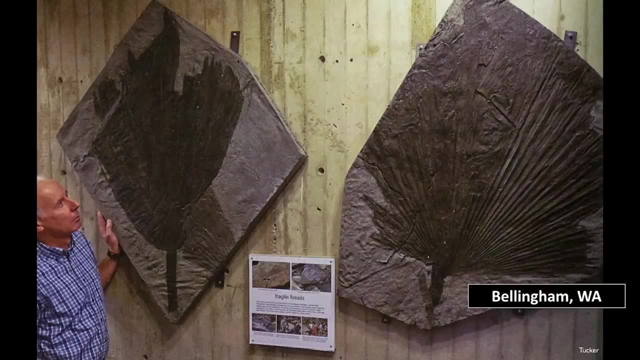 bunch of precipitation, but if we use lidar we can actually see those beds of sandstone and shale that are complexly folded but yet they reveal amazing palm leaves. Same time, 56 hot. This is in the geology department at Western Washington University. 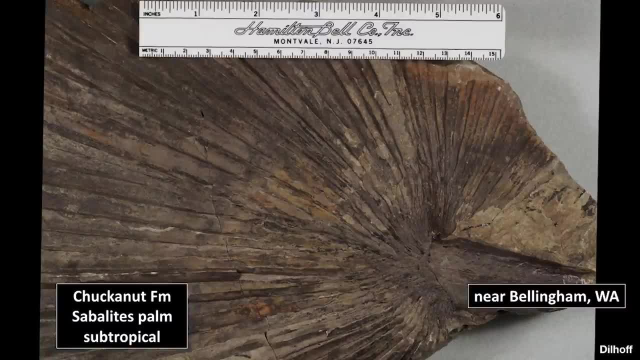 And these are just the beginning of these wonderful professional photographs from Tad Dilhoff, who's at the Burke Museum in Seattle. He has been especially helpful putting this lecture together. So thank you to Tad Dilhoff for these wonderful photographs. And last year, 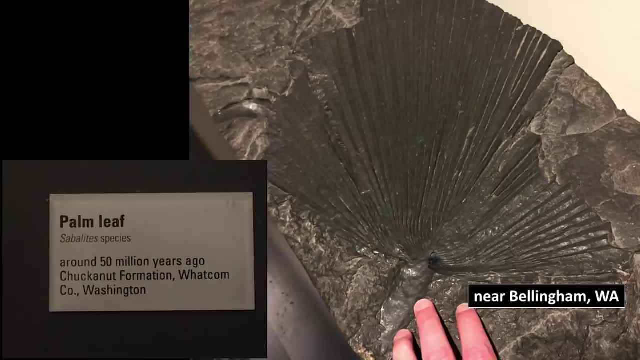 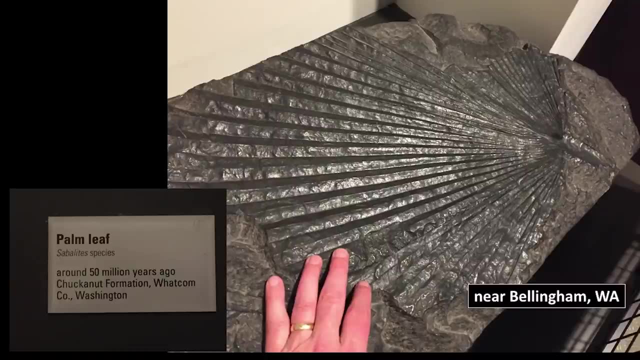 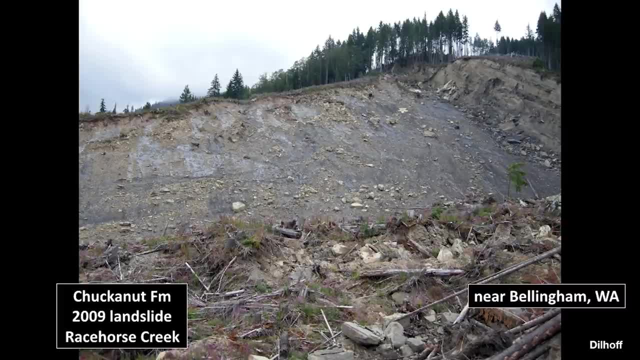 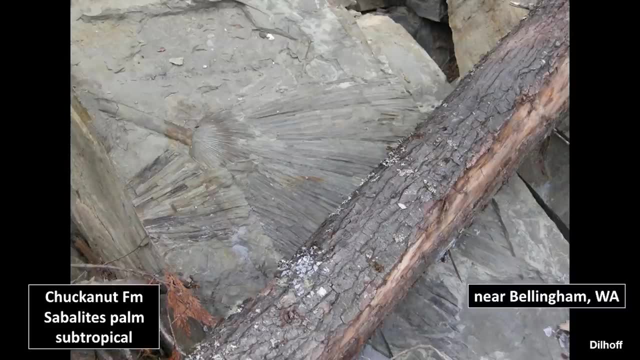 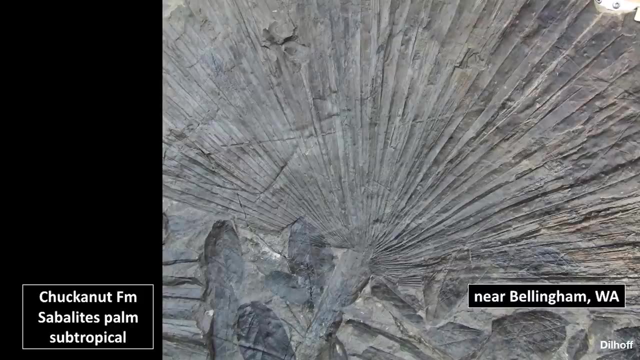 a big landslide in the foothills of Mount Baker And, in addition to the landslide being interesting, it revealed a whole new crop of amazing palm fossils in Whatcom County. Look at those beauties. We're focusing on the palm leaves, but you should know that there's a lot of exotic. 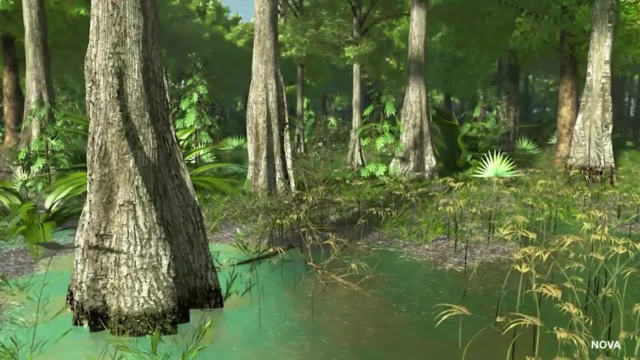 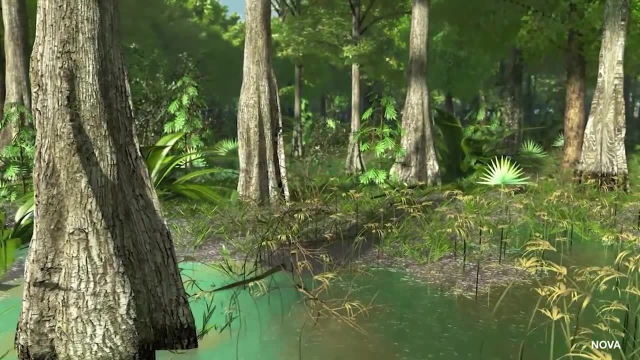 leaf types from that former swamp at 56 million years ago. So I grabbed this off the internet before we went to Charleston a couple weeks ago trying to get an assimilation of the palm leaves and the palm meadows and the cypress and the swamps and 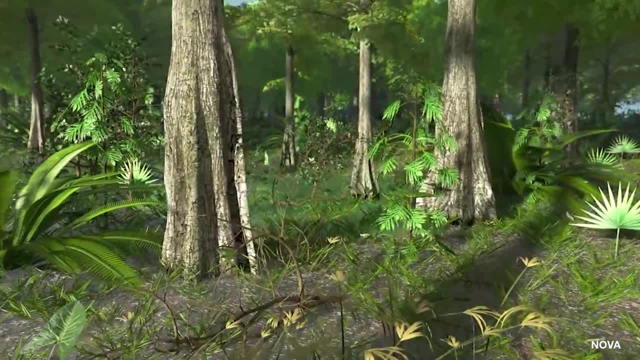 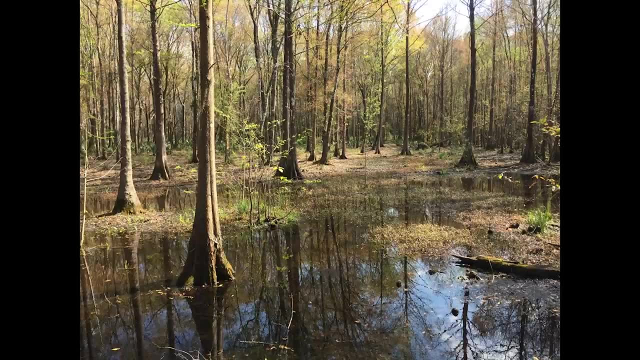 thought: well, that'll be good for the lecture. That'll give us at least a rough idea for what it looked like here during the Eocene time in central Washington. And then here's our hike two weeks ago in the swamps of South Carolina. Looks exactly like that, complete with palm. meadows and dense mats of those palm leaves that have died and have been added to the swamp floor- Amazing stuff. So the Carolinas or the Everglades in Florida is really what we want to think about for hot and humid conditions here in central Washington. Back to Washington today. 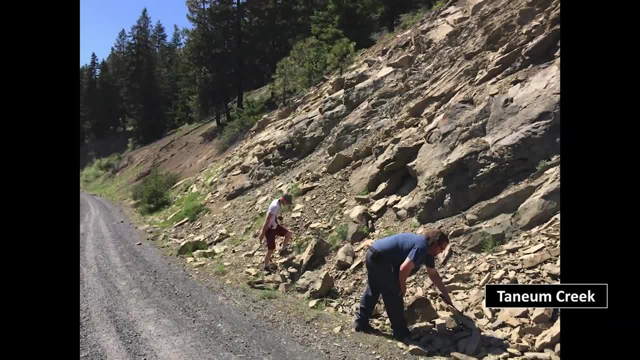 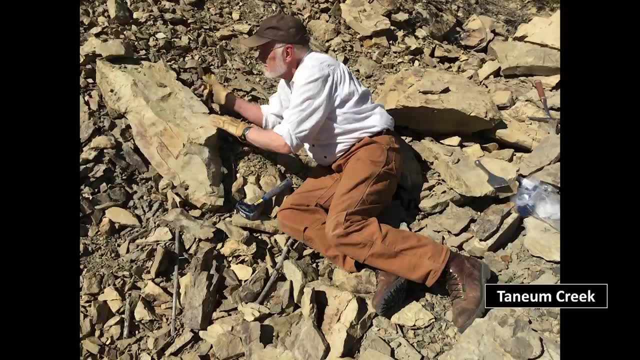 in addition to Blewett Pass. many of us know we can go up to Tainham, to the west of Ellensburg, and get those same beds and those same palm fronds pretty easily. So if you've got a young family, you've got kids who have limited attention spans. 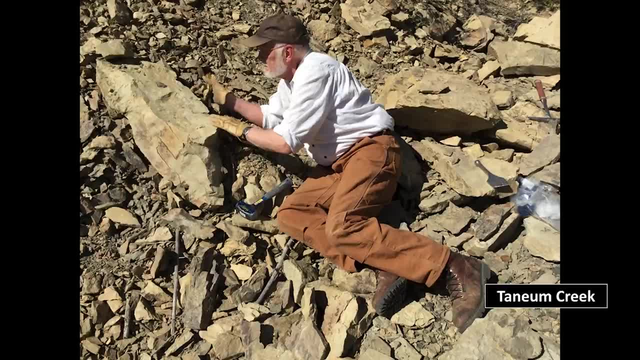 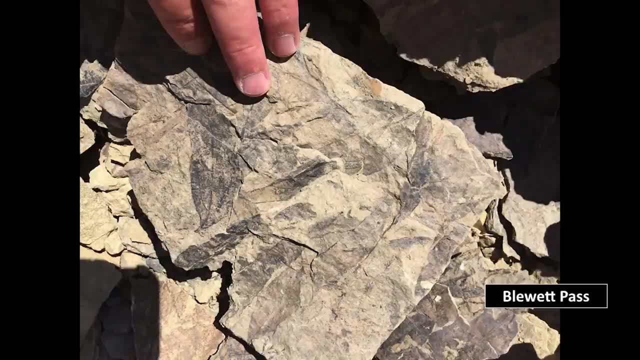 I promise that if we can get to the right spot- and I'll send you some directions if you're interested- you can get to a place where, within 10 minutes, you can easily find stuff like this, Oftentimes fragments of things. Of course it's not the huge palm fronds, That's. 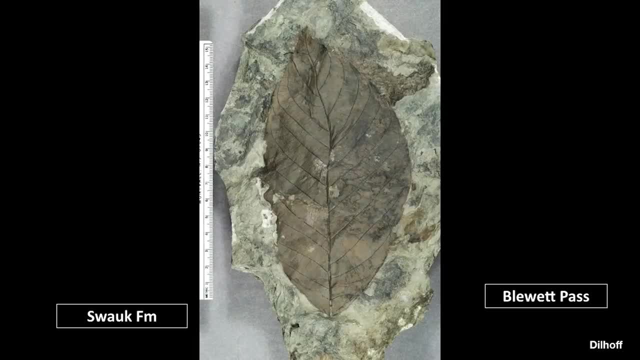 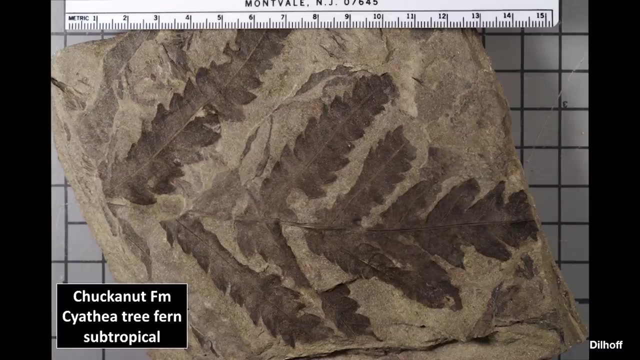 more difficult to find, but there's definitely palm leaves and other kinds of leaf fossils within an hour's drive of here, free and available for all. It's good, wholesome, clean, fun, All right. I think we've had enough of 56 Hot, at least locally. Let's expand our view. 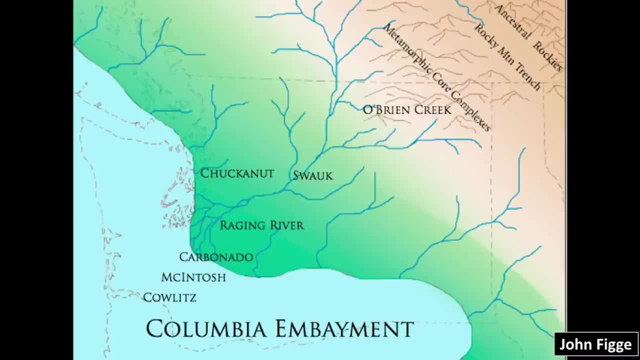 Because it is a global story. Remember this thermal maximum time. Actually, before we do that, this is a wonderful map I've used a lot by John Figge, who teaches geology in Seattle. This is Washington during 56 Hot. There are no cascades. The west coast of Washington is at I-5. 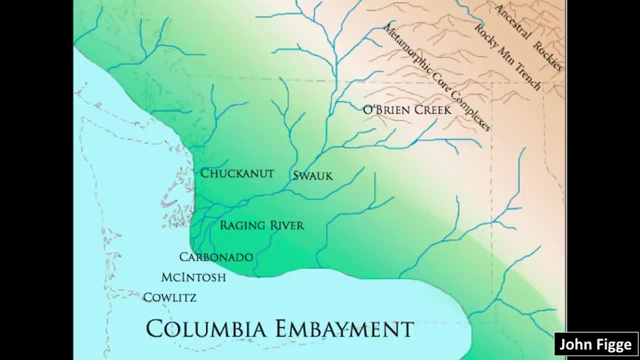 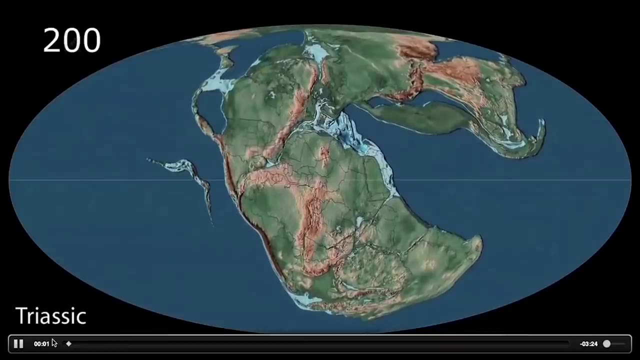 There's a south coast of Washington running through Granger, where the dinosaurs live. No, no, no, they don't, they don't, And we've got these poorly drained swamps and rivers coming from the northeast. Now to bust that myth so I can drive this global animation. 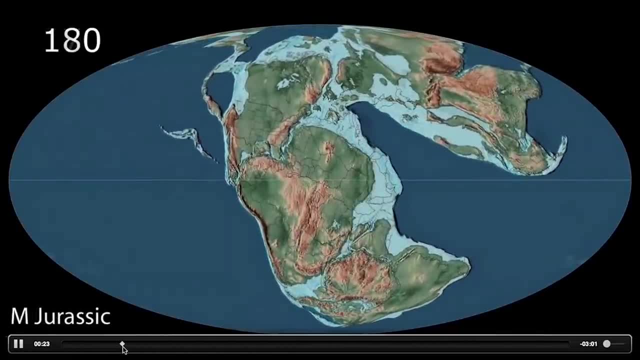 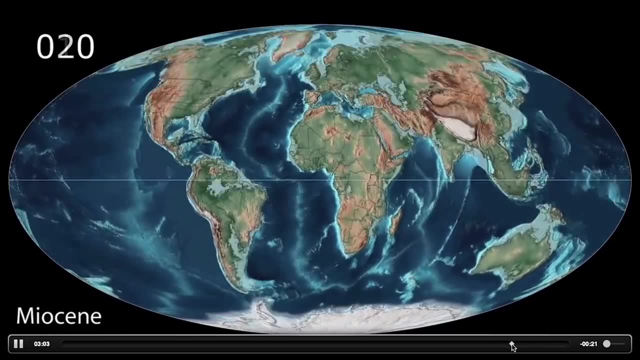 and let's keep our eye on North America. You know, like I'm not sure where North America is yet. Well, let me go way ahead. Now you got North America. Let's go back in time. Let's go back in time. 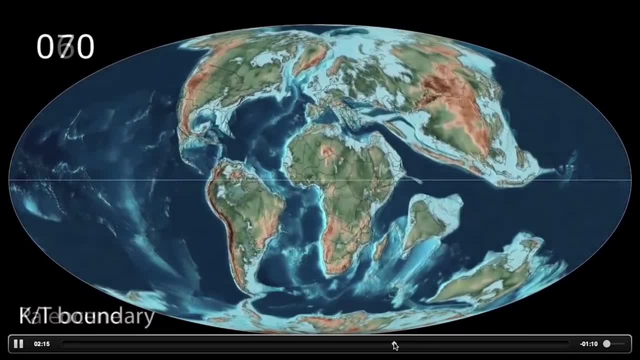 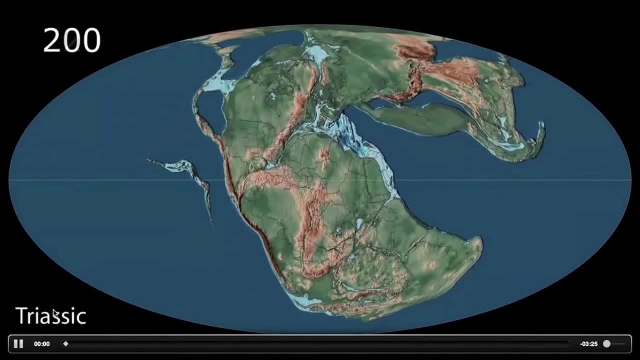 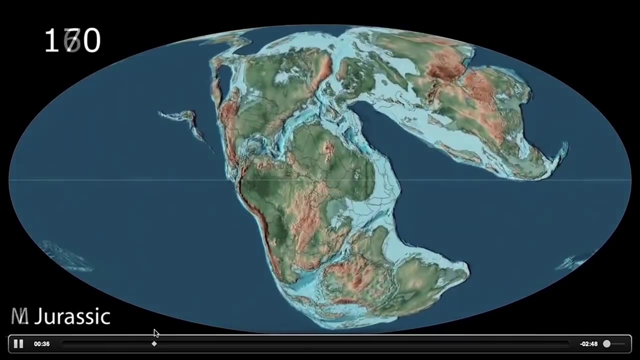 There's North America 56 million years ago. Now, can we get North America to the equator? Well, we can, but if only go back close to Pangea time. So is it true that Washington, 56 million years ago, was at the equator? It was not. This is not an idea. These are carefully reconstructed. 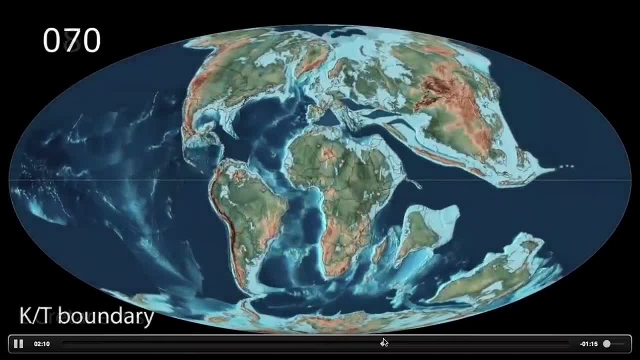 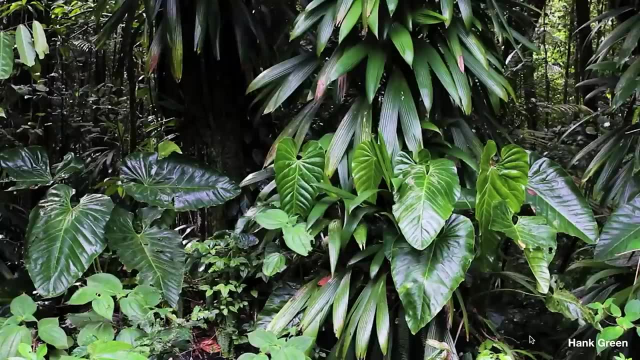 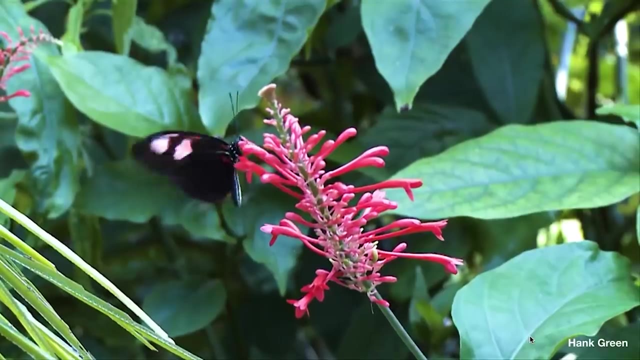 maps to show that we were further north 56 million years ago than we are now. Wonderful, So let's learn more about the PTEM, otherwise known as 56 Hot. according to me, This is a map of North America. It's a map of the Arctic. It's a map of the Arctic. 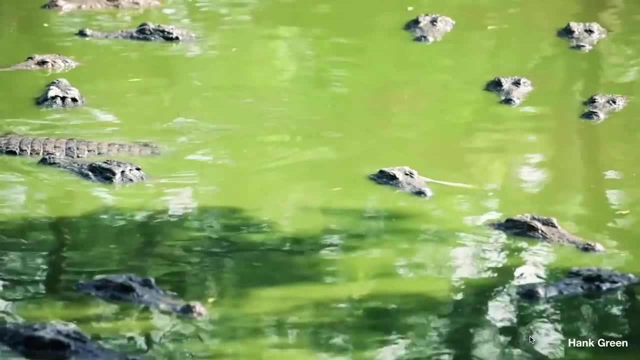 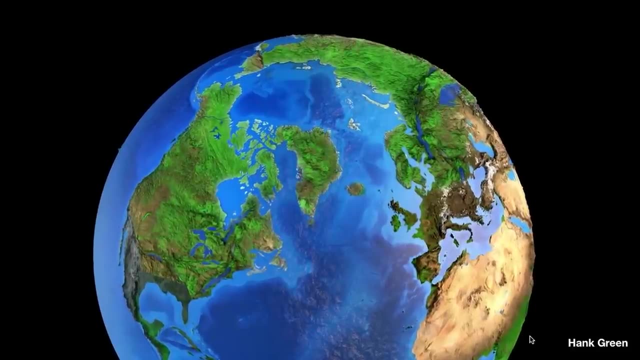 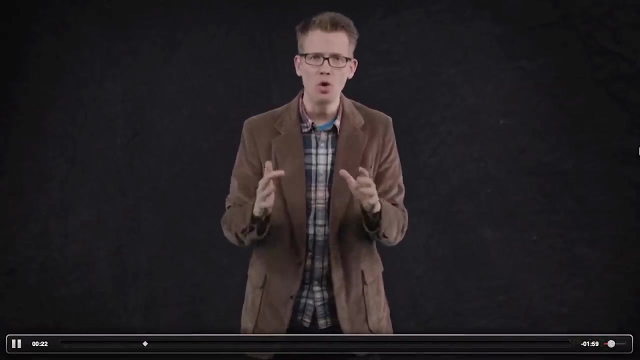 Primates are climbing up in the canopy while crocodiles and turtles swim in the rivers below. Beautiful, isn't it? Now imagine this lush rainforest in the Arctic. There was a time, not too long ago, when the world warmed more than any human has ever seen. 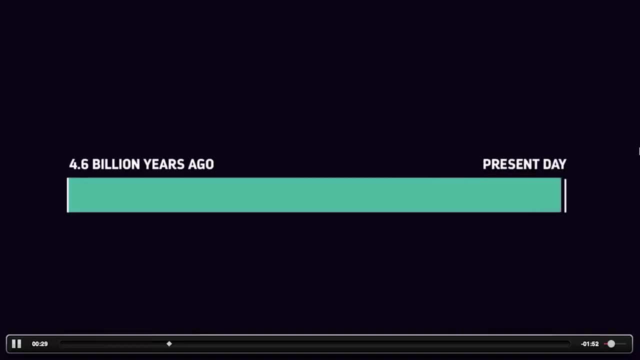 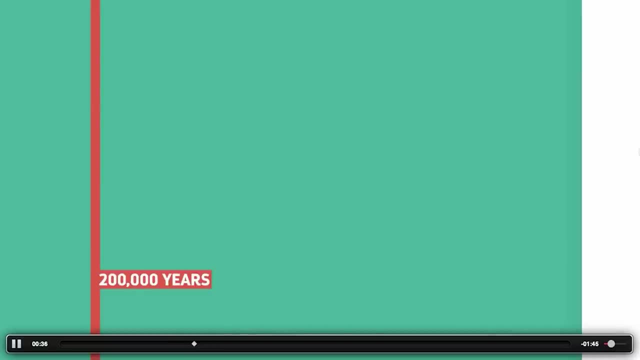 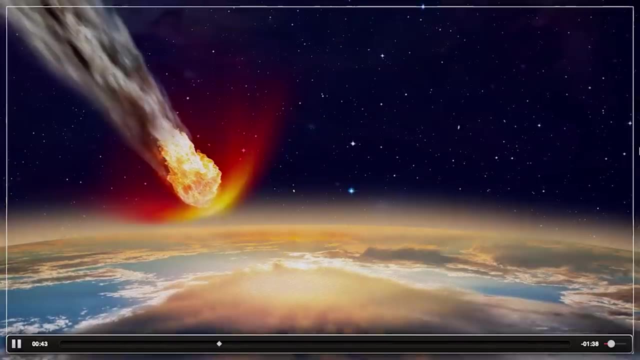 So far, This ancient warming took place over the course of just 200,000 years. The blink of an eye and it ended much like it began, suddenly and mysteriously. It all started 56 million years ago, at the very end of the Paleocene Epoch. Back then, life was still recovering from all. 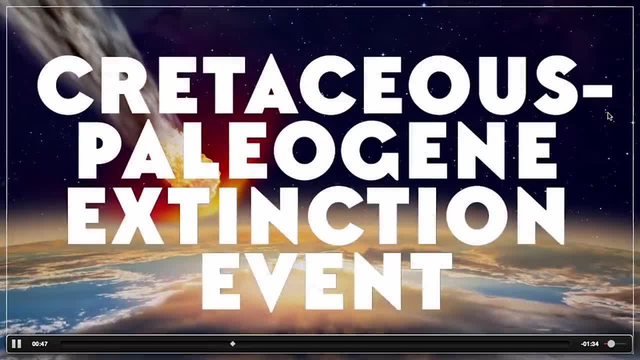 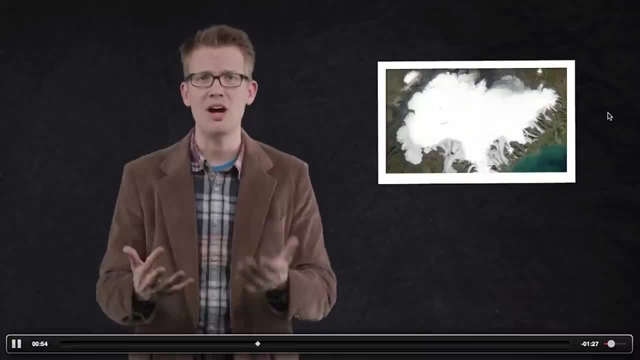 the unpleasantness of the Cretaceous-Paleogene extinction event, which wiped out the non-avian dinosaurs, And things were already warm by today's standards. There were no polar ice caps, which meant sea levels were much higher And the continents which were just beginning to take a 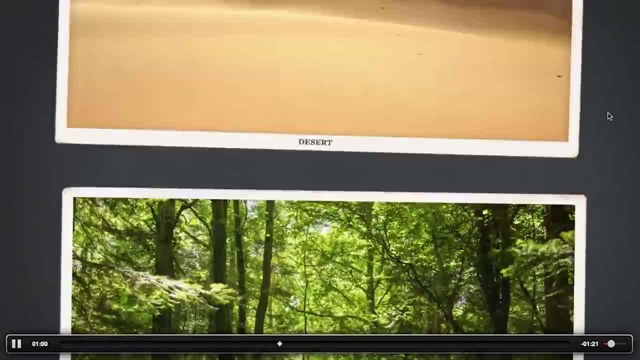 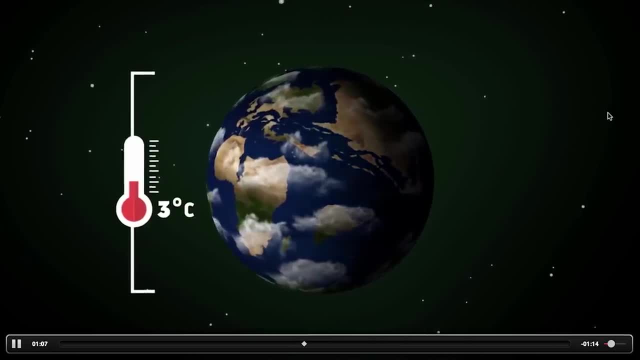 familiar shape were covered in habitats like temperate forests and deserts, and a belt of forests around the equator. But this environment was about to change. In fewer than 20,000 years, the global average temperature increased by 5 to 8 degrees Celsius, And the warming was 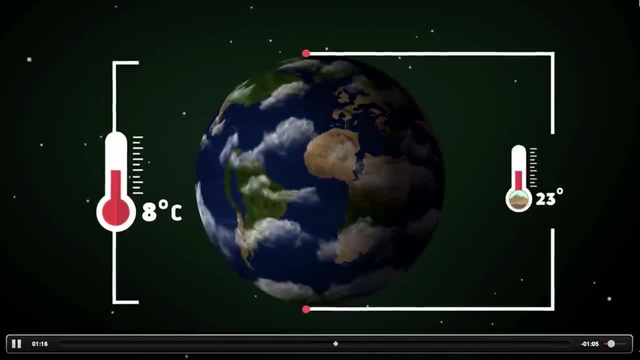 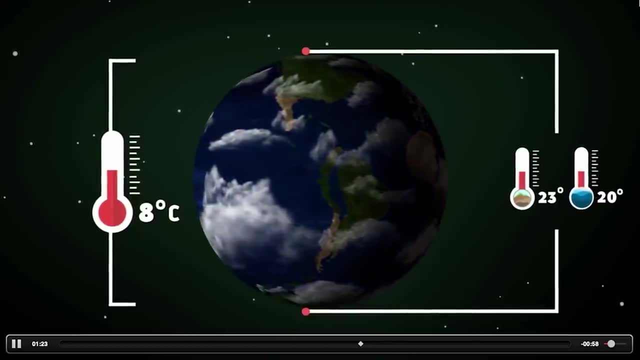 greatest at higher latitudes. So at the poles, temperatures on land reached an average of 23 degrees Celsius, while the ocean waters got up to a balmy 20 degrees. This means you could have gone for a comfy swim in the seas around Antarctica. This remarkable and sudden warming. 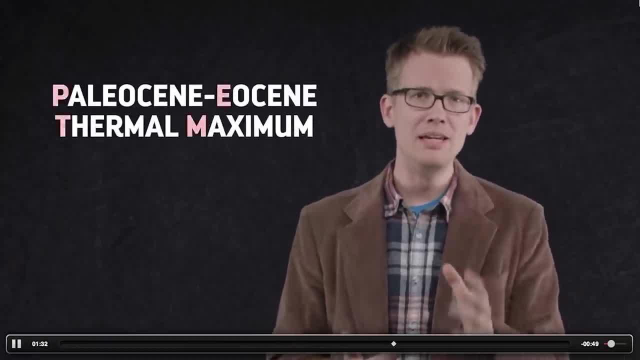 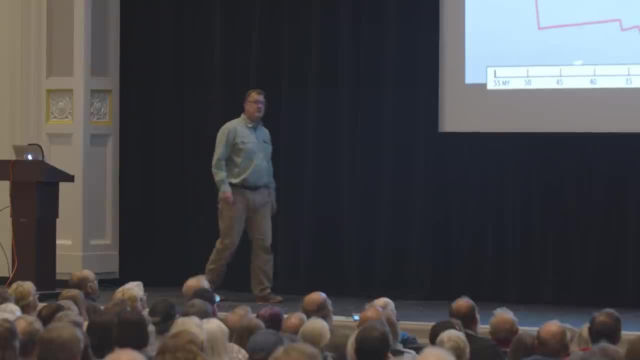 event is known as the Paleocene-Eocene Thermal Maximum, or PPM, and it had a massive effect on life on Earth. All right, One of these days I'm going to get brave enough to do a global climate lecture. I'm 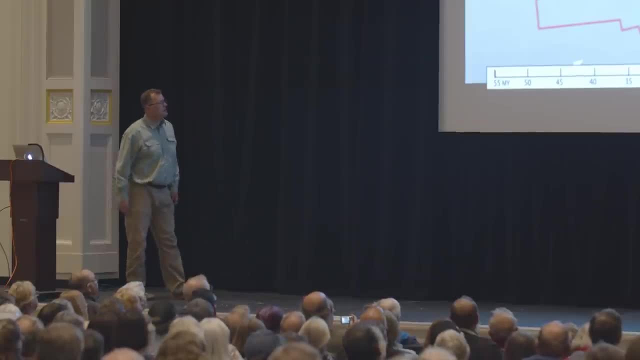 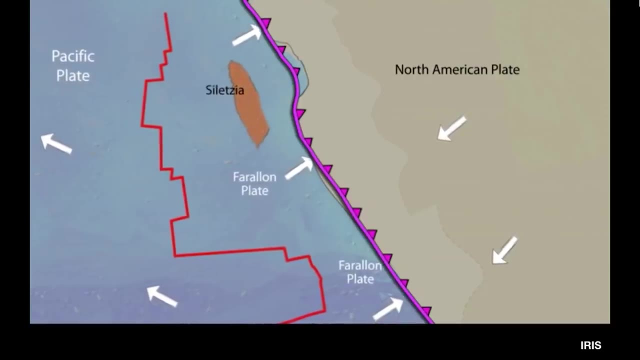 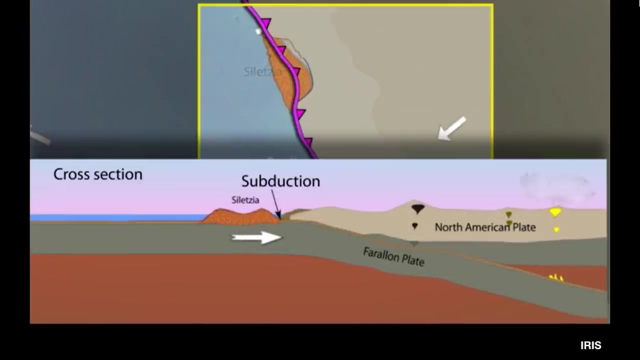 not quite there yet, but it's coming. I'm feeling like it's necessary. One of the ideas that I'm just going to throw out as conjecture: is it possible that Siletia, that huge shield volcano with 14 times the volume of all the basalts in the Pacific Northwest, is responsible for the 56 high? 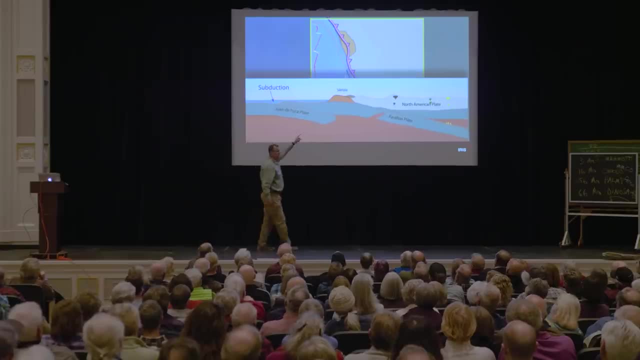 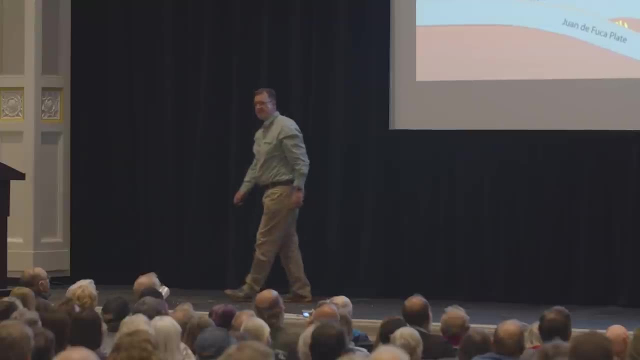 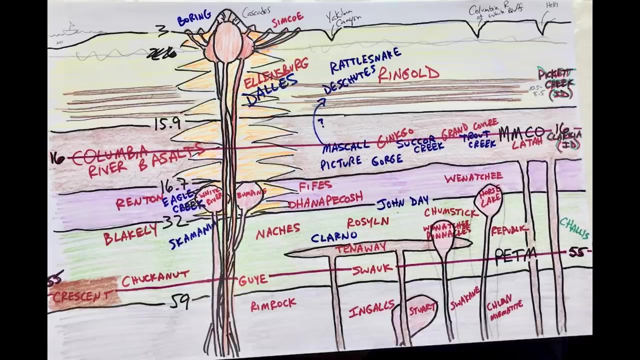 In other words, that oceanic island with an amazing amount of basalt and plenty of carbon dioxide coming out of the Earth was precisely at 56 million years ago. Just throwing that out Time for a professional diagram. This is me at my desk with my colored pencils, trying to keep. 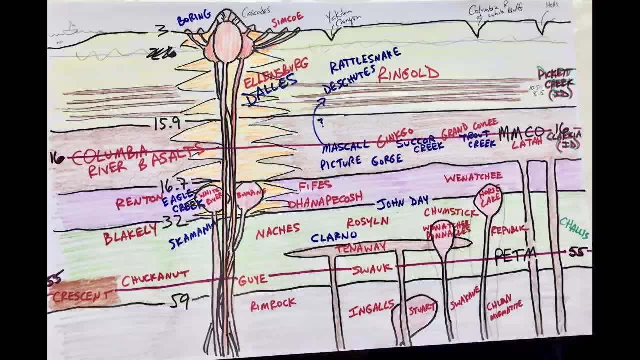 track of all these different spots. I know this is going to go quickly, but I want, if I'm giving a plant fossils lecture in the entire Pacific Northwest, I want to make sure we get a little taste of all these spots- Not every one, but all the red words are Washington plant fossil locations. 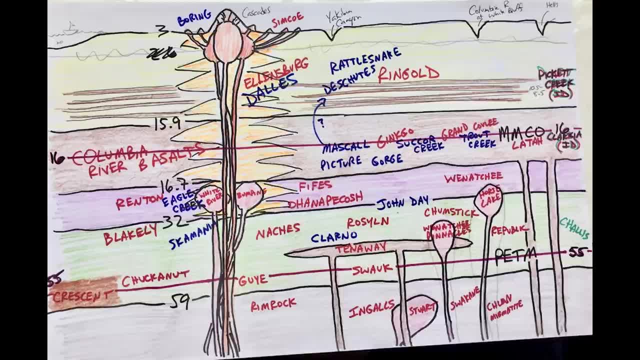 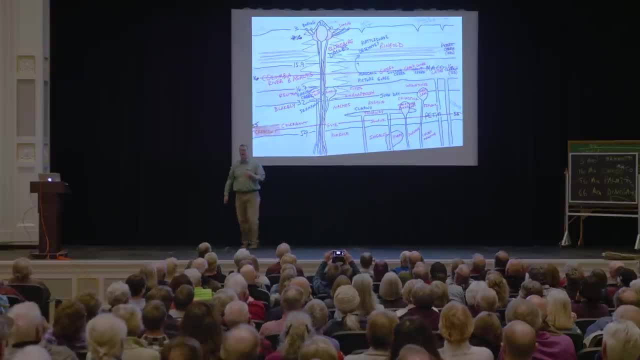 All the blue words are Oregon plant fossil locations- and there's a few greens in there getting us into Idaho- Plant fossils of the Pacific Northwest. And please note, we've got our PETM, our 56 hot down low and another line going across at that: MMCO, the mid-miocene climactic. optimum with our ginkgo trees and vanilla trees. I'm just going to give you a little�� to share with you what we built in the past, and then, with the butlenose, we'll get to the next slide real quickly. We've got plant fossils of the Pacific Northwest And, please note, we've got our. 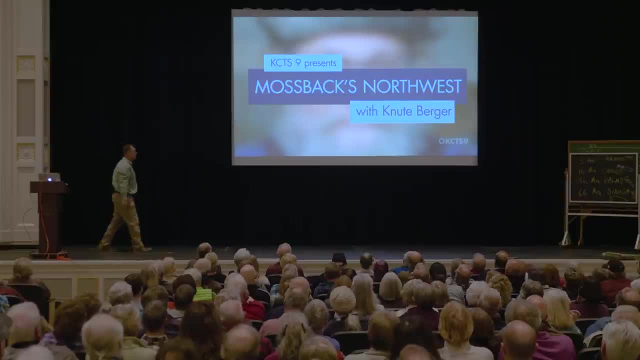 PETM, our 56 hot down low and another line going across at that, MMCO, the mid-miocene climactic optimum, with our ginkgo trees and Vantage Knute Berger from downtown Seattle. Today we're at the Burke Museum. 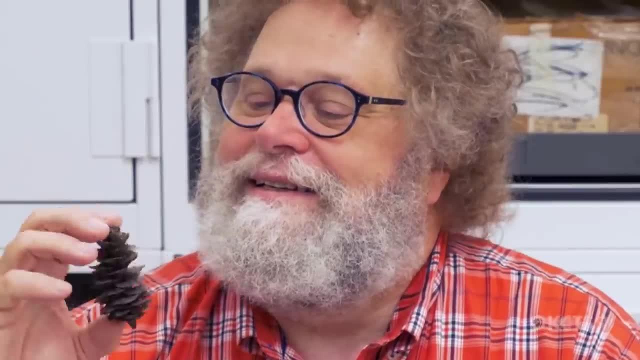 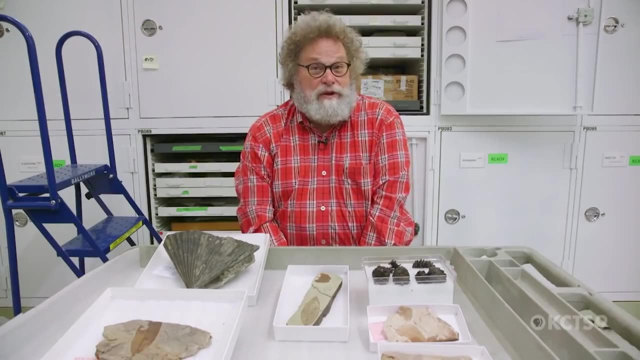 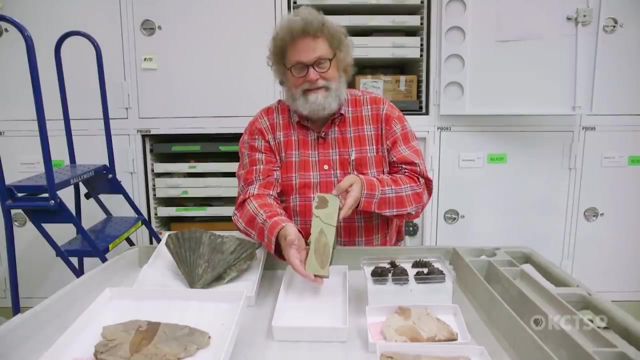 in the paleontology department. The one thing people in the Pacific Northwest think they know is our climate, But what a lot of people don't know is that the Pacific Northwest wasn't always the gray rainy haven that we think of it today. About 50 million years ago, palm trees thrived here. 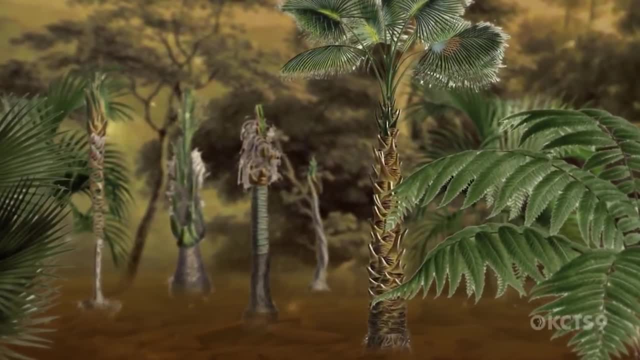 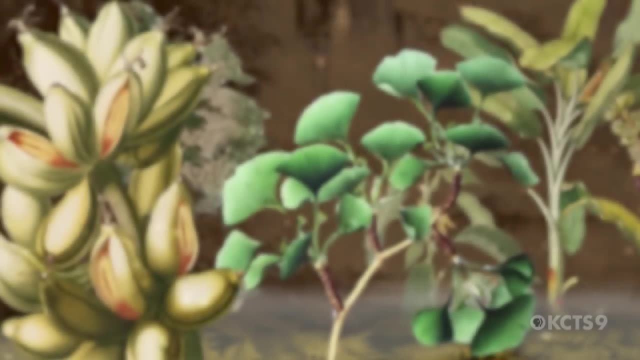 So imagine the Bellingham area. you're in a palm forest, something like you would find in Central America. Think Costa Rica. You move ahead maybe to 40 million years ago. you're getting ginkgo trees. That's a climate that's similar to the Deep South. 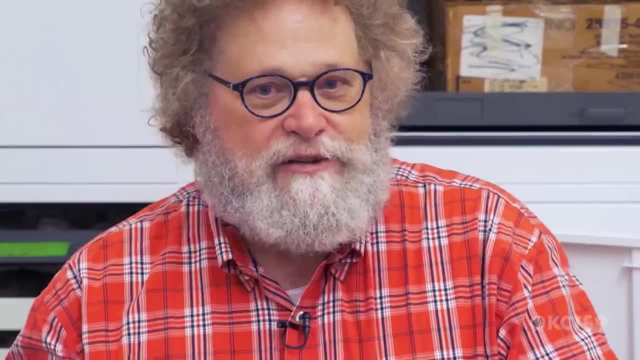 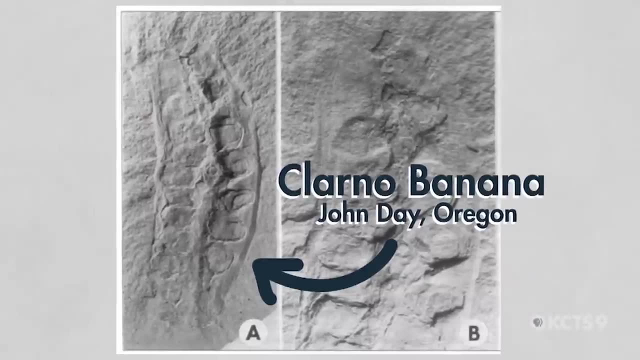 In Central Oregon, they've actually found fossils of banana plants. You think of the Pacific Northwest. you think of the Pacific Northwest. you think of the Pacific Northwest. You think of apples. 44 million years ago it was bananas, So that's a great reason to transition. 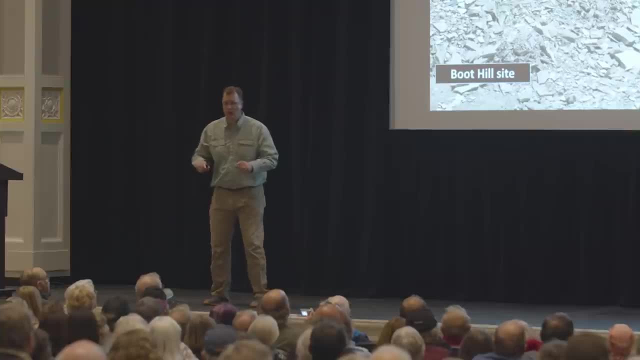 to slightly younger plant fossils. Hold on to your hats now. We're gonna go all the way across the Pacific Northwest, stopping at places that, if you're a plant fossil enthusiast, you've been to multiple times- Republic, Stone Rose- You've been in your family with up there. 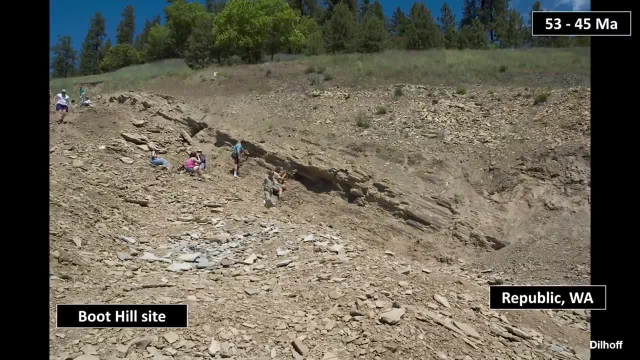 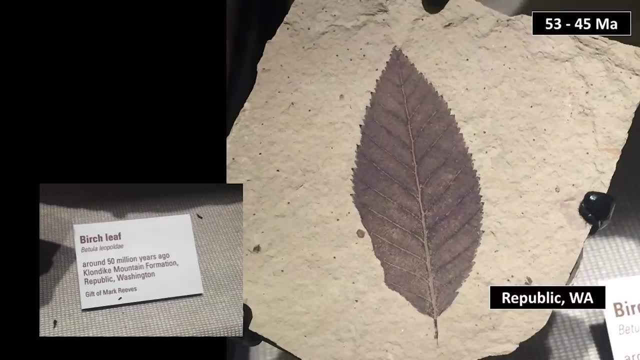 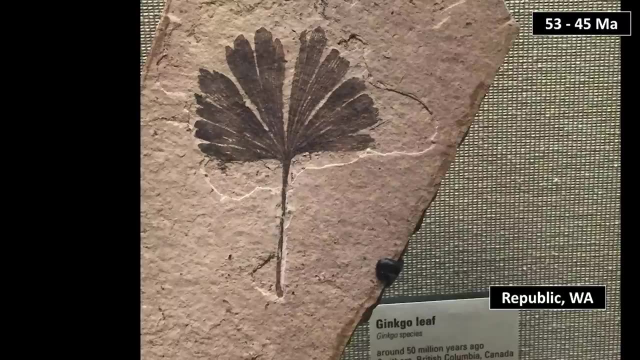 You've been collecting up there through the years in North Central Washington. We're slightly younger, 53 to 45 million years ago, kind of overlapping with Swahk formation time. But look at these fantastic plant fossils and leaves coming from the Republic area. 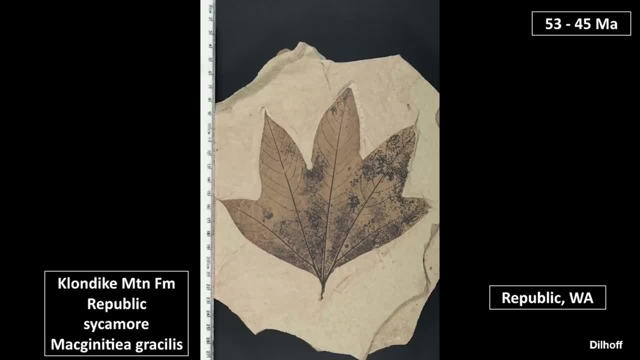 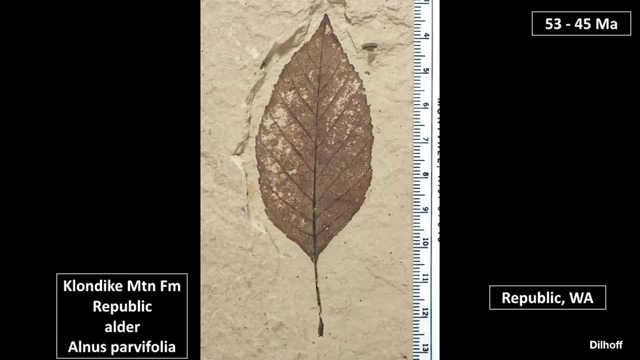 and these sedimentary beds preserved there. Many of these photos from Tad Dilhoff at the Burke. I've already mentioned that, but they've got a treasure trove of fossils across the Pacific Northwest with amazing levels of preservation, And some of these are ginkgo. 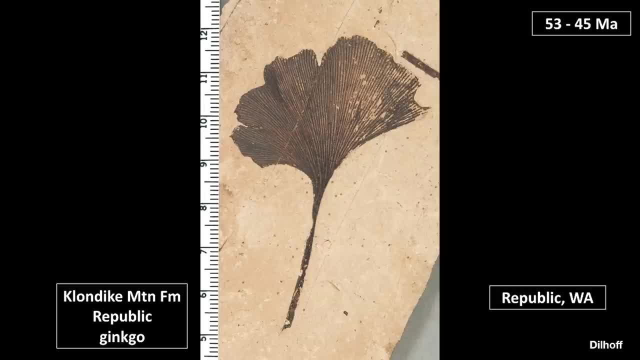 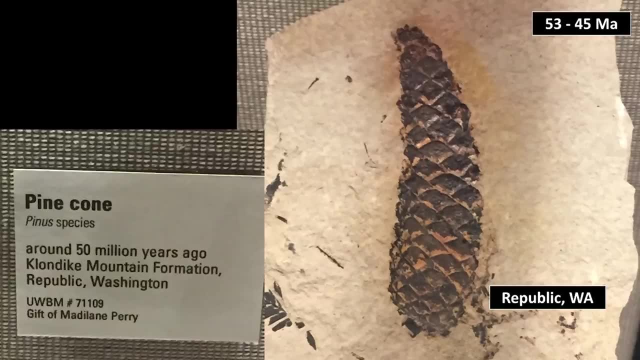 So we can get confused. You know our ginkgo discussion tonight was 16 million years ago. but here we go with some ginkgo trees as early as 53 million years ago And pine cones, all from the Republic area. 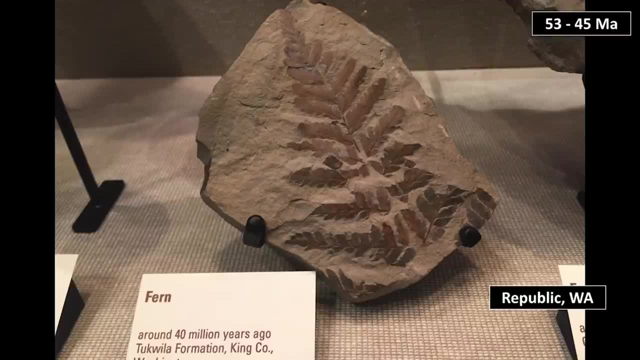 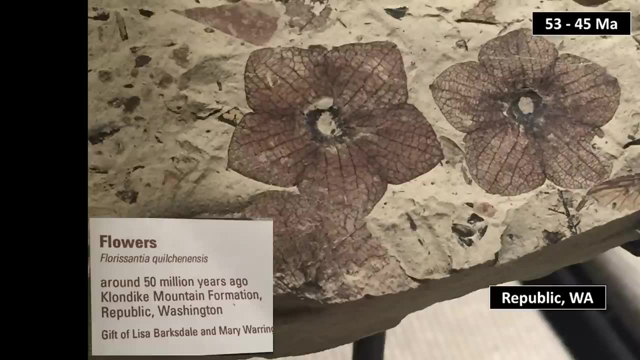 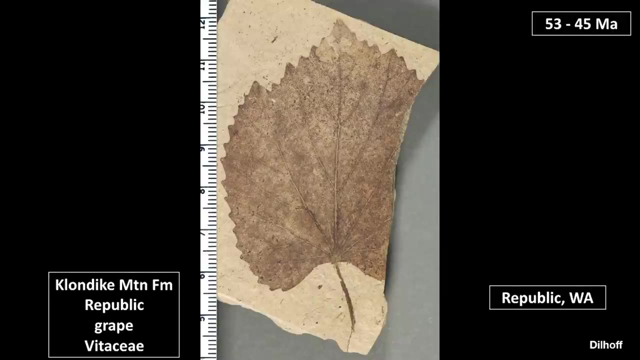 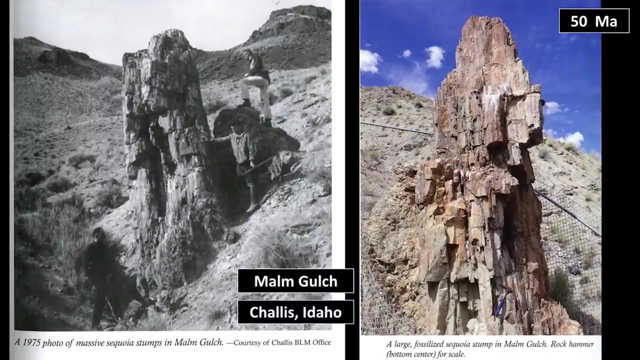 We're still in North Central Washington now, Slightly younger than 56 hot, Even flowers preserved in the Klondike Mountain formation. Isn't this amazing Stone rose? get it All right. great Grape leaves, maple leaves, So it's not a fossilized tree trunk story. 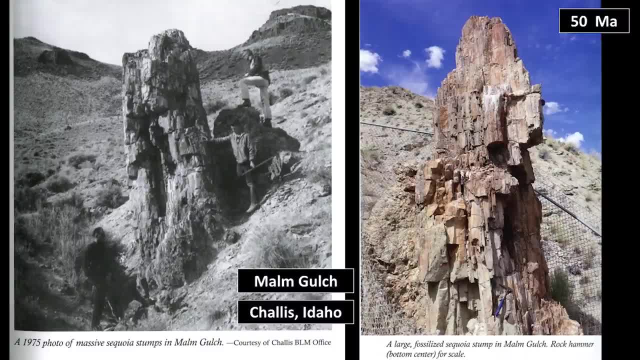 primarily in republic. It's more of a leaf and delicate insect and fish story. Jump over to Chalice, Idaho. There's a giant sequoia tree stump, 50 million years old, related to the Chalice volcanics. I told you we were gonna jump around. 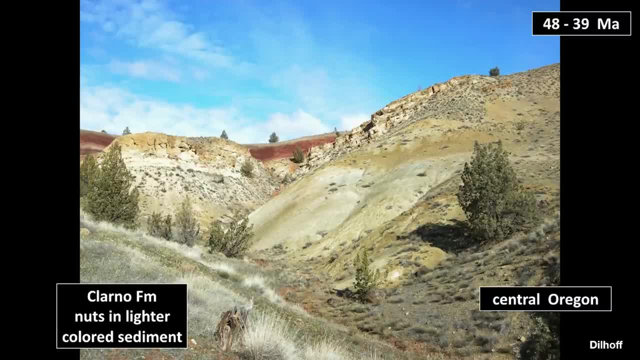 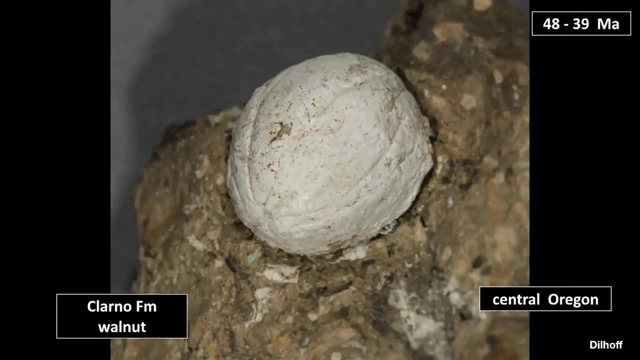 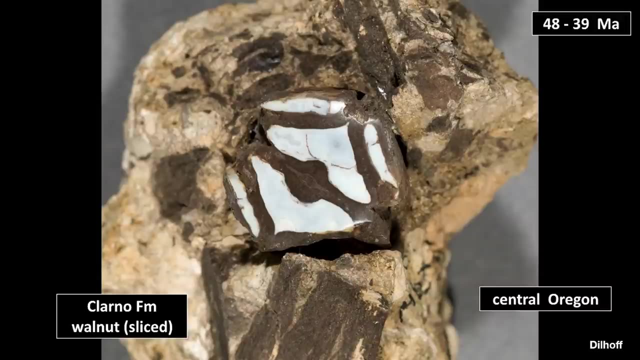 Central Oregon, Oregon, now down by John Day 48 to 39 million years ago. What kind of fossils can we find? especially in these lighter colored sediments, We can find walnuts fossilized in the Clarno Formation 48 to 39 million years ago. We can slice through the walnut Back home, rosaline. 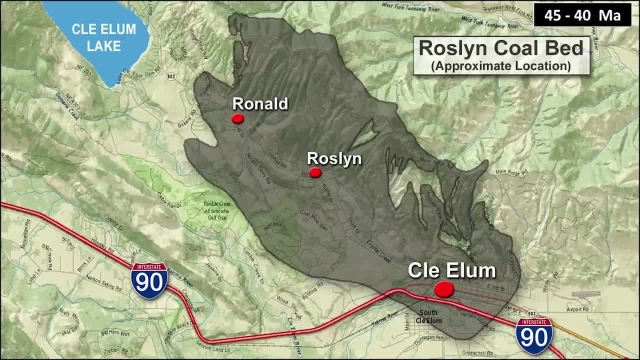 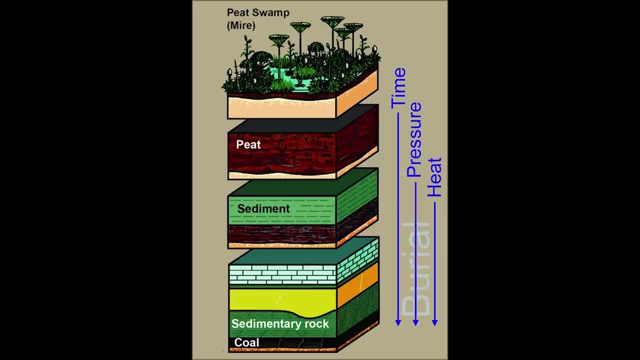 Well, that's just a bunch of coal. Well, technically that's plant fossil stuff, isn't it? We know how coal forms. The coal beds of rosaline in the upper Kittitas County are the result of swamp-like vegetative mats that are buried deeply enough to convert that vegetative matter into rock. 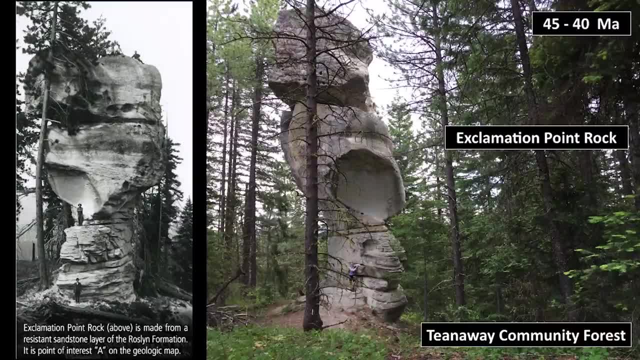 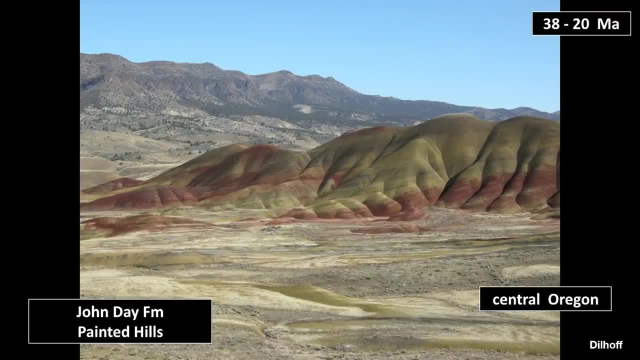 essentially coal, And all through the Teanaway Community Forest these spires of sandstone of the rosaline formation are in amongst the coal beds. Back down to Central Oregon, the John Day now in the Painted Hills, We're getting younger, 38 to 20.. 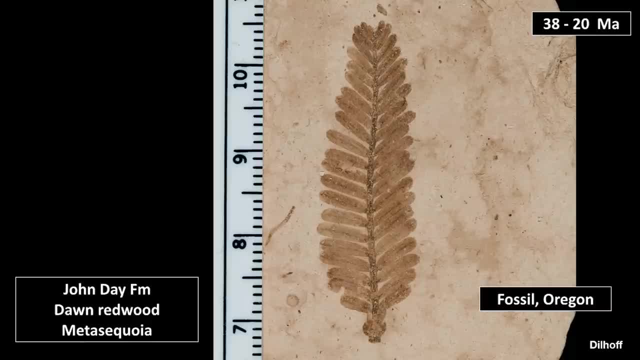 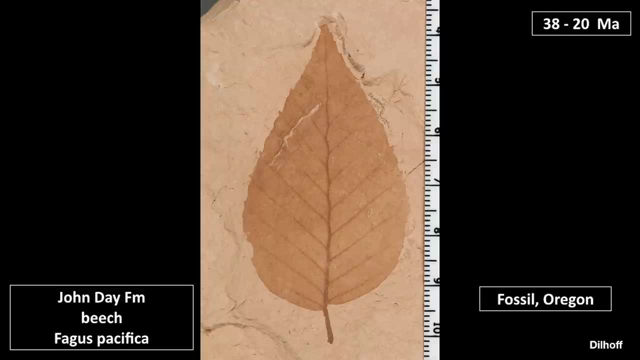 million years ago And in the John Day redwood- This is all at the high school there in Fossil Oregon. if you've dug there 38 to 20 million years ago, Beech leaves, birch-winged fruit. 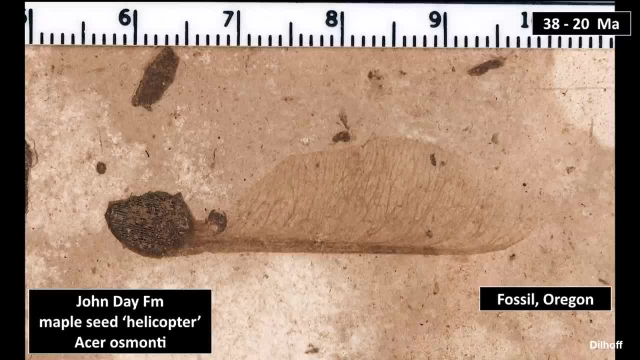 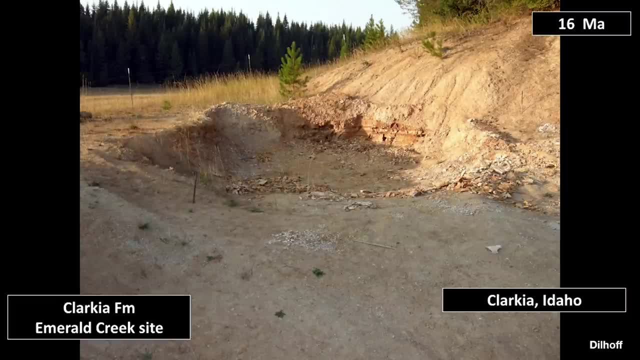 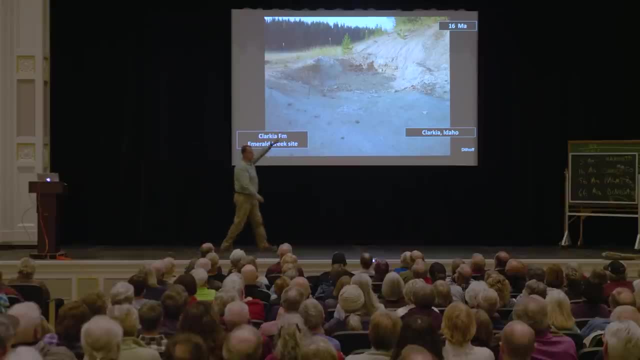 freaking helicopter from a maple tree: Clarkia, if we jump over by St Mary's, Idaho, a little town of Clarkia, and there was Lake Clarkia. Now let's be careful. Suddenly we're at 16 million years ago. Suddenly we are going to stop and realize we are at the time of 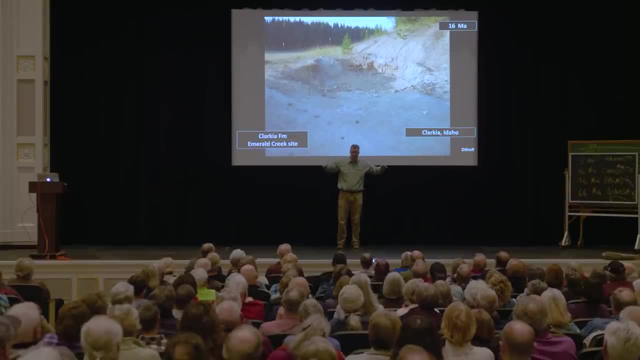 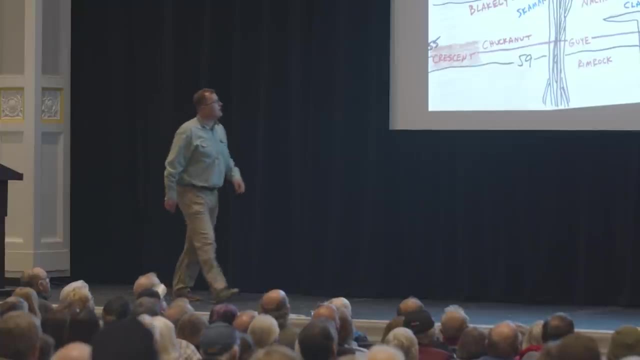 our Ginkgo Petrified Forest State Park, remember, in the Great Lavas. So the rest of tonight we're going to be basically in that mid-Maya scene. So thank you, I need that now. So this red line going from through the Columbia River, Basalts, heading all the way over to Clarkia. 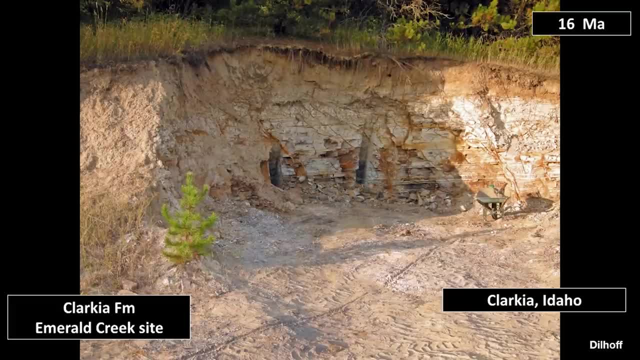 Idaho will help us realize that there's a lot of red line going through the Columbia River Basalts, a lot going on across the Pacific Northwest during the time of our crazy logs being carried from God knows where 16 million years ago. In northern Idaho, in the Clarkia, there's an 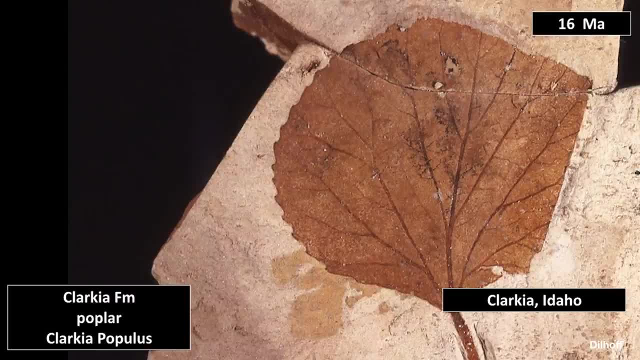 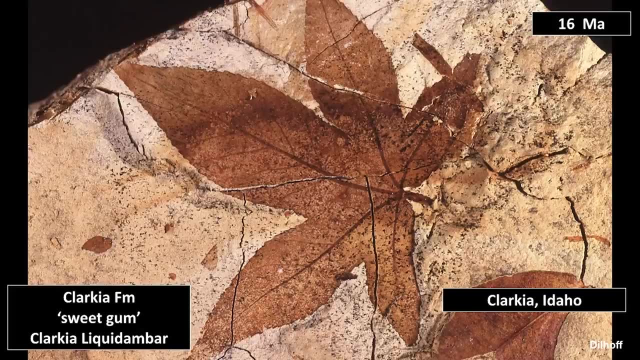 amazing amount of preservation of magnolia, tulip tree leaves, poplar leaves, sweet gum- Again, leaves instead of the tree trunks, but ultimately telling the same story: We're now into pollen and getting the best out of it. We're now into pollen and getting the best out of it. 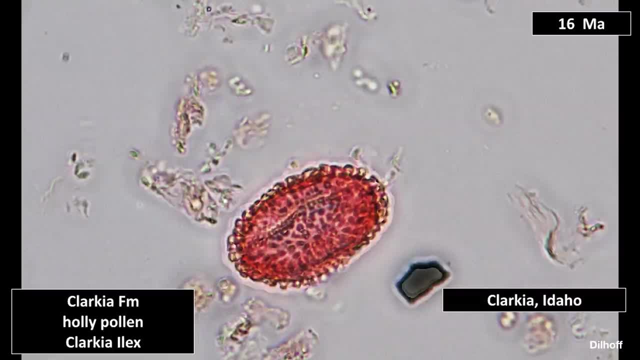 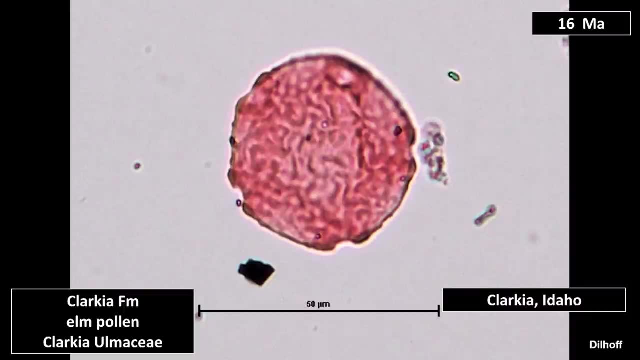 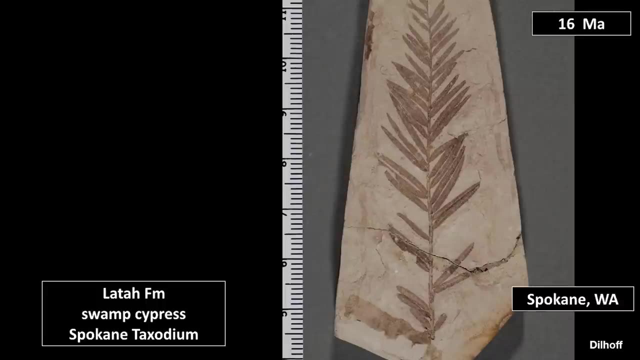 exquisite details of climatic conditions from the pollen in much of the fine-grained sediments in the Clarkia area. All photos from the Burke Museum. If we jump over to Spokane there's a series of beds pretty close to downtown, you know the Hangman Creek area or Leyta. 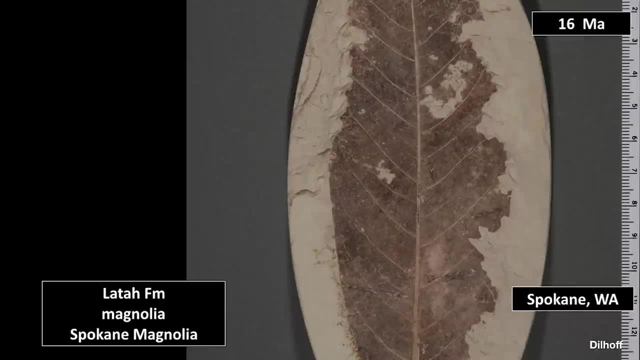 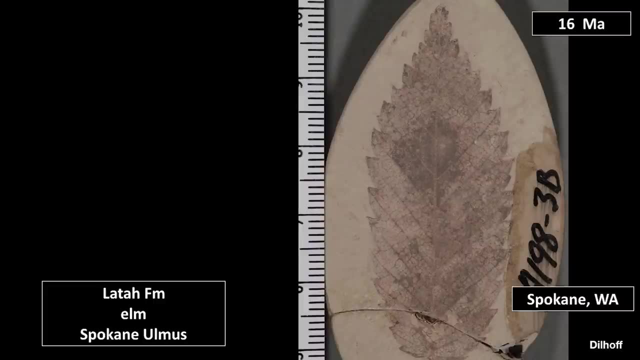 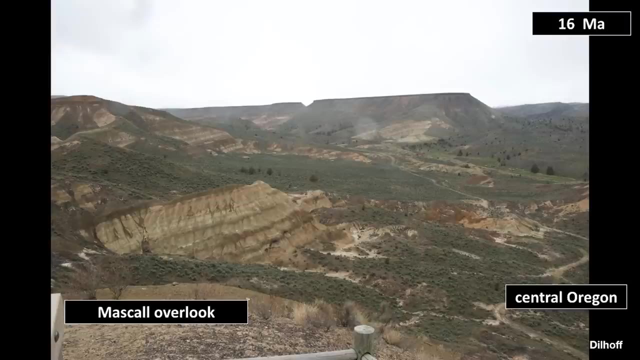 There's a whole area there. This is again pre-ice age, but we can preserve a lot of the leaves from a lot of the trees and other plants. at this time in the Spokane area An elm leaf, an oak leaf from the Leyta formation Back down to central Oregon, back down to the John Day country. But 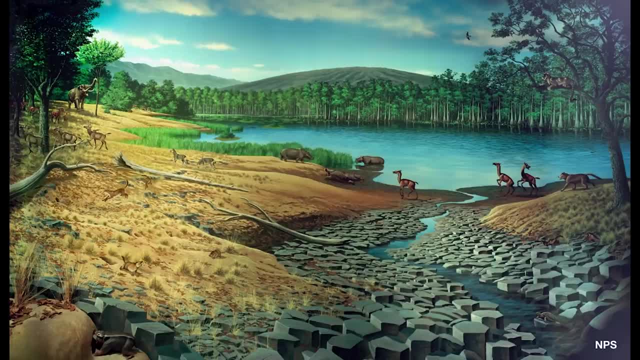 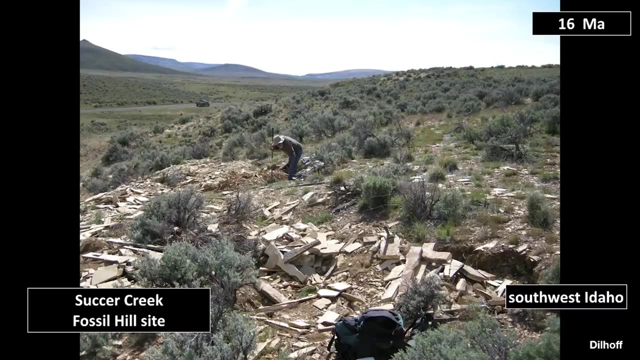 these are the Mezcal areas that are helping us realize that we had this Miocene scene with rhinoceros and other creatures among these exotic swamp-like creatures, The Mezcal White Hills and the fossils. The fossils are coming from the White Layers in central Oregon And finally in the Owyhee country. 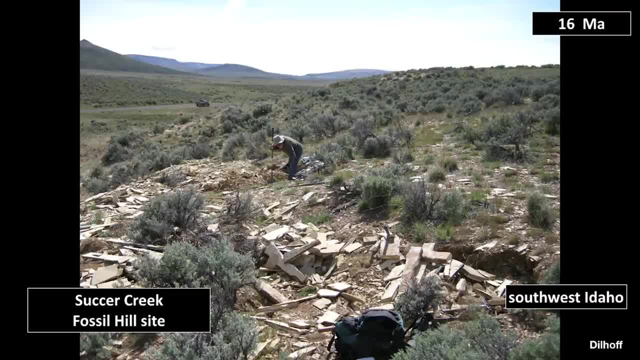 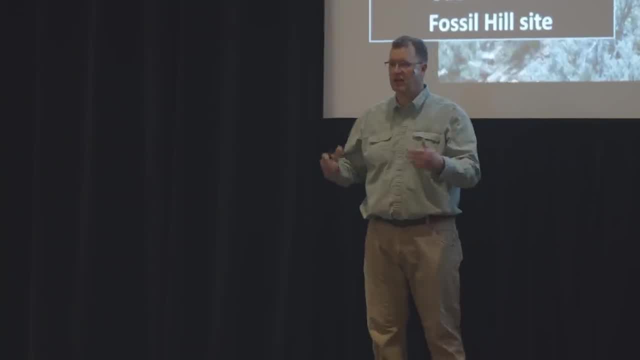 of southwestern Idaho, Sucker Creek, So I don't know much about any of these places, I have to confess to you. I communicated with this buddy of mine, Ted Dilhoff, and said: look, if I'm giving a lecture on plant fossils in the northwest, can you give me a list of places that I really should make? 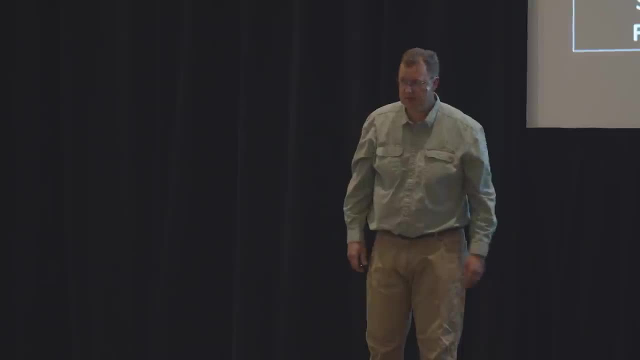 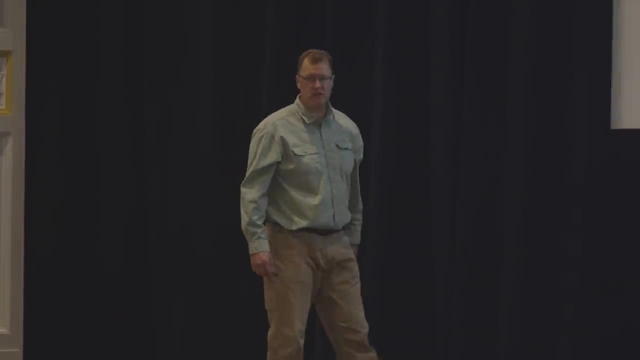 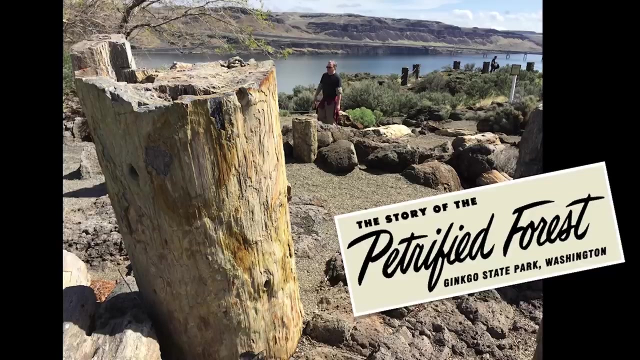 Well, we were trying to make a lot of this stuff, So that's why we're glossing over many of these spots and choosing to hammer two stories pretty hard. So this is the second of our two stories: The famous Petrified Forest at Ginkgo State Park. Where is it? 30 miles east of here. 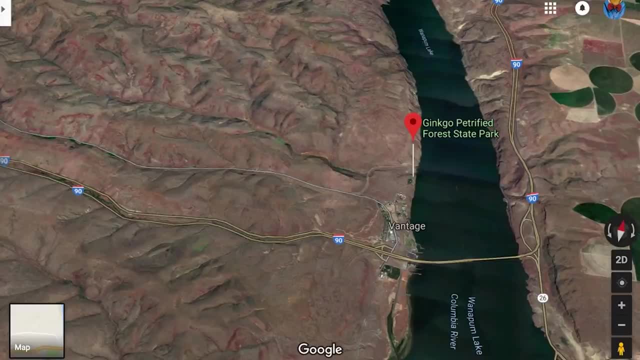 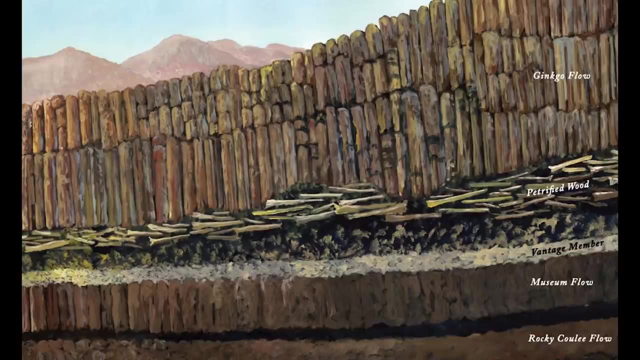 where I-90 crosses the Columbia River Hotter than heck in the summertime. Ginkgo Petrified Forest, just a mile off the freeway. So here's a key diagram for us. It's part of a new exhibit that will be on display at Ginkgo this summer. 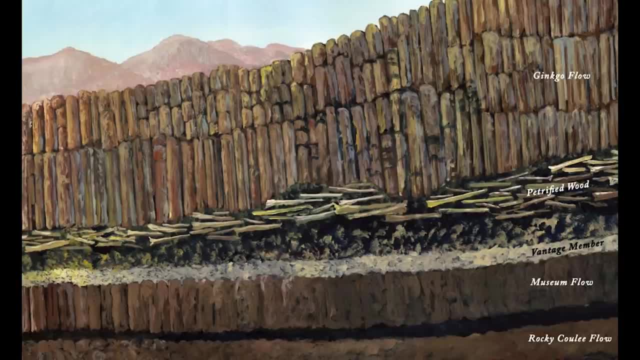 There's our Ginkgo flow And at the base of the Ginkgo flow we can see all of our logs tucked in with the pillows. and all the logs, importantly, are not in the Vantage sediment, they're directly above the Vantage sediment. 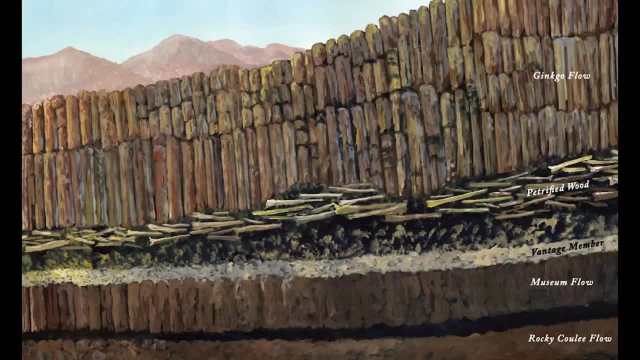 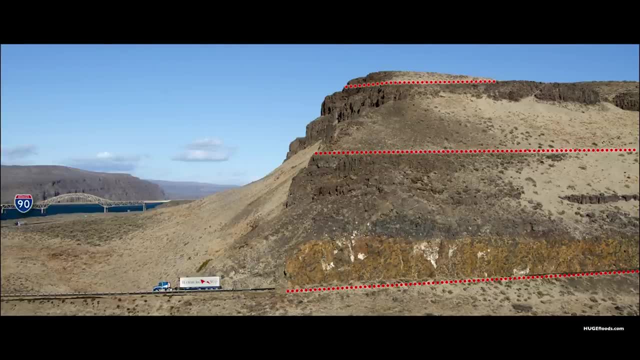 Every log has been transported, presumably before the Ginkgo flow arrived on the scene. Here's the Ginkgo flow, a photo from Tom Foster looking north. there's Vantage in the bridge. there's two of these great lava flows. 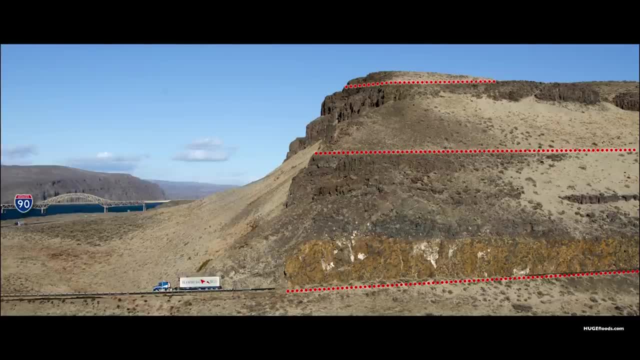 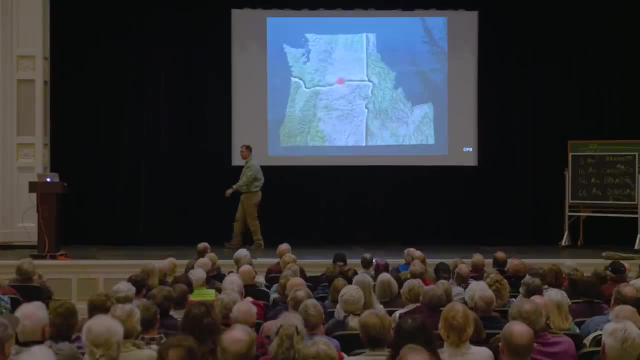 You see the scale of these lavas And you see that orange kind of weird area down in here. Here's where the petrified wood is located in the pillow zone of the Ginkgo lava flow. So many of us know these great lavas. 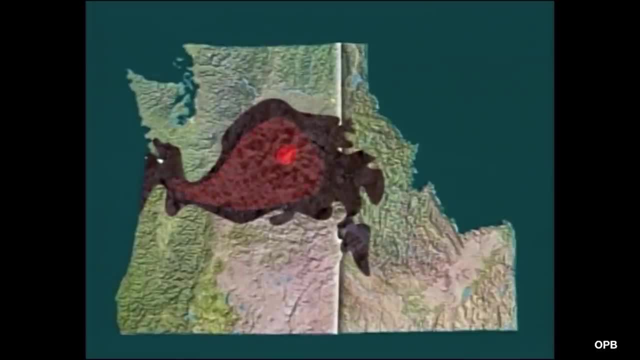 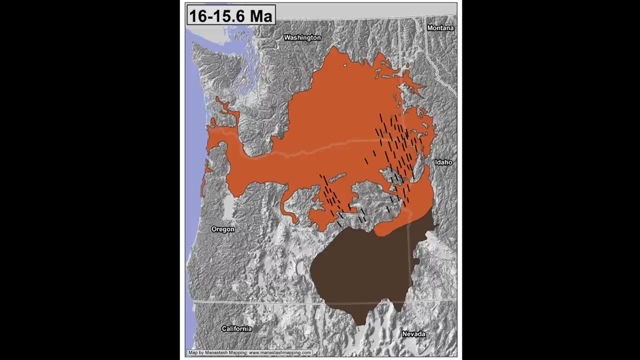 are an inland Pacific Northwest story. It's got nothing to do with the Cascades, And these Hawaiian-like lavas came out of cracks which are in extreme Southeast Washington and Northeast Oregon. The cracks flowed through the Ginkgo formed 16 million years ago. 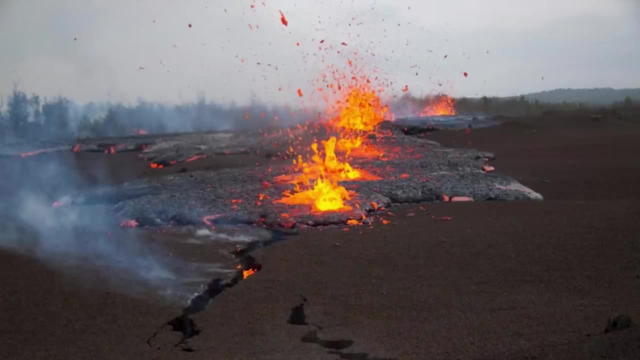 and the mafic magma- that's very fluid- came to the surface. Here's a miniature version of what it must have looked like. This is at Kilauea Volcano in Hawaii, showing a fissure sowing some mafic magma. 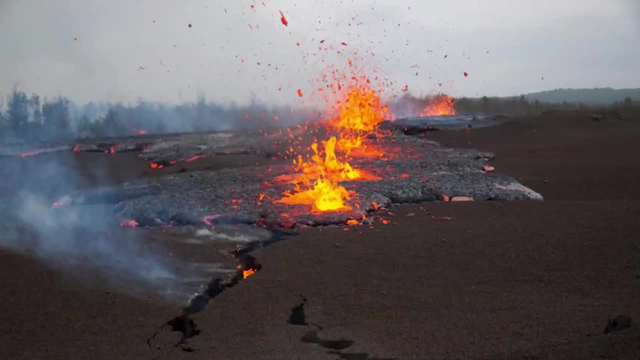 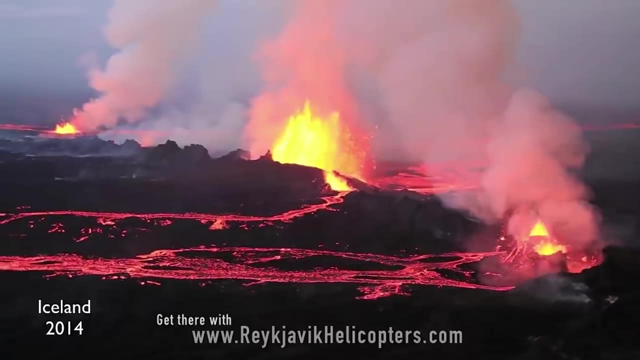 and showing not only spatter at the vent but flows flowing away in both directions from the fissure. That is the story with the Ginkgo flow, our friend tonight, but all 300 of the lava flows that flooded the inland Pacific Northwest. 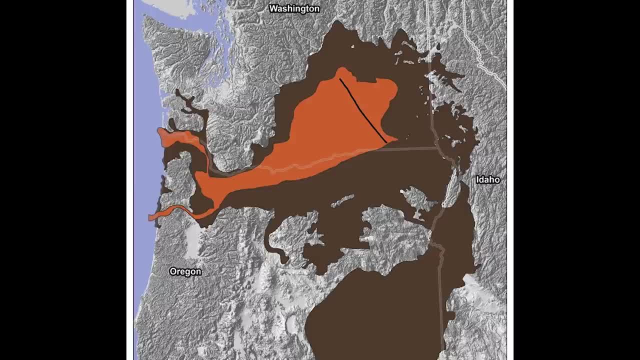 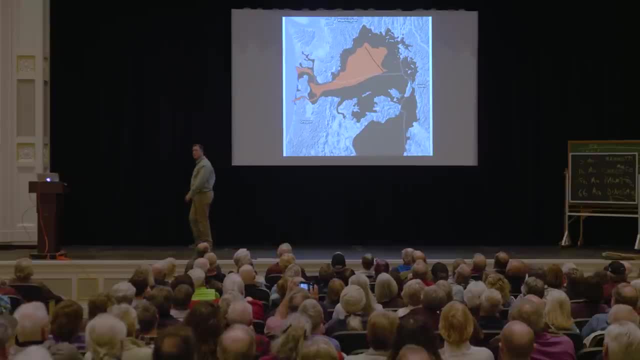 There is the precise fissure for the Ginkgo which I tried to draw on the green board just a second ago, And there is the Ginkgo lava crossing through the Cascades- The Cascades were low at the time in places- and getting to a part of the Oregon coast. 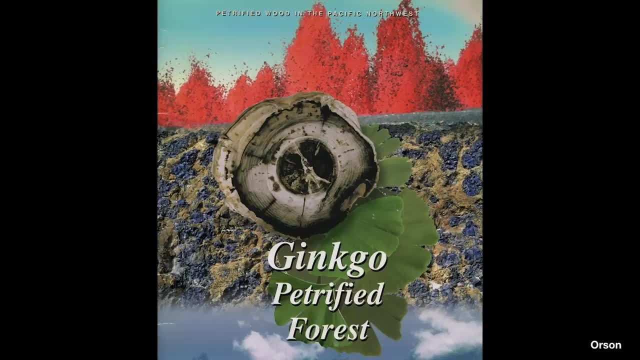 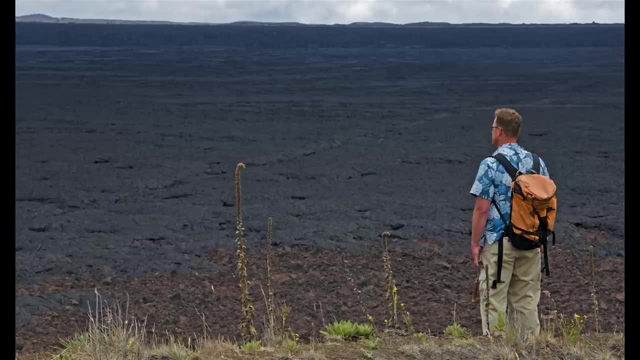 in two different places. The lavas and the logs are intricately connected in the vantage area. An important concept is: when we petrify those logs, we completely seal them off from the surface, And so if you are one log, who is remembering? 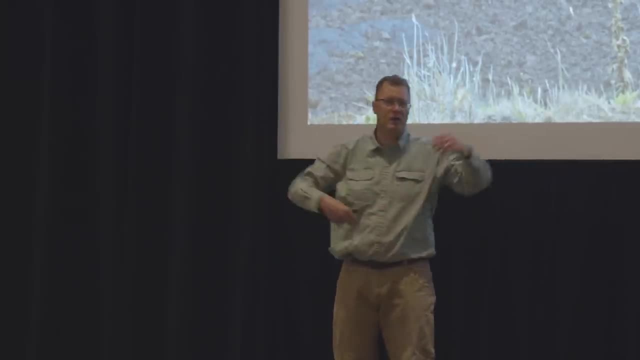 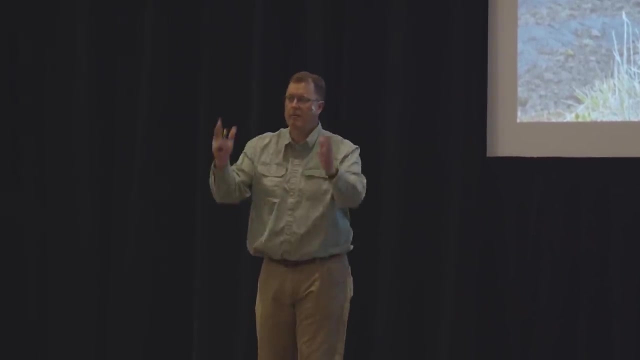 this kind of swampy, wet time. whether you're a log from the Okanagan or the Cascades, you're underground for millions of years until the Ice Age floods come through, rip up a bunch of the bedrock and suddenly reveal a desert. 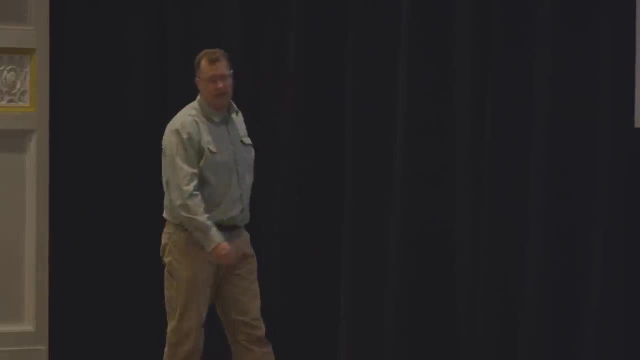 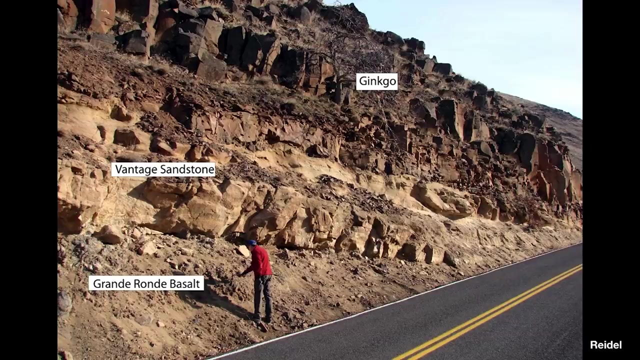 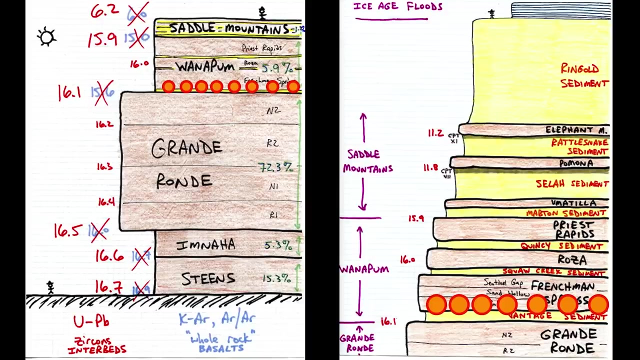 We went through this complete change in climate in the last 16 million years. Okay, here we go. Ginkgo: flow above, vantage sediment underneath. We're going to keep going back to that. If you're a real junkie with geology. 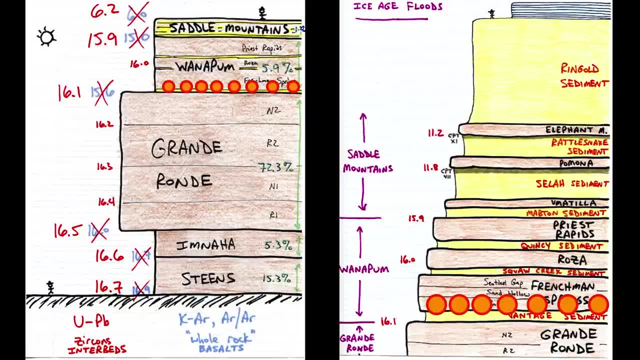 you should be alerted to the fact that we now have more precise dates for the great lavas and the sediments in between, And all I'm showing here is that we used to have a date of 15.6 million years for those Ginkgo logs. 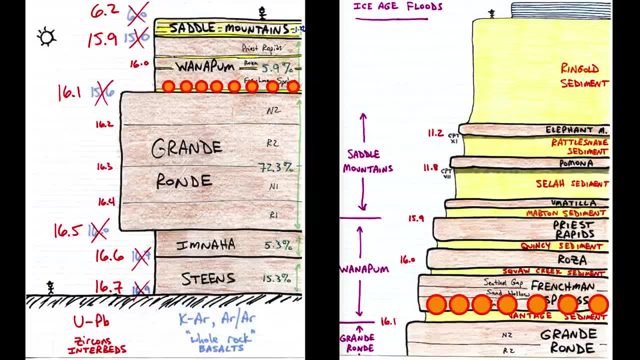 It's now been changed to 16.1.. Who cares in general? But for those of us that really study carefully, there's zircons that we can pull out of the interbeds And get more precise dates. Okay, so it's the logs that are the fascinating part of this. 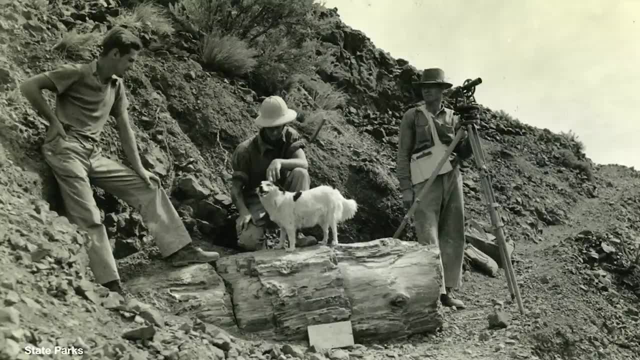 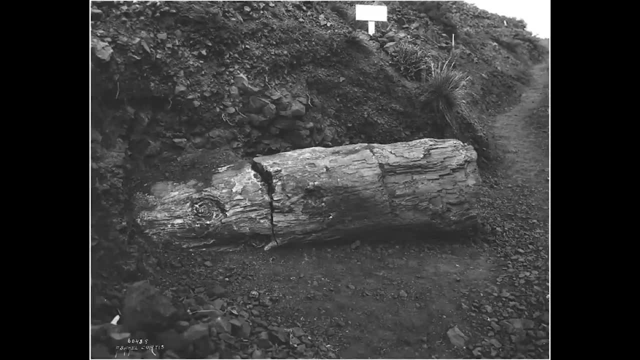 And it's the logs that were discovered first by George Beck, the guy who taught here in town in 1931.. He is the reason for Ginkgo Petrified Forest State Park- Again, exhibits from state parks starting to show up. 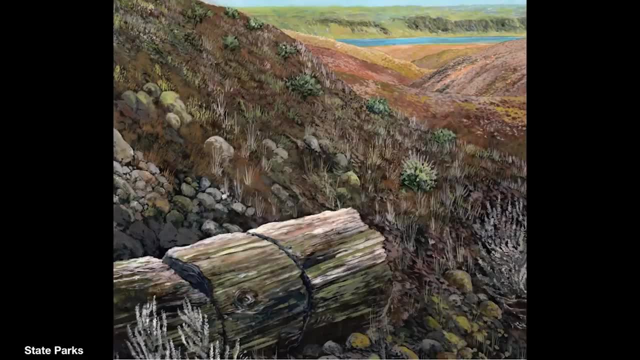 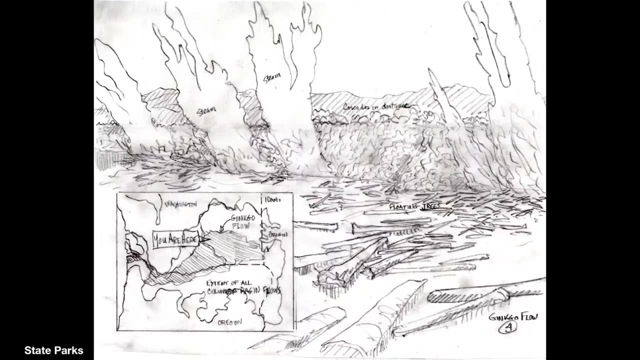 And we've had back and forth between the artists and the scientists to try to create watercolors that have relevance to our current understanding. And that's what we're trying to do with the Ginkgo Flows: We're trying to create watercolors that have relevance. 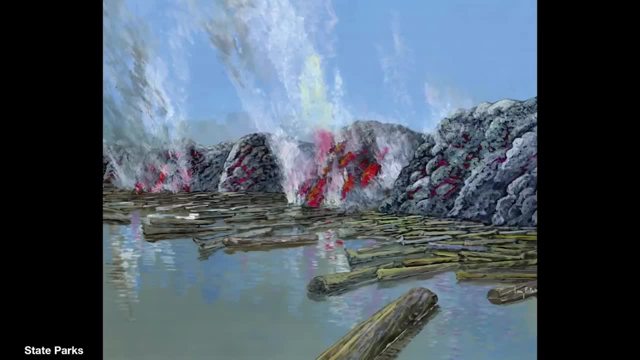 to our current understanding of those logs, even though there's still a major mystery left. This artist, Sam, did a beautiful job with these things. There's the Ginkgo Flow coming into Lake Vantage and dealing with these waterlogged tree stumps. 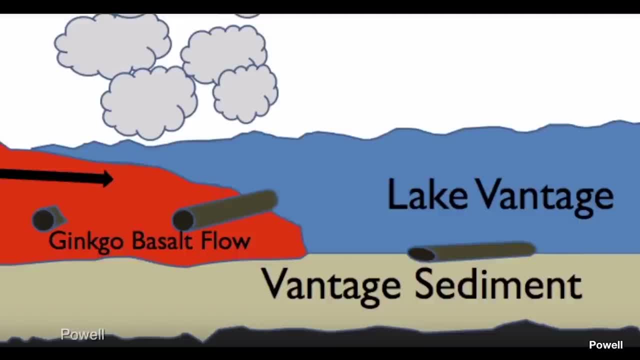 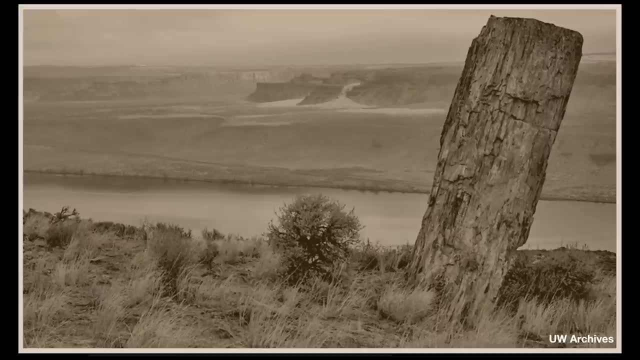 tree trunks that don't have roots. None of them have roots, None of them are in growth position. Jack Powell with a cartoon to give us a sense of the Ginkgo Flow coming in, And I would swear that they've been standing there. 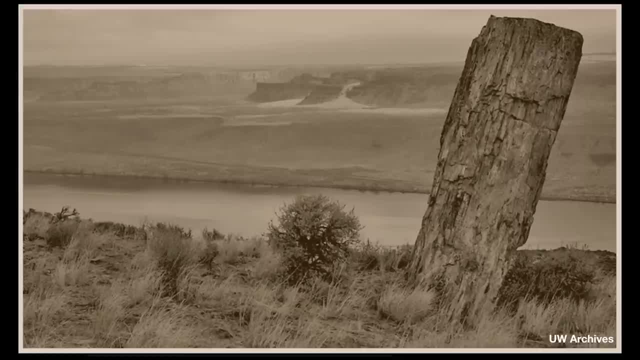 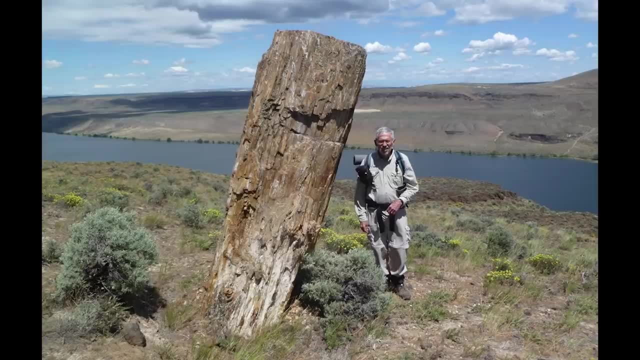 for 16 million years. This is a favorite of mine, which is on the ridge north of the museum, And it caught my eye a few years ago on postcards et cetera, And it's still there. You can hike out to it. 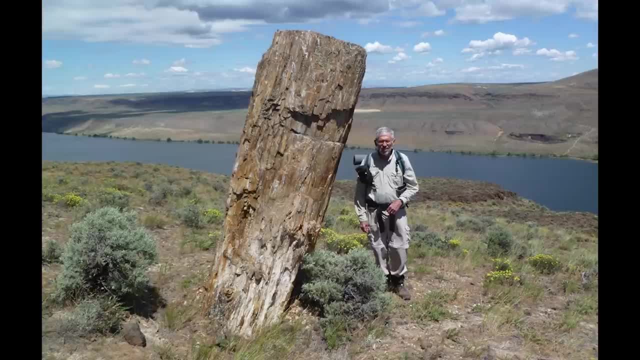 I'll send you out there. It's a bit of a hike but it's glorious. But the important point is that was entombed in the pillow zone of the Ginkgo Flow and everything's been eroded away, except for that log. 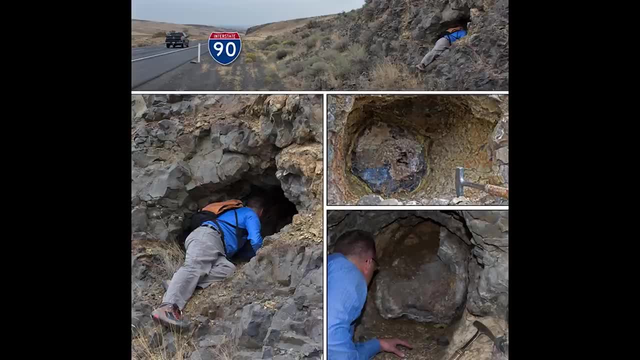 Along I-90, a couple miles east of Vantage. if you're thoroughly wide awake you can see some big holes along the road. When they put in I-90, they took a bunch of logs out of the area And those holes if you crawl back into them. 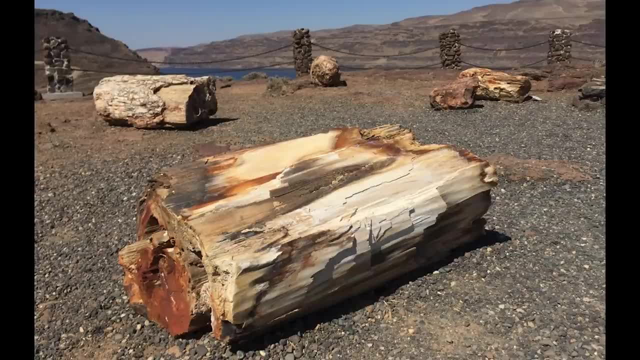 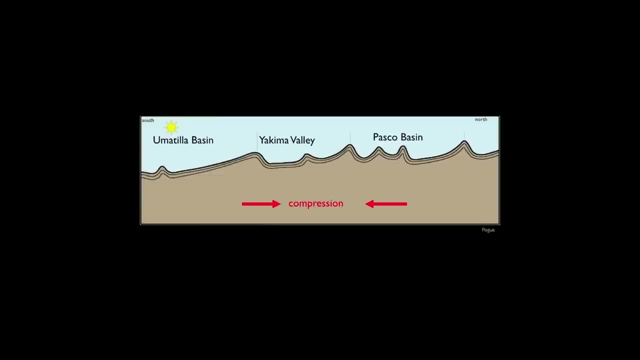 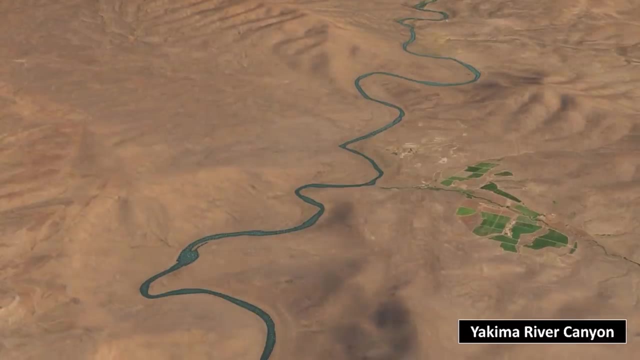 have petrified logs within them, And some of those logs are now for close inspection at the museum. Many of us know that those layers have been folded because of tectonic squeezing, And not only the squeezing has made the ridges, but it helped form the Yakima River Canyon. 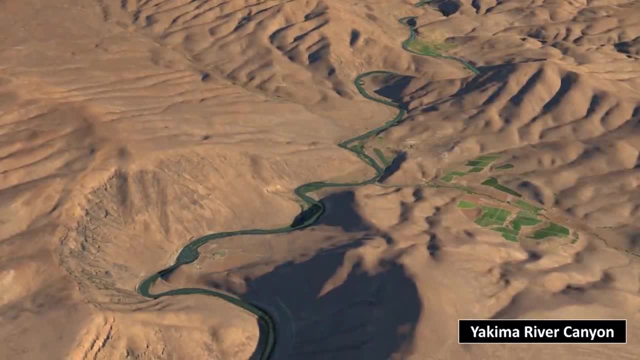 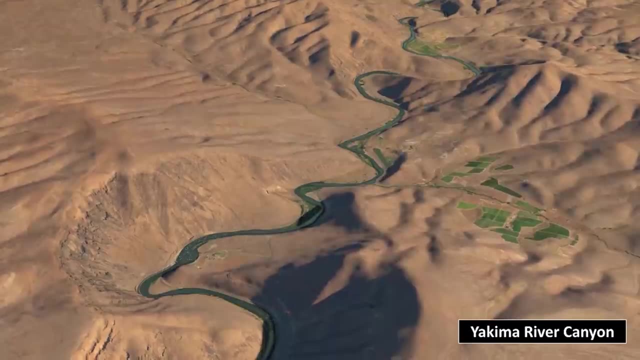 So there's petrified wood. in the Yakima River Canyon. There's actually more than one forest horizon, but we're focusing primarily on the Ginkgo horizon. tonight, Let's visit the walls of the Yakima River Canyon with some old footage that we never used. 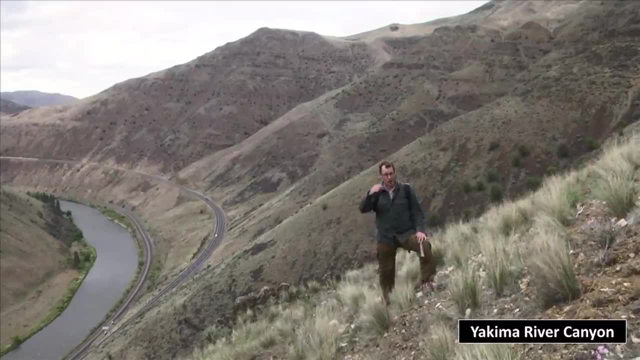 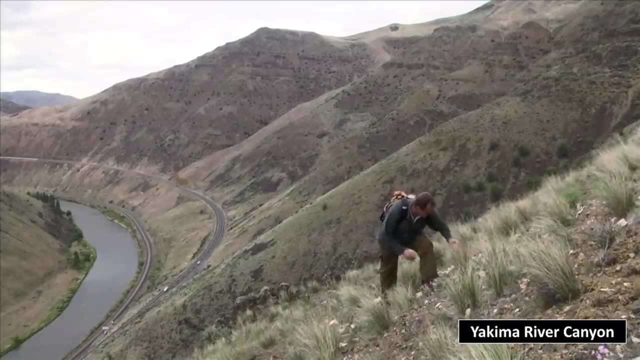 and so it's a bit rough, but I want to use it anyway. We're up on one of those layers right now, And all over the ground, amongst all these beautiful wildflowers, is petrified wood Stacks of it. 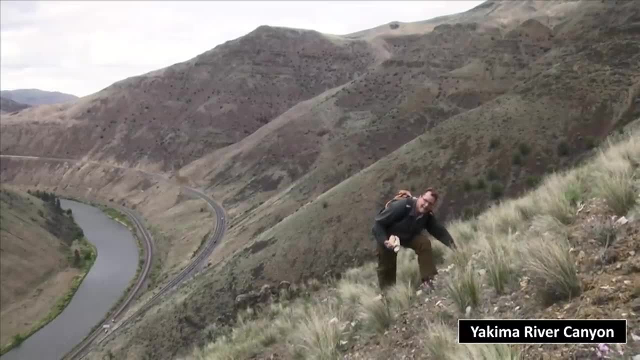 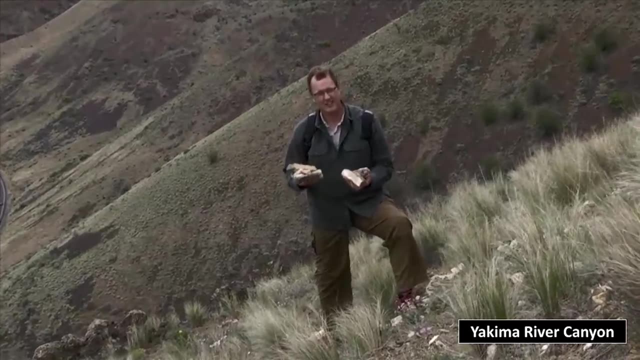 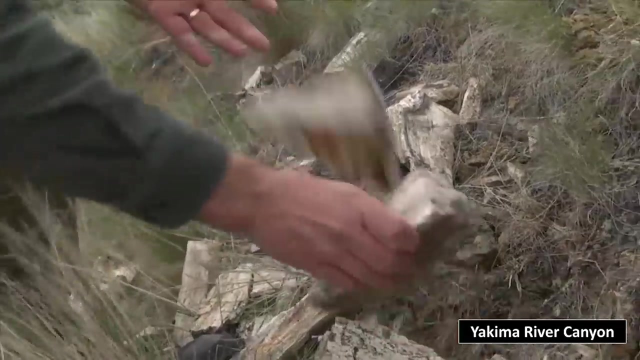 Like I'm sent to the backyard to go get some wood, bring it in for the fire. But this wood's got heft: 15.6 million-year-old wood that feels like stone, feels like rock instead of wood. So how does this work? 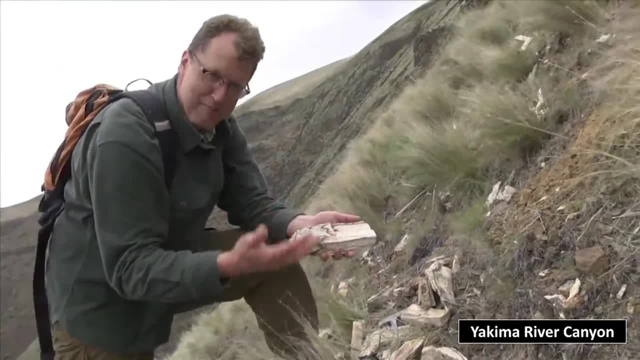 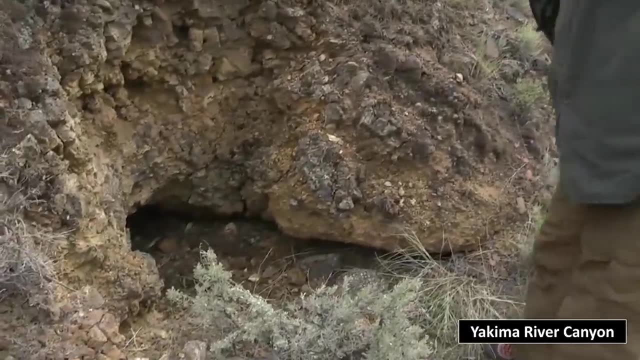 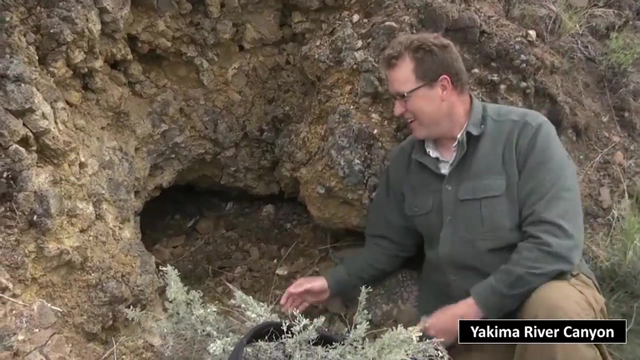 How do we get wood to turn to stone? How do we get it to petrify? All right, this is what I'm talking about. Check this out. Oh gorgeous, This is a hole in the hillside where a petrified log was sitting. 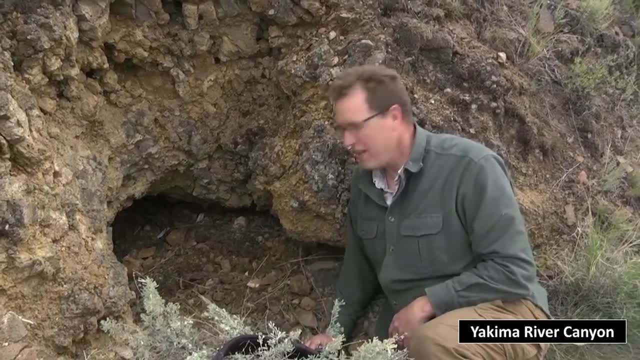 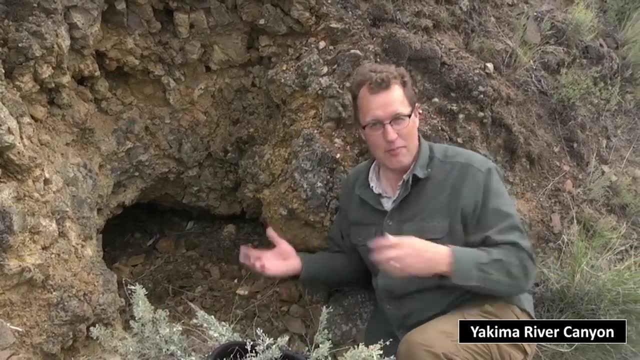 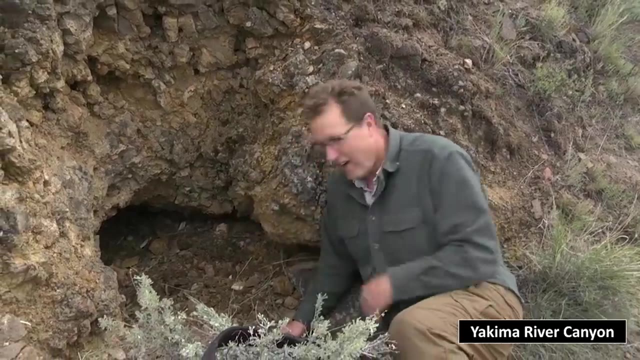 for 15.5 million years, until probably the 1930s, when guys came up here and put incredible effort into pulling a heavy petrified wood log out of the hill and skidded it down to the river. The hole is all that's left. 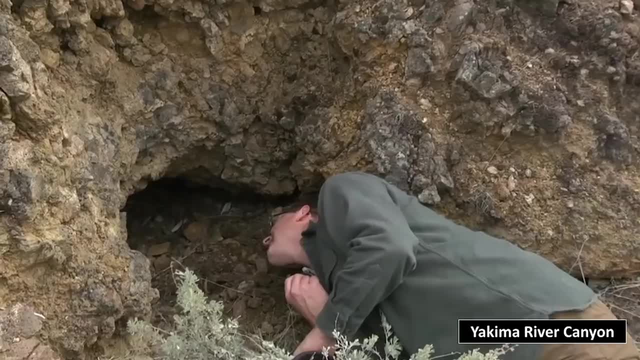 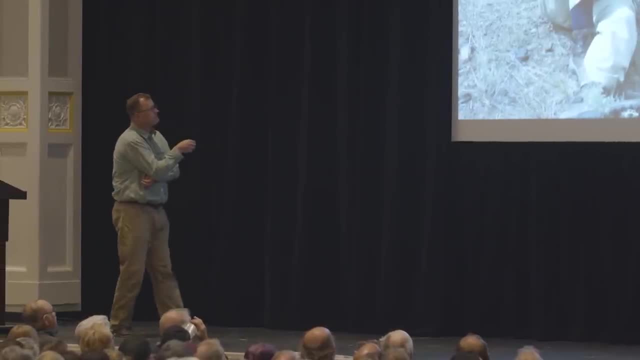 There is some petrified wood. you can see way back in there. Oh my God, You've actually got to take a look at this. You can see a part of the log. I didn't know that. That's cool. You can see why we didn't use it. 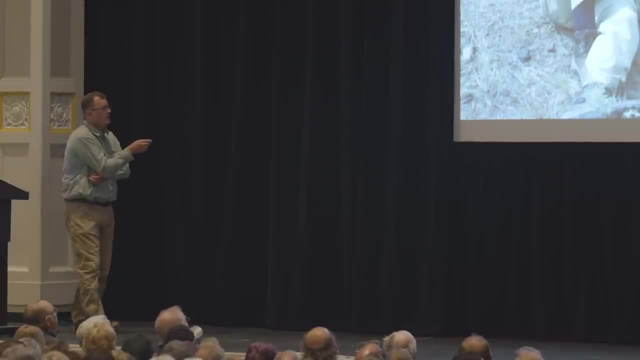 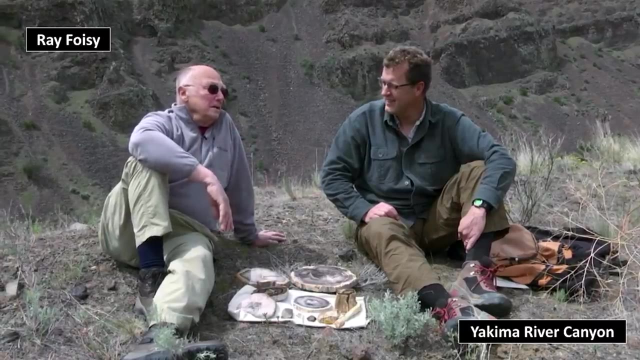 There's a gentleman with us tonight from Yakima named Ray Foisey, And Ray has been a collector for a long time. Yeah, He was going to show me the petrified wood if I'd show him fossils. So we came up. 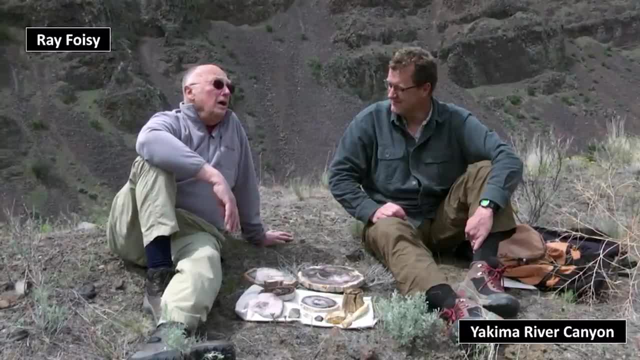 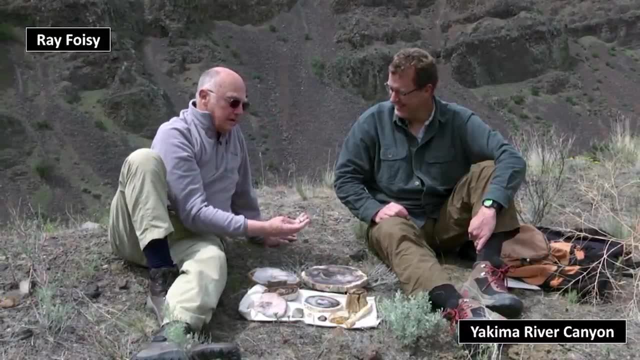 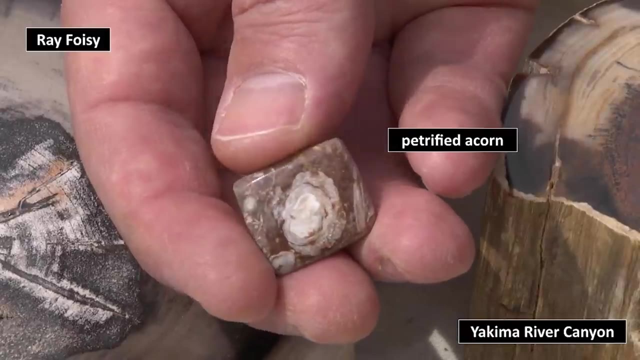 to look at the wood and I happened to look down and right alongside of me was a petrified agateite acorn, An acorn from 15 million years ago. Yes, Come up to the stage after the lecture tonight if you want to chat with Ray. 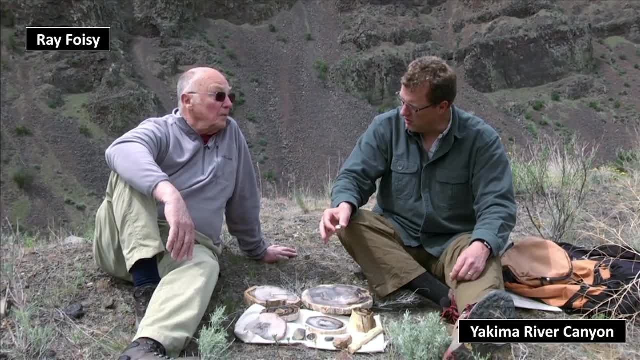 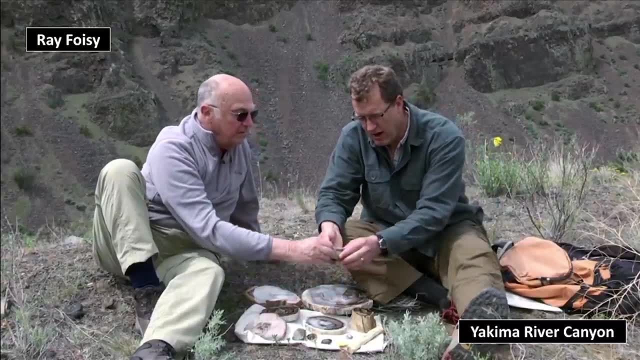 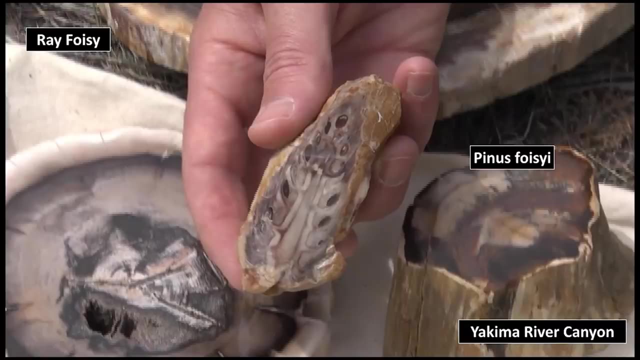 about these things, So it's more than acorns, though. Oh yeah, What else did you find in those piles? One of the most beautiful is the pine cone That happens to be called Pinus foisei, Meaning that it was. 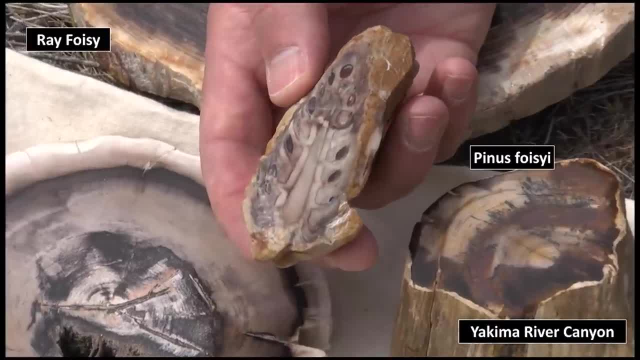 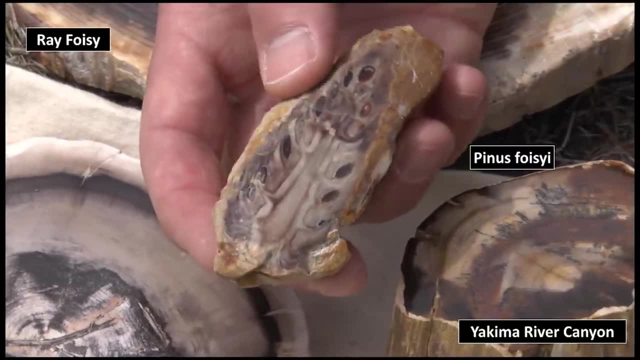 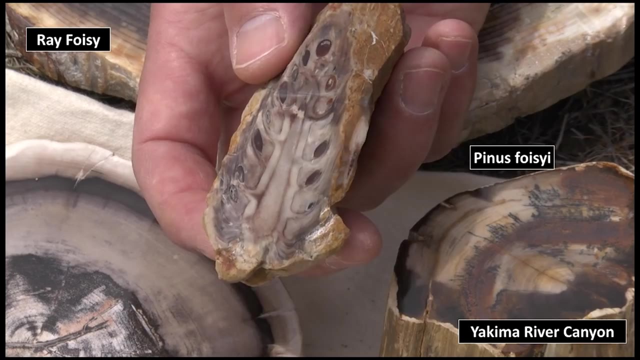 This is all from 16 million years ago, during the time of the Ginkgo flow, and a little bit older in this case. Oh my heavens, How does that even work? Get those seeds in there like that? It's like somebody painted that on. 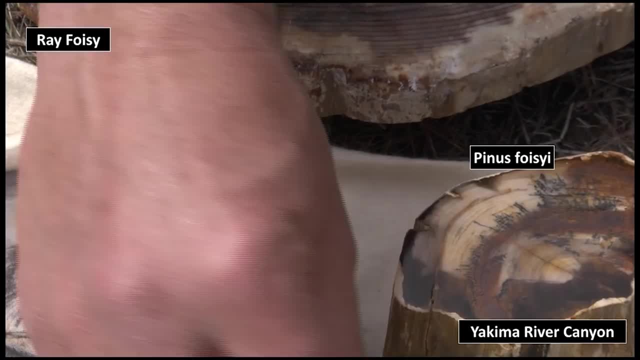 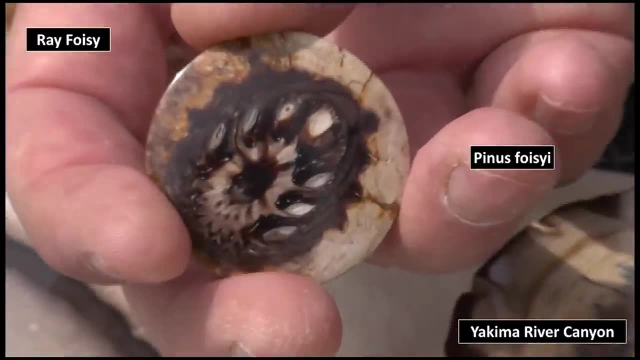 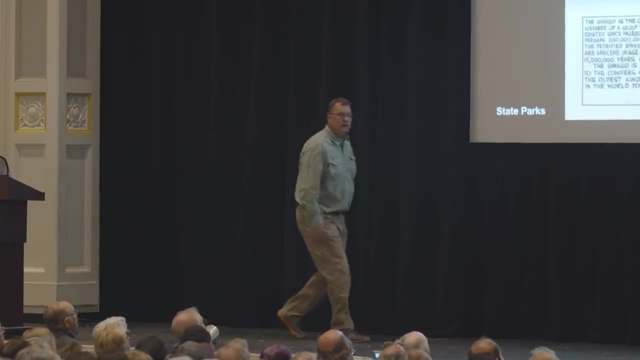 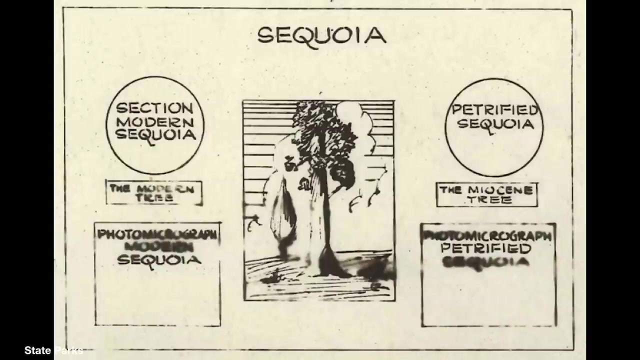 Next one, Maybe the cross section of the cone Pinus foisei. All right, So the person who did most of this work originally to realize the incredible variety of wood. By the way, how do they know what kinds of trees they were? 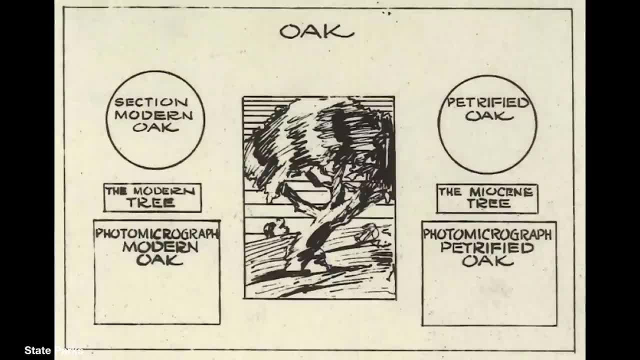 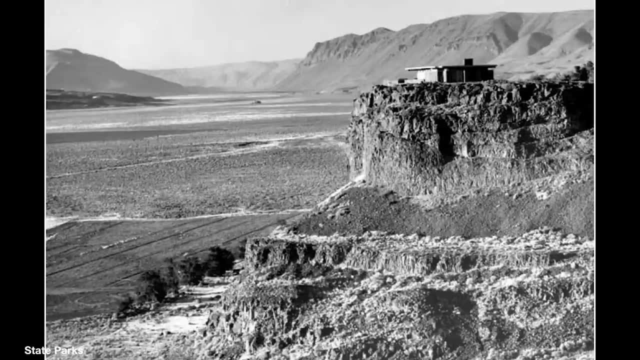 if they're just a bunch of petrified stumps. Is there a way to figure that out? That's coming, And also some details on George Beck. So this is what Vantage looked like back in the 1930s, when George Beck discovered. 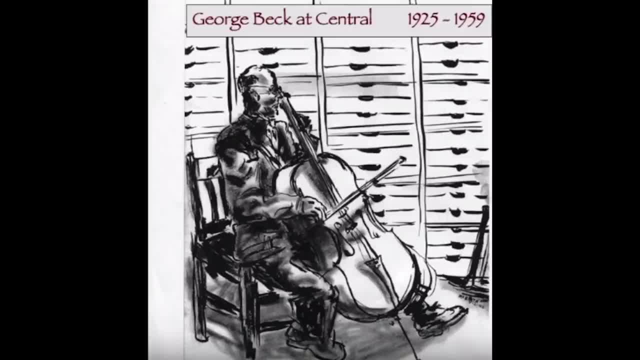 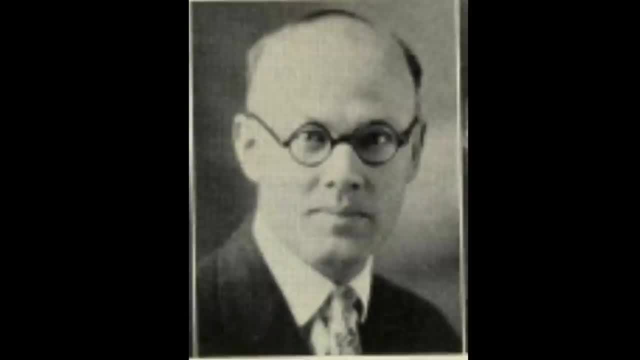 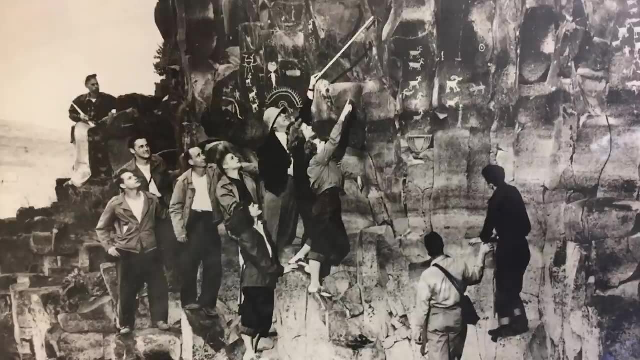 the petrified forest. And finally, we're talking about George himself, A music professor at Central and a geology professor at Central. 1920s George Beck, 1930s and 40s George Beck taking students to the petroglyphs at Vantage. 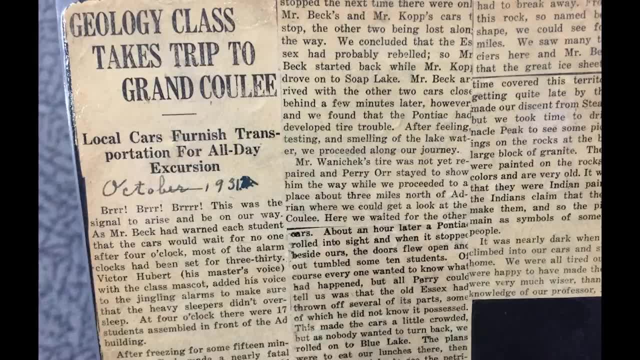 before the Wanapum Dam was constructed. George Beck taking students on field trips in private cars in October of 1931 up to Grand Coulee, before the Grand Coulee Dam was built. yet Amazing stuff that's been put together recently with historical information. 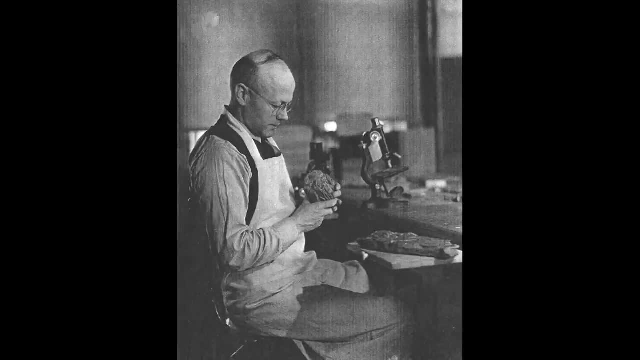 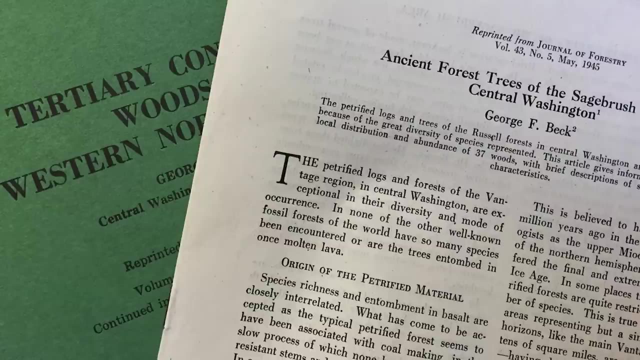 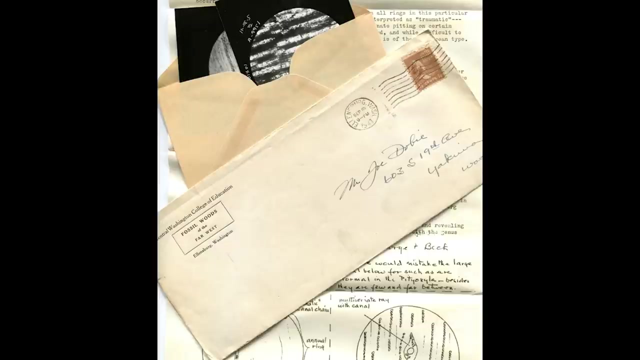 from the archives at Central and some other sources I'm about to tell you about. So George Beck is worth our attention tonight with all of his publications of these logs, as well as his rich history with Ellensburg and Yakima. He was also doing a lot of public outreach. 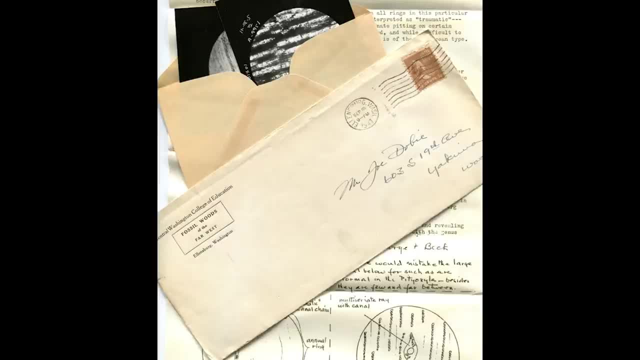 He had a club called the Fossil Woods of the Far West. He's actually got a little return envelope with that letterhead on it And he would send out newsletters and photographs through his microscopes and communicating to people who were really into this petrified wood business. 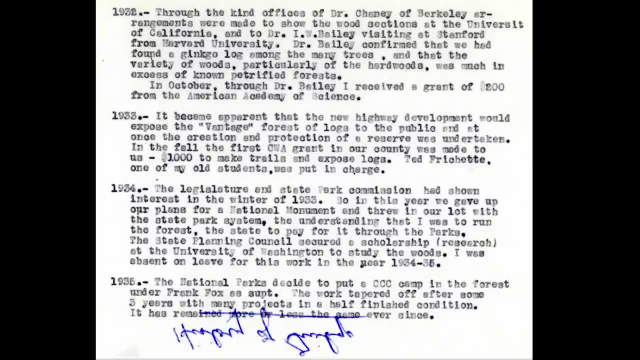 I won't overwhelm you with this, but I've got my hands on some original documents when they started to put the Ginkgo Park together, and I'll point out a couple of quick things: 1933, they were going to build the new highway. 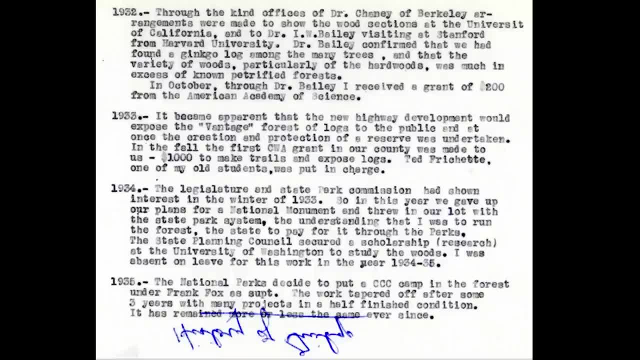 that's the old Vantage Highway to expose the Vantage Forest of logs to the public: 1934, the legislature and state park commission had shown interest to put this into a park status, but in that year Beck gave up on the plans to become a national monument. 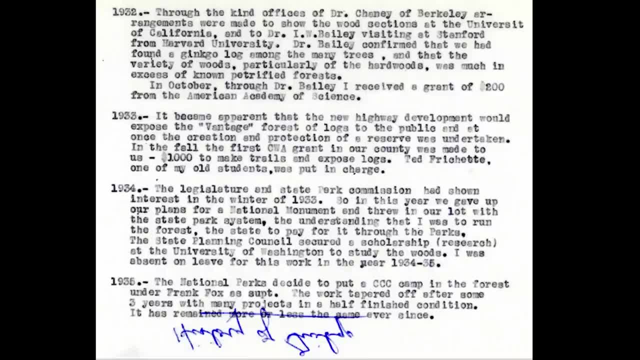 That was the original hope: to have a Ginkgo national monument. have it be part of the national park service and not the state park service. And in 1935, the park service decided to put a CCC camp in the forest under Frank Fox as supervisor. 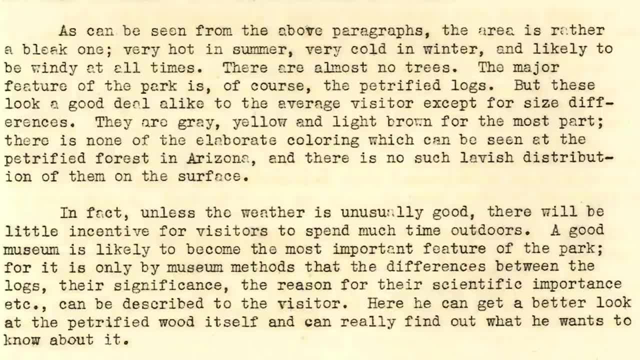 So work began to build, during the depths of the depression, the museums at Ginkgo Park. I got a kick out of that because Beck is saying: look, this area is rather bleak, very hot in the summer. We're talking about Vantage now. 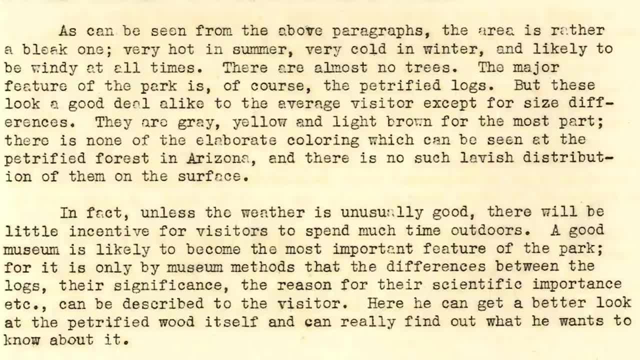 Very cold in the winter, likely to be windy at all times. There's almost no trees. The major feature of the park is, of course, the petrified logs, but these all look pretty much alike to the average visitor, Unless the weather is unusually good. 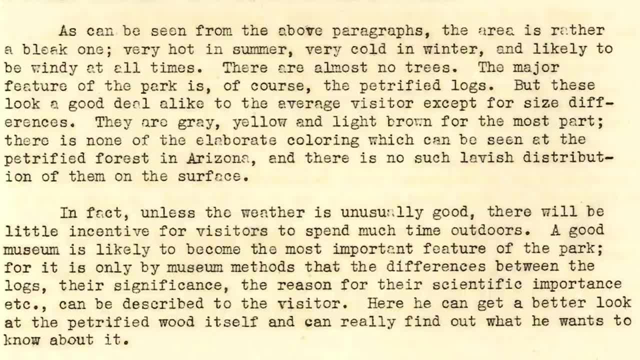 there will be little incentive for visitors to spend much time outdoors. A good museum is likely to become the most important feature of the park, And it's the museum itself that's going to help educate the significance of the logs. Yeah, it's bleak man. 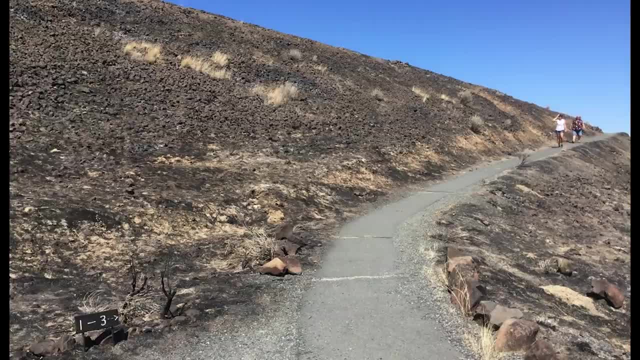 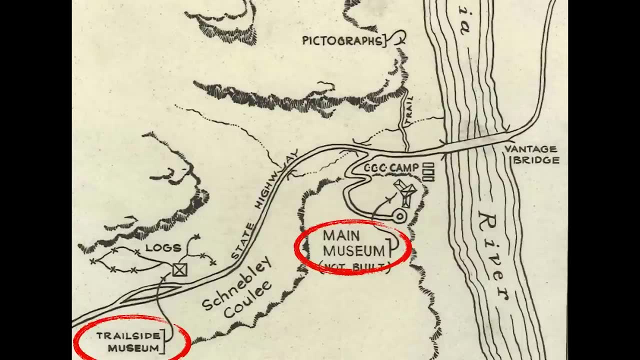 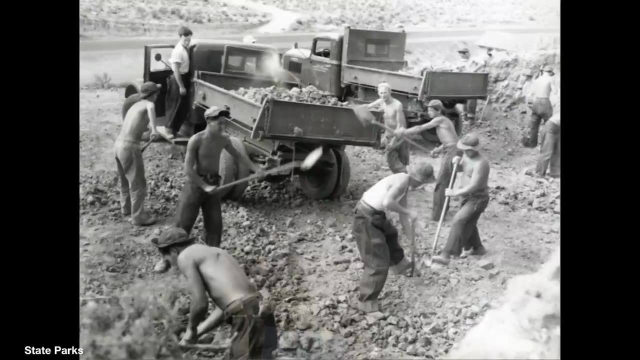 This is last summer after the big fire that went through, But even without fire it's not the most hospitable of conditions most times of the year. The main museum, the Trailside Museum, and the CCC boys make a back-breaking work to put those structures together. 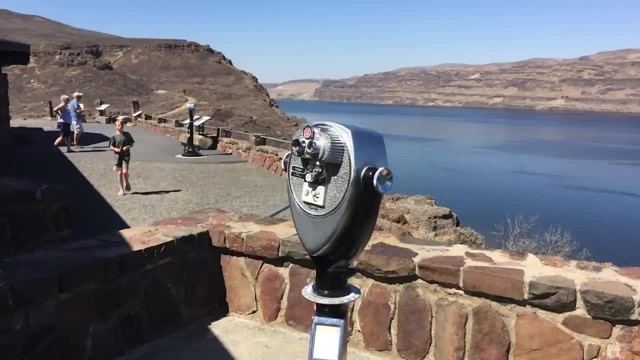 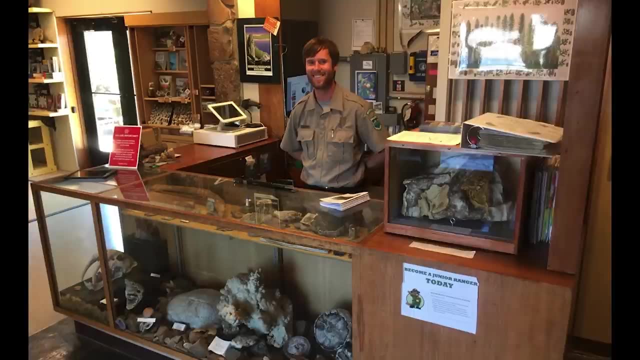 The museum is still there from those days in the 1930s and it's heavily visited by travelers across the state. And there's still a park ranger there who's chatting about all these logs and doing all this material. Some of the exhibits are probably 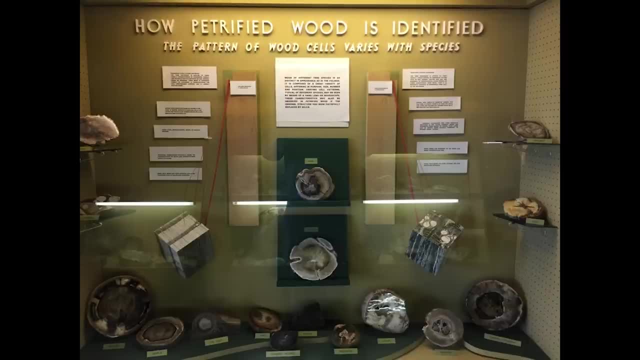 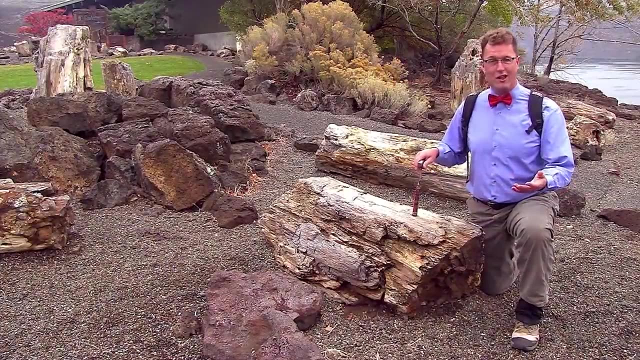 from the 30s, I must say. That's maybe not right to say, but they could use a little dusting off on occasion. Oh good Lord, I am at Ginkgo State Park. Got petrified logs laying on the ground here. 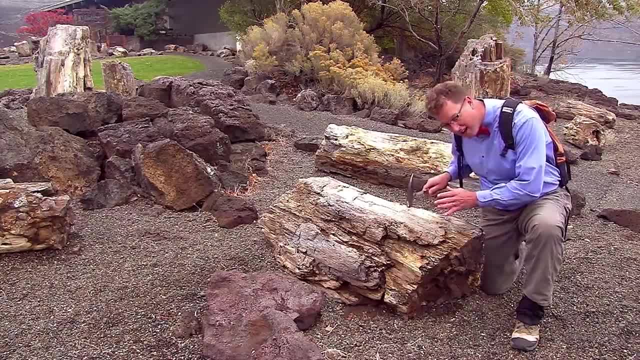 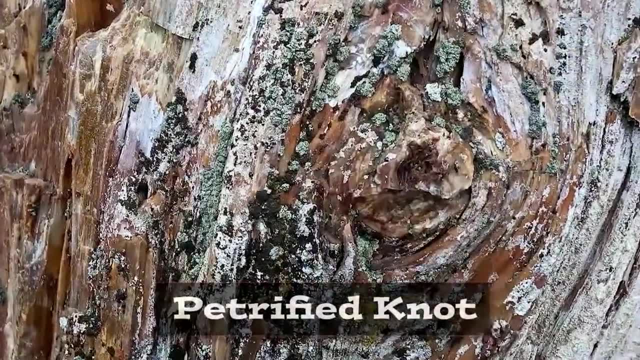 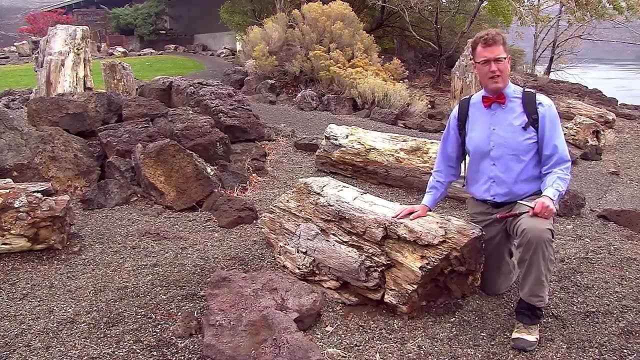 for visitors to enjoy. It's petrified. These are logs made out of stone. They were pulled right out of basalt lava in the hills. Logs right in the lava. Why didn't the logs just burn up from the heat of the lava? 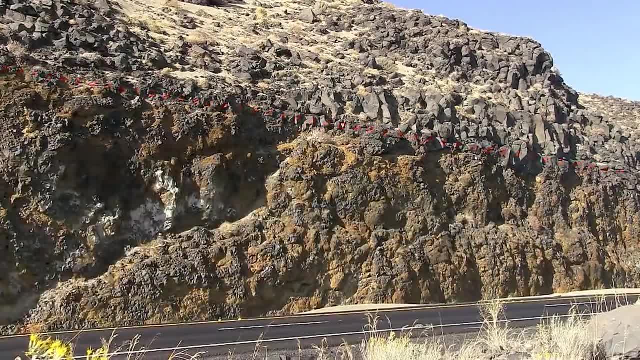 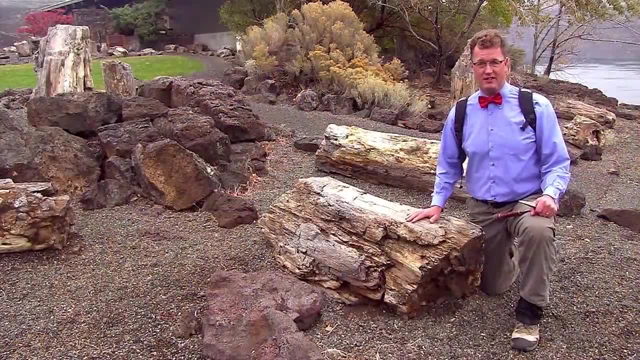 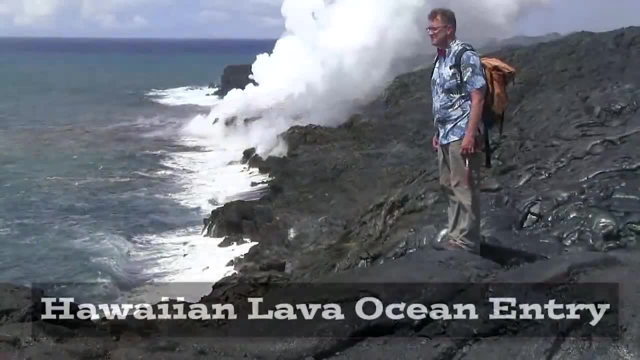 They survived because there was water present. The logs were pulled out of the pillow zone at the base of a lava flow, which tells us that water dominated this landscape. The lake water protected the logs from the heat of the lava, And there was so much lava. 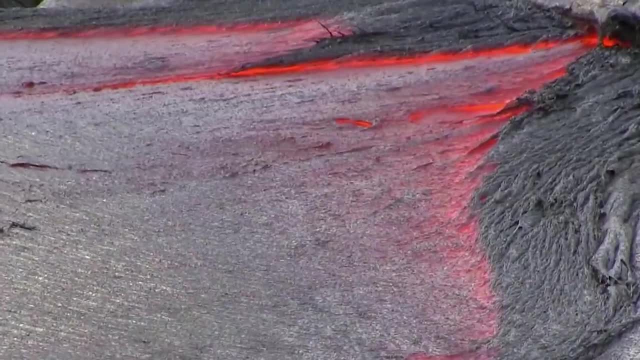 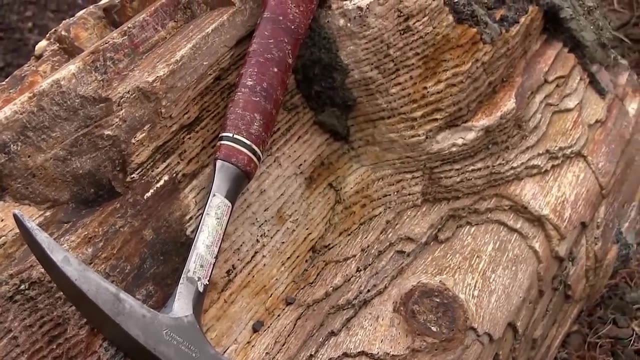 that we sealed off those logs from the atmosphere so we didn't rot the logs with oxygen. We had the right ingredients then for petrification: A lot of water, a lot of heat and minerals. Okay, we got it. If we go to the Trailside Museum, 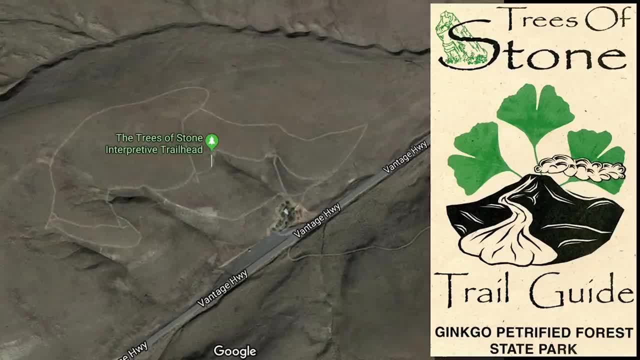 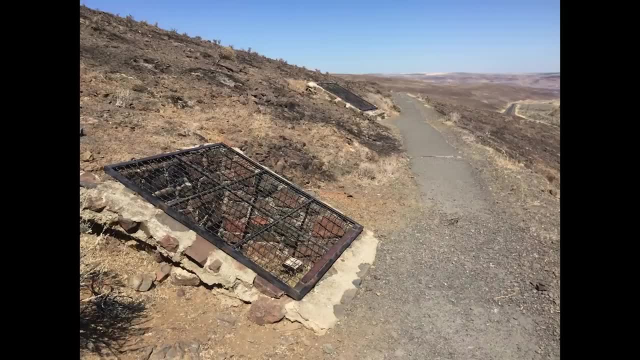 the grand opening back in the 30s and the early 40s and you can go there, You can take these trails. but I understand you got to protect the logs so they don't get pilfered. but maybe we can do a little better than this. 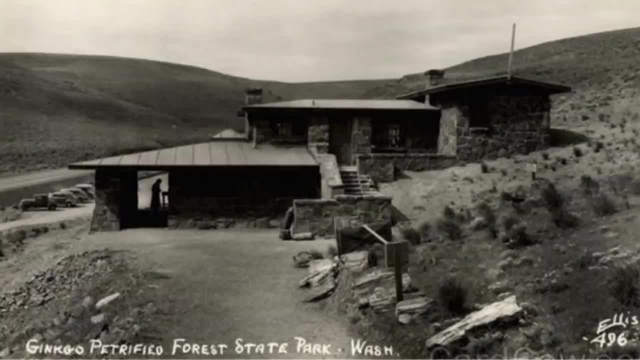 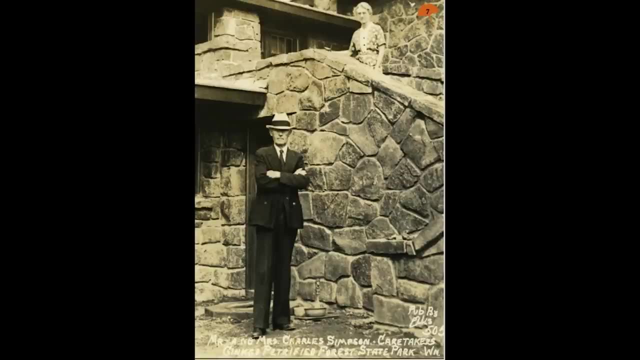 This is kind of a tough sell for some. The caretaker's cabin right next to the museum and this is the place that's going to have the new exhibits. For the first time in decades, they're going to have those new exhibits I've been sharing with you. 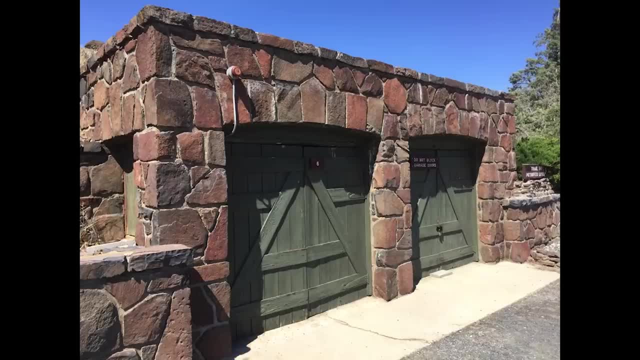 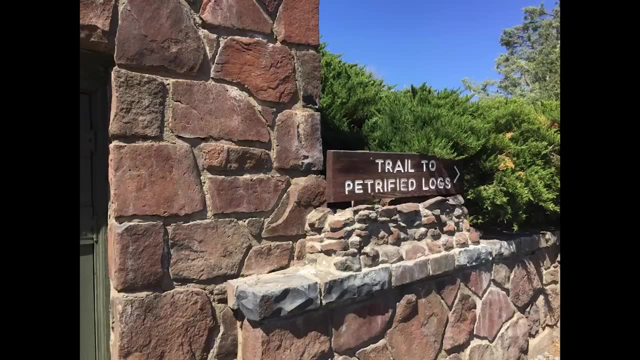 in the Trailside Museum which has been boarded up for years. Looking forward to that Right here, Looking forward to that in the next month or two Hopefully. Trail to the Petrified Logs And again these exhibits by the artwork to try to reconstruct those conditions in Vantage. 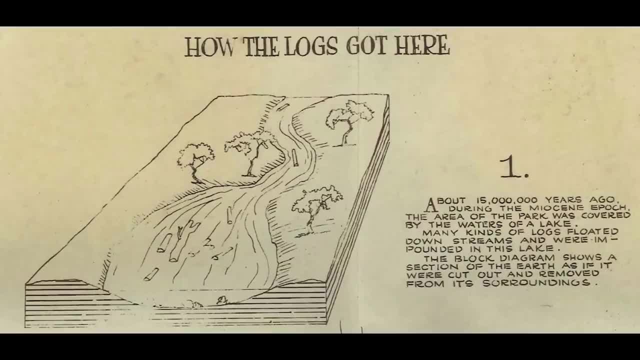 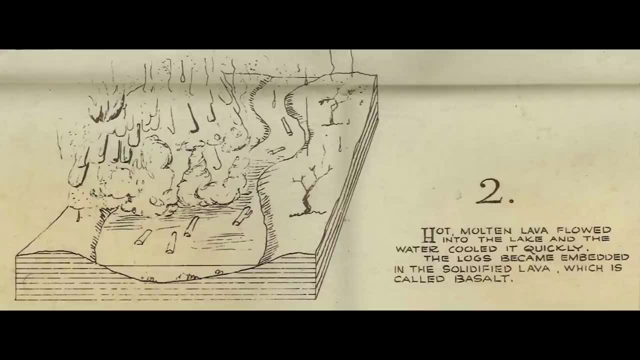 which is very difficult to try to figure out exactly what it looked like when the lavas came in. We're in the homestretch now. Beck is talking about the Okanagan being the source of the logs and having the lavas come in after those logs come down from the Okanagan. 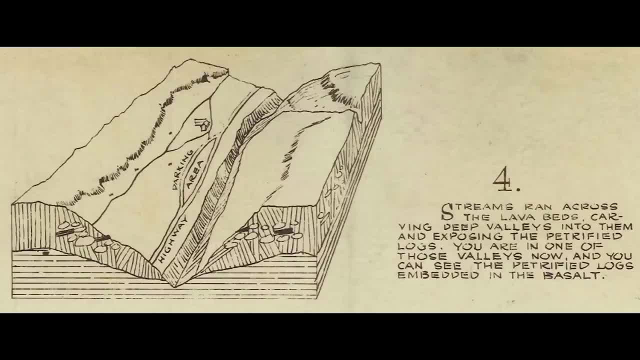 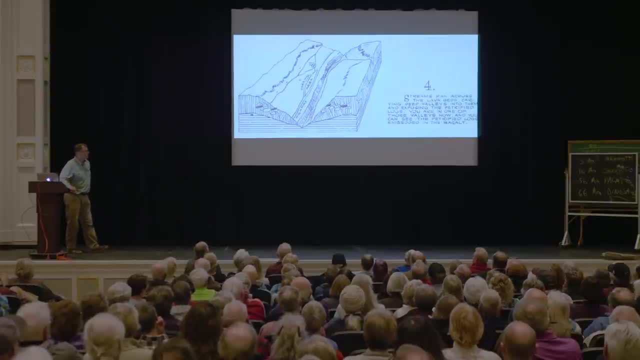 and come down to Columbia. By the way, no talk of the Ice Age. This is in the 1930s. This is before it's accepted that we had Ice Age floods coming from Montana. And this is Beck talking about these trees that have to have come from different elevations. 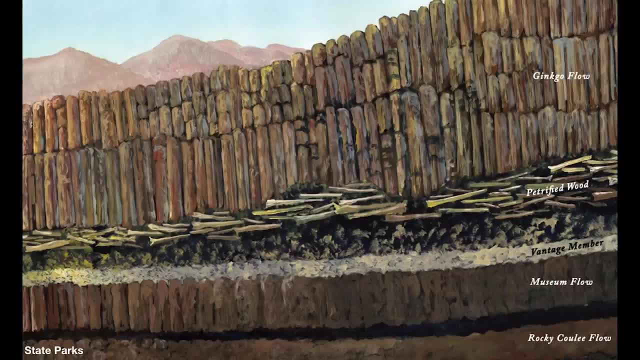 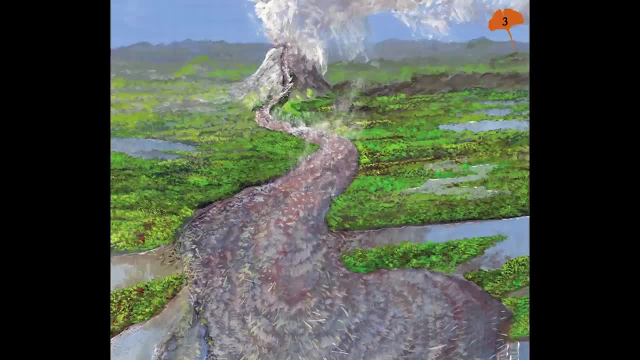 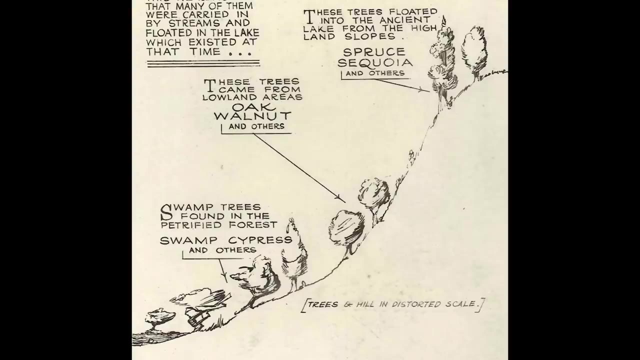 and that's why he was promoting the Okanagan as a source. We know about those logs and how varied they are- New ideas involving lahars. Is this another way to bring all these logs into Lake Vantage? Can we do the same thing? 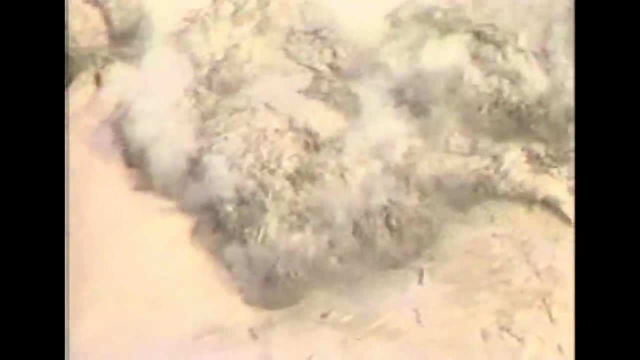 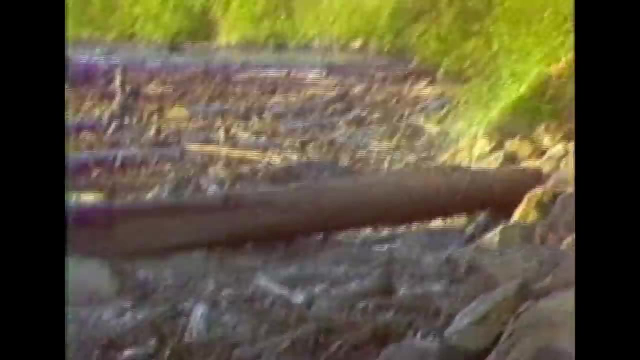 and collect logs from different elevations. Here's some footage of an actual volcanic mud flow. I think it might be actually St Helens in 1980 in the Toodle River. And here we go. This looks promising, But it's difficult to pinpoint for sure. 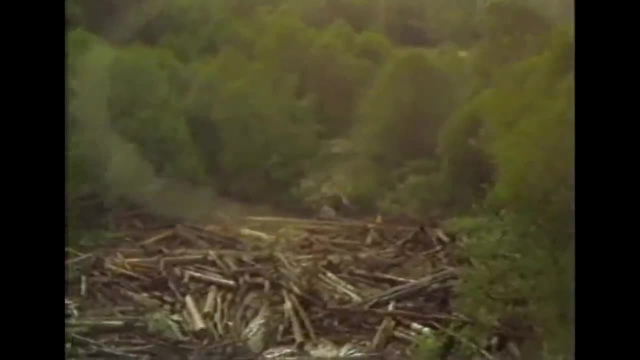 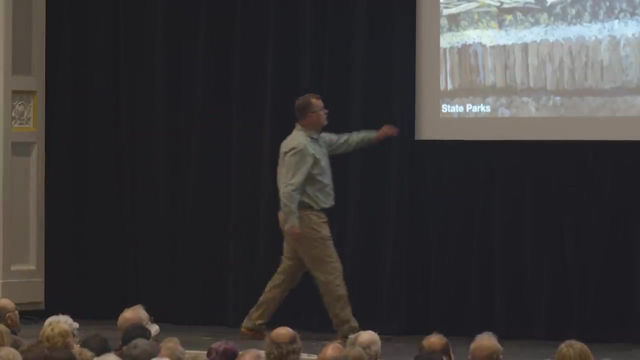 that is the story with the logs at Ginkgo. There are no lahar deposits mixed in with the logs And that's a fatal problem with this story, Even if the Vantage member is a lahar story. why aren't there logs? 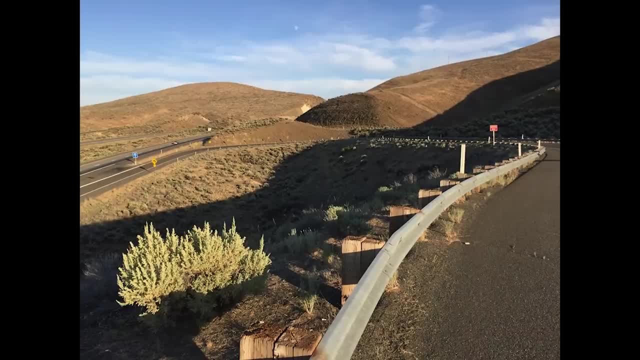 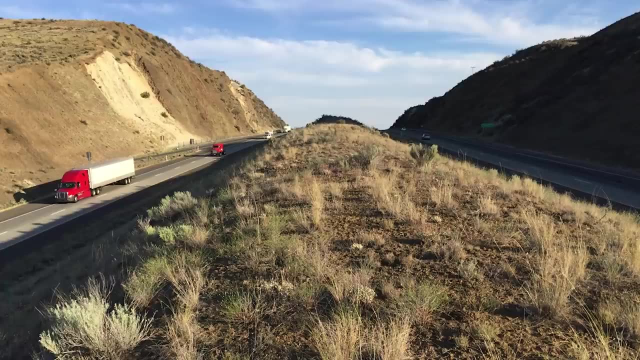 in the Vantage sediment itself. The Vantage sediment is not only at Ginkgo, it's just north- excuse me, just south of Ellensburg, up on Menashtash Ridge through Vanderbilt Gap. Last summer I picked just the right night. 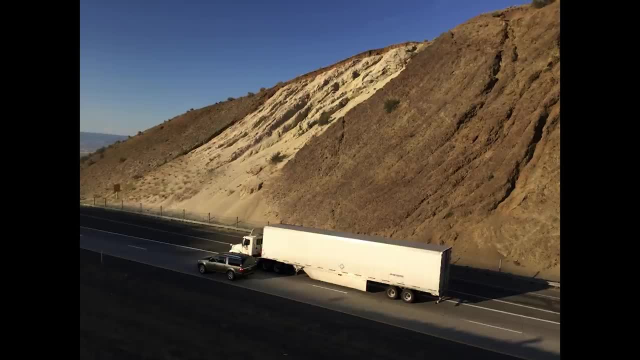 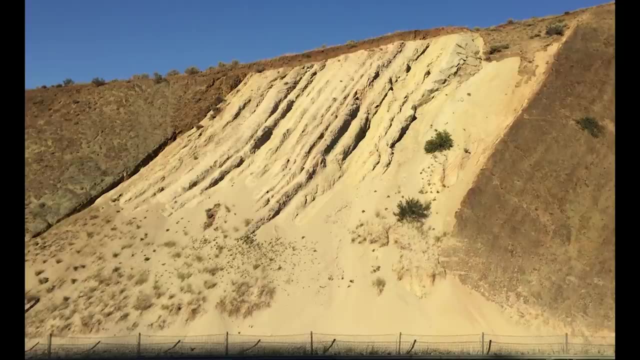 to get good light. You know that spot. Can you picture this? We're on the east wall, right past the rest areas, at the summit of Menashtash Ridge, And can you see the repetitive little flood-type deposits, The 15 mini layers within the Vantage? 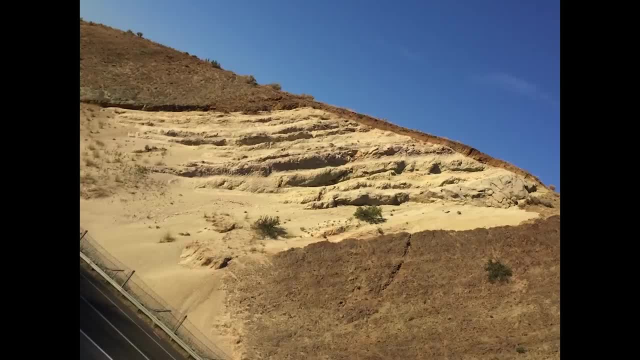 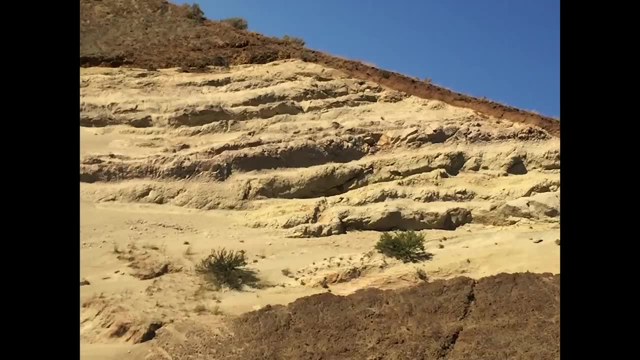 This is the Ginkgo flow on the left and an older flow on the right. If we restore those, at least with my camera, to their original horizontal position, can we look in detail at those layers and convince ourselves it's an Okanagan story. 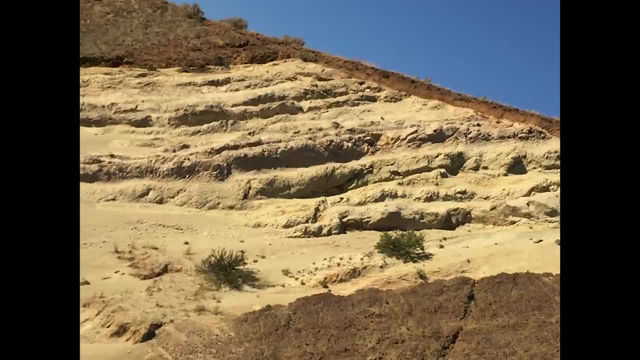 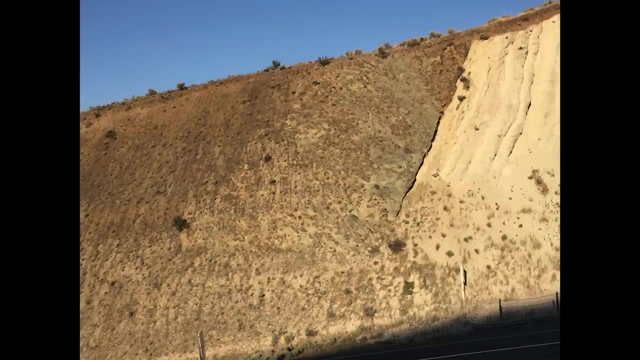 instead of a Cascade story. We cannot with our current understanding, And these layers continue to be looked at. By the way, if you feel like risking it, stop at the rest area on the northbound side of I-82 at Menashtash. 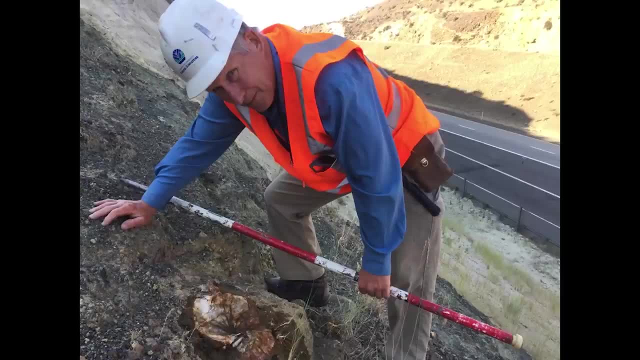 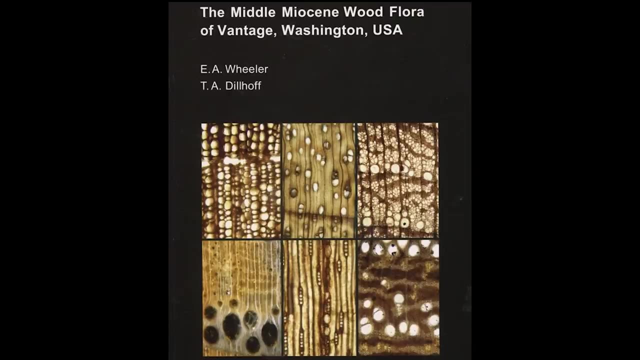 Scramble up this, which is very difficult, And Jack Powell and I did this last summer, And there are some petrified logs up there. Wonderful, Tad Dilhoff has put really the best resource available in my opinion. It's a beautiful, glossy little book. 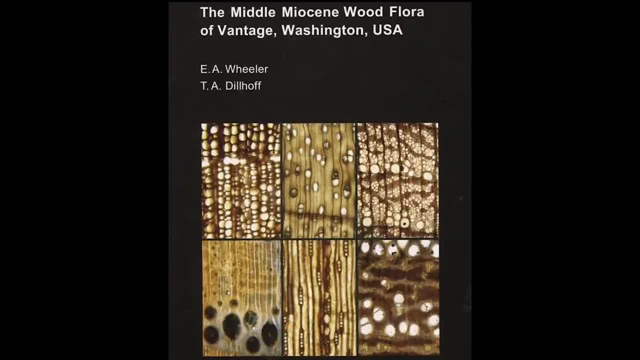 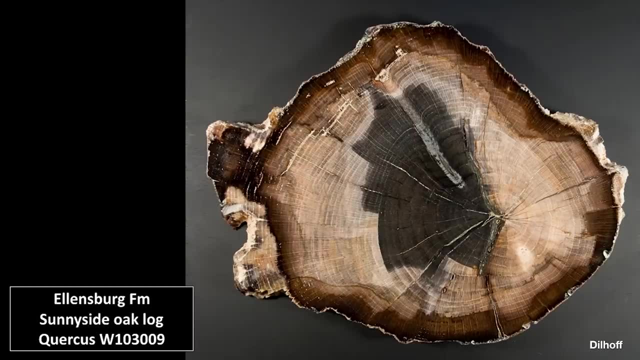 called Middle Miocene Wood Flora of the Vantage Washington, USA. It's a few years old but really well worth your efforts to get it on Amazon perhaps. And Tad has continued to help us identify woods, understand and try to promote. 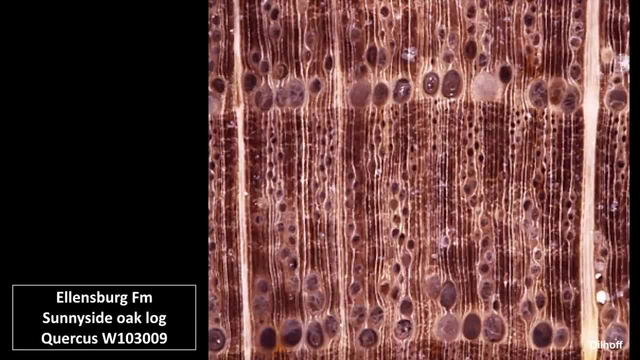 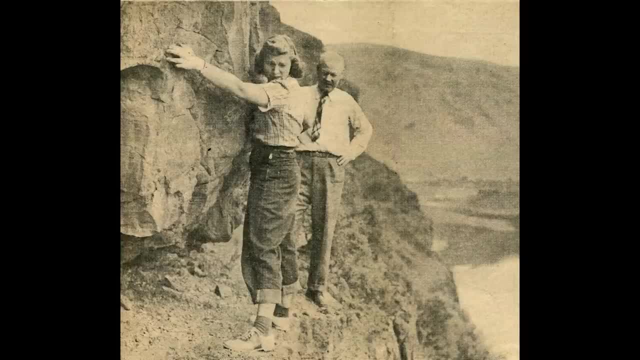 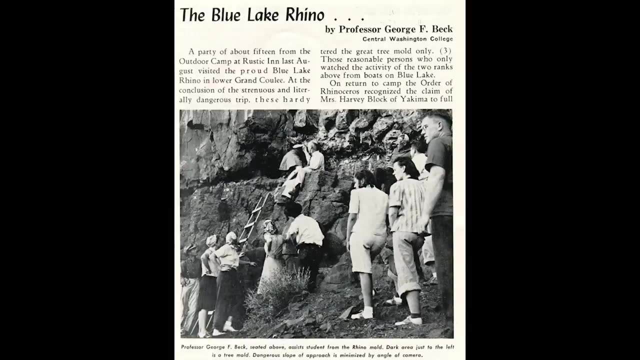 new work with these petrified wood samples to eventually solve the mystery of the source Okanagan Cascades. both or neither. We finish tonight with our friend George Beck and paying particular attention to him up at the Blue Lake Rhino, where he was actually helping to promote. 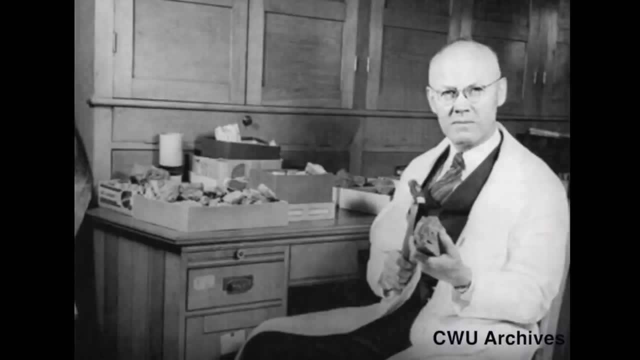 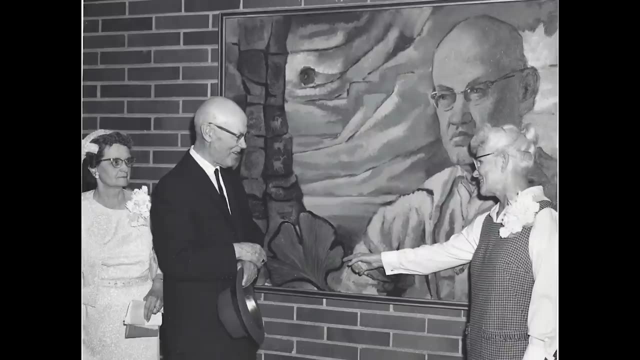 that rhinoceros mold that was found near Dry Falls, Also from this Miocene time, And Beck continued into the 1950s and after his retirement at CWU, was honored with a celebration and artist professor Sarah Spurgeon created this big, colorful mural. 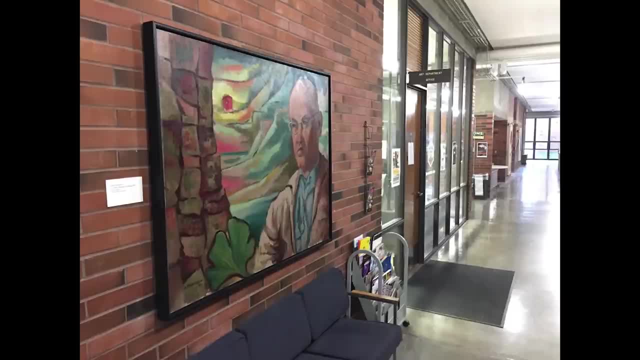 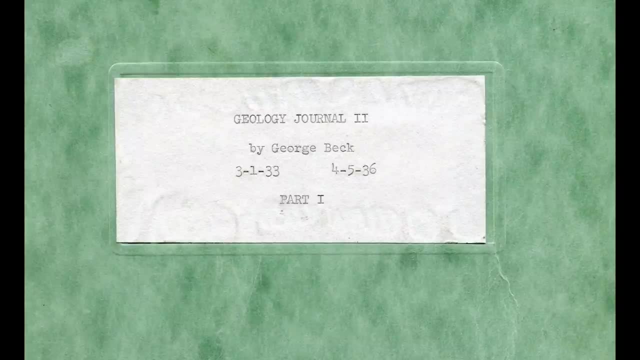 of George and the Ginkgo leaves. and that mural is still in Randall Hall at Central's campus. That's my mother. We're almost done. In my office I've had this photocopied version of George Beck's journal, Not the original. 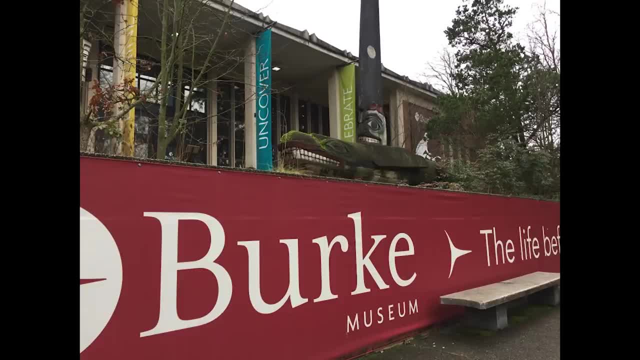 Book one of his journal And it's all I had, And it's all the Burke Museum had. And Tad Dilhoff, this fellow I've mentioned a lot, has really wanted to get the original journals from George Beck. But how was that going to be possible? 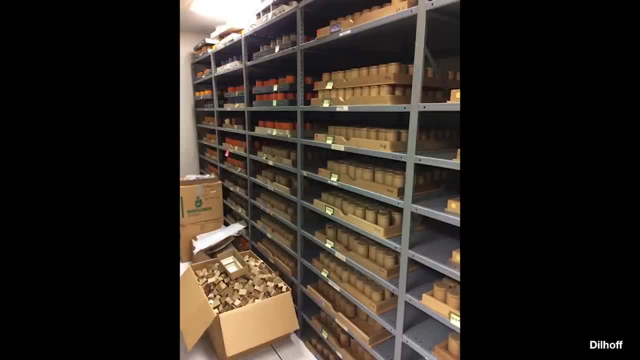 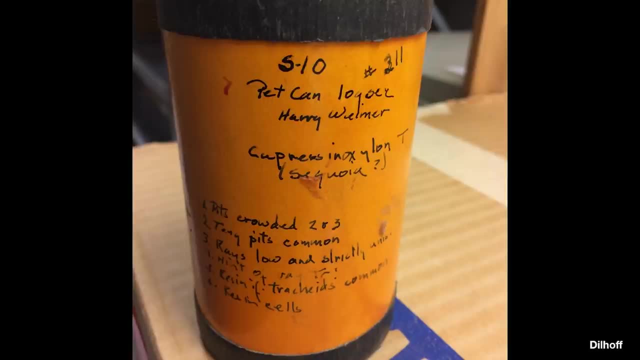 They have all of Beck's materials now at the Burke in Seattle: All his little petrified wood chips, All of his handwritten work. It's in the right place. Those are the folks doing the paleobotany research. And then I got tipped off. 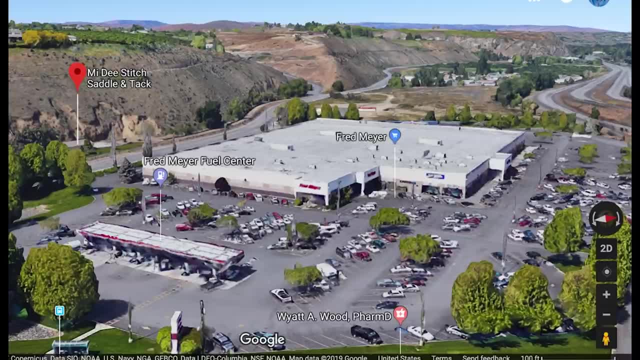 that there's a relative of George Beck still with us in Yakima. You say: go down to 40th Avenue in Yakima. You know where the Fred Meyer is. Yeah Well, right behind Fred Meyer there's a saddle shop. 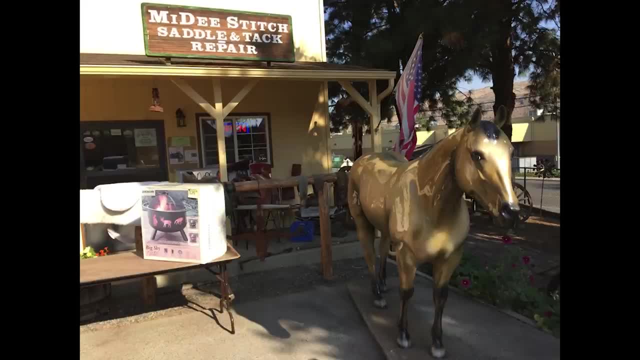 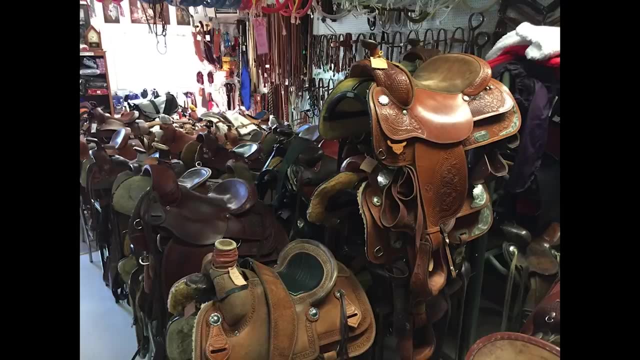 The mighty stitch, saddle and tack repair. So I called ahead of time, explained who I was. The guy said: sure, come down, I'll chat with you. It's George Beck's grandson, And I visited the first time and chatted a little bit. 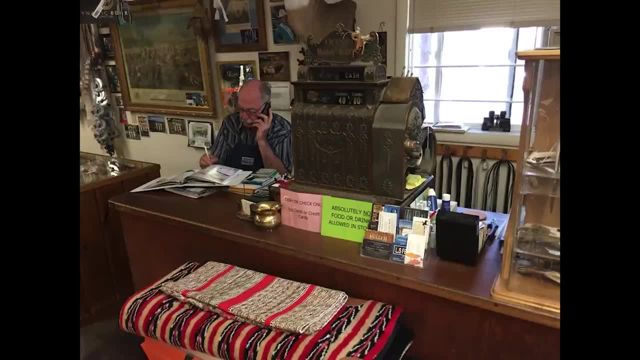 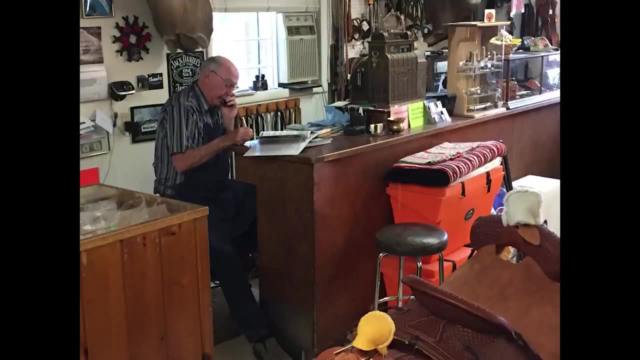 about his grandfather George Beck, And came back the next time and developed a little bit more trust with George. Mitchell is his last name. He's also named George, So George Beck we're talking about tonight, But George Mitchell, the grandson. 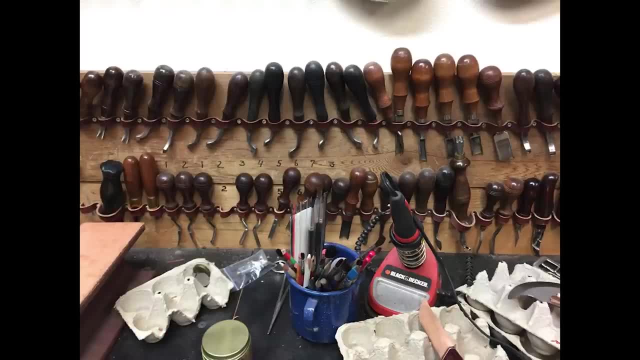 runs this saddle shop And I kept visiting every few weeks And the visits got a little longer and a little longer And before long I got invited back Private work area with the shop And the next visit. well, I got a few things. 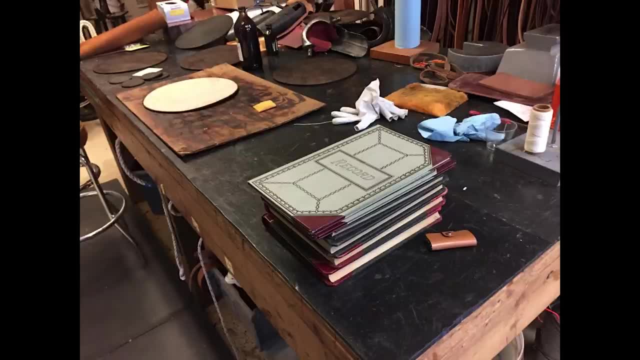 that George had. you know, And I'm the last of the family, Nobody else is really interested in this. Would you like a few of some of the original documents for George And I'm like: yes, that's wonderful. Thank you. 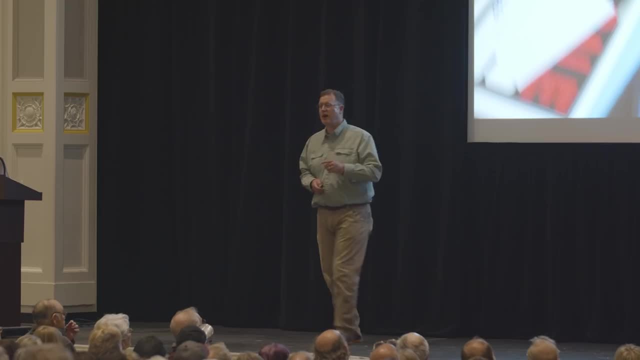 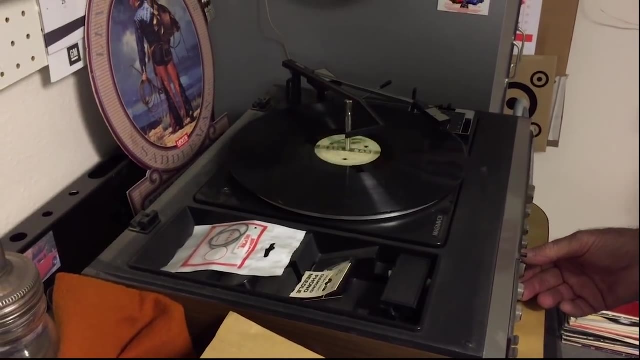 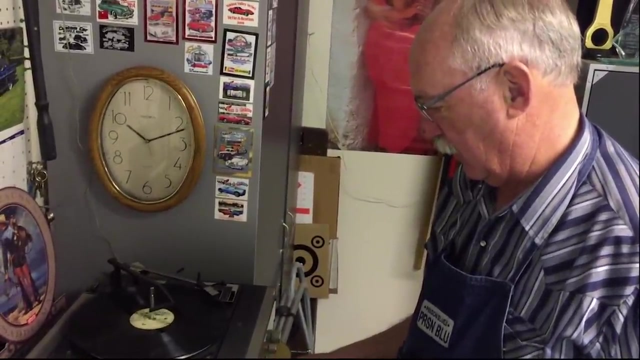 And then I went back again And there was another surprise for me. Tonight we turn our eyes to the future, Injected a world as peace or totally destroyed by the weapons of another war. Now, if our second guest comes to the microphone, George had found some 78 records.